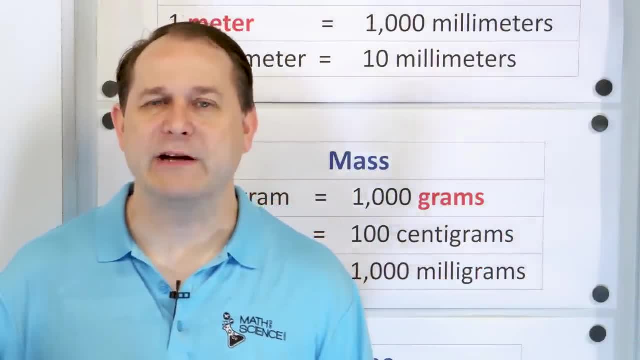 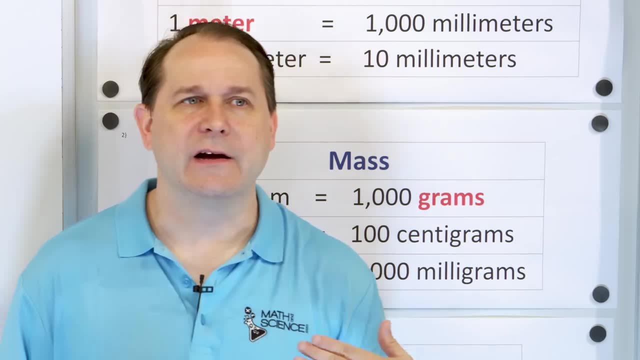 be talking about the US system or the British system of measurement and converting between pounds and ounces and things like that. And when I show you the same table, the numbers will not look nice like this. They'll look weird and just random, And that is one of the main reasons we use. 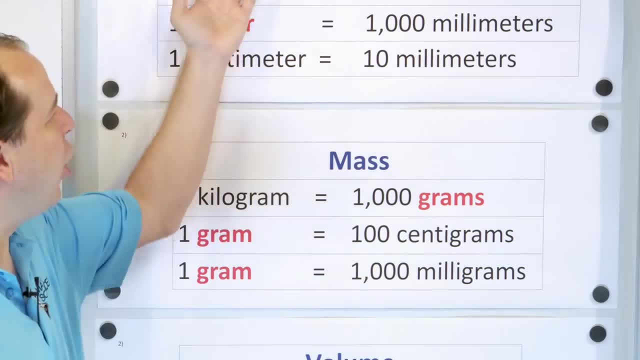 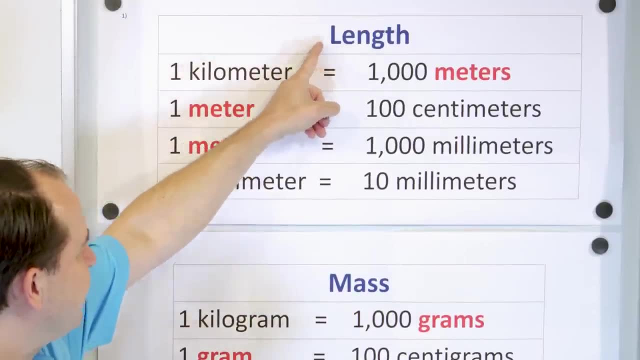 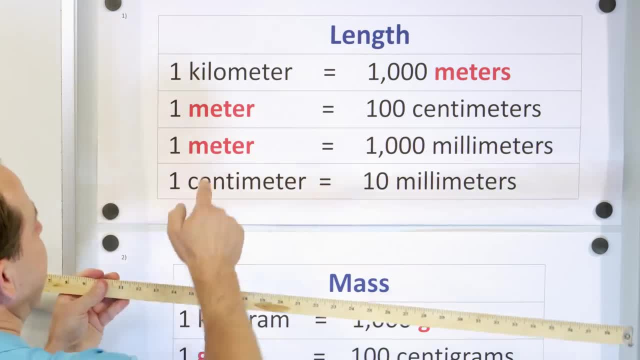 going to go from there. So what is the unit of length? Well, we're going to go from there. So what is the unit of length in the metric system? The basic unit of length- you can see it in red- here is the meter. This is the basic unit of. 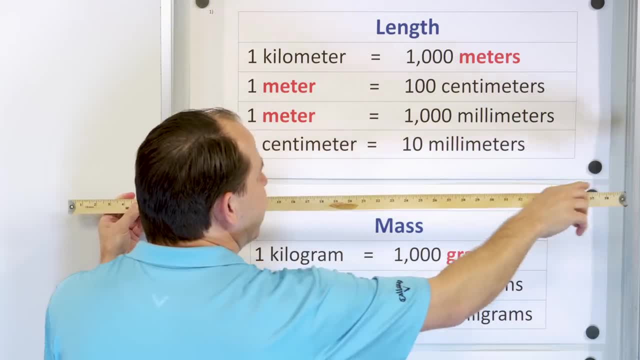 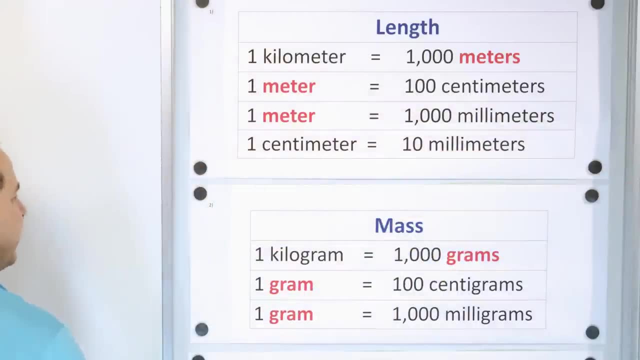 length. We're going to come back to what the unit of length of a meter. you know how we work with it later, But for now just remember the basic unit of length is called the meter. Then we talk about something called mass. The unit of mass in the metric system is called the gram. You see, it is in. 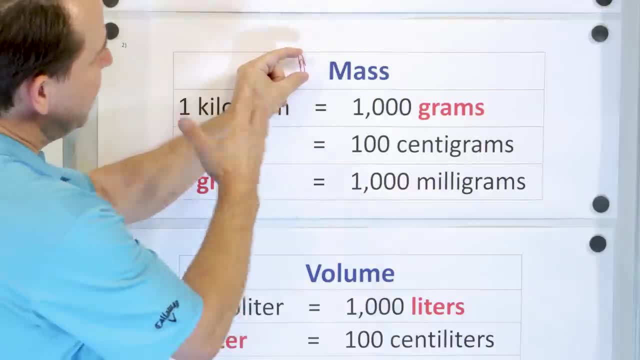 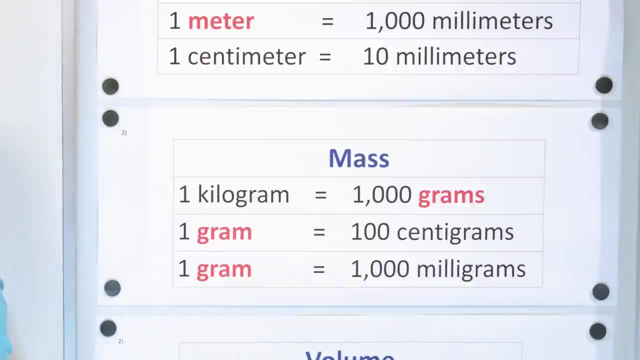 red here The basic unit here we call it the gram. At least in this lesson we're going to call it the gram. The paperclip that I'm holding up is one gram, And the basic unit of one meter is this stick here: 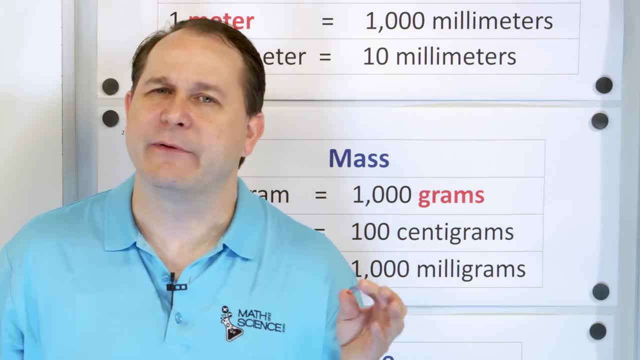 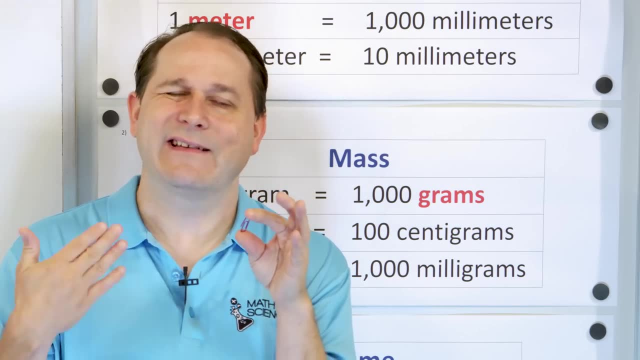 All right. Now, exactly what is mass? Some people think it's the same as weight. It's not really the same as weight. The unit of mass, of grams, is telling you how much material is in here. It's kind of telling you how many atoms and what kind of atom It's. how much mass, how much matter is. 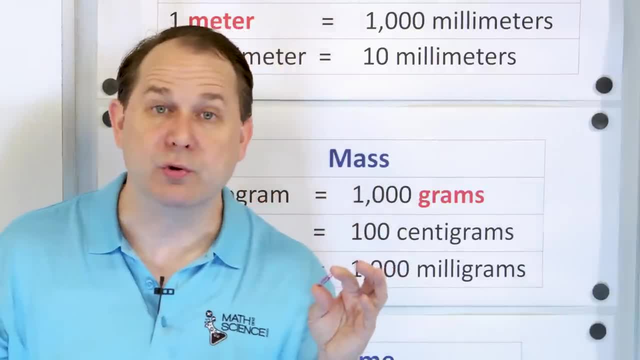 inside of this thing. Now, if I take this paperclip to the moon, it will not weigh as much, but it will still have the same mass. If I take it to Jupiter, it will not weigh as much, but it'll still. 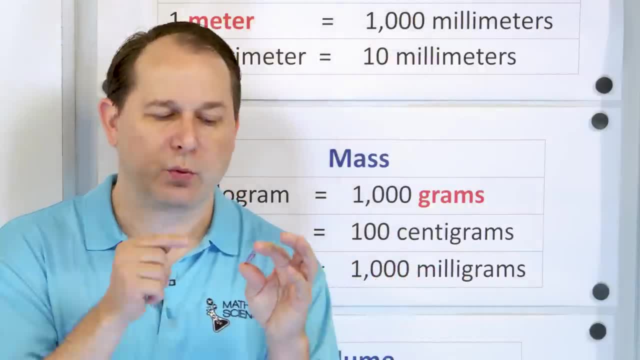 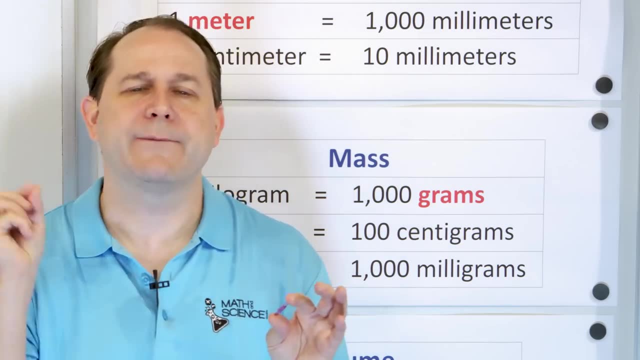 have the same mass. If I take it to Neptune, it will not weigh the same, but it will have the same mass. So the mass of an object never changes. But when you go to different planets with different strength- gravity, the force of gravity- the weight can change, but the mass never changed. The 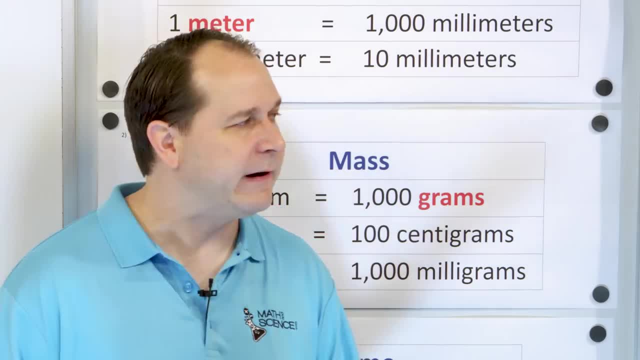 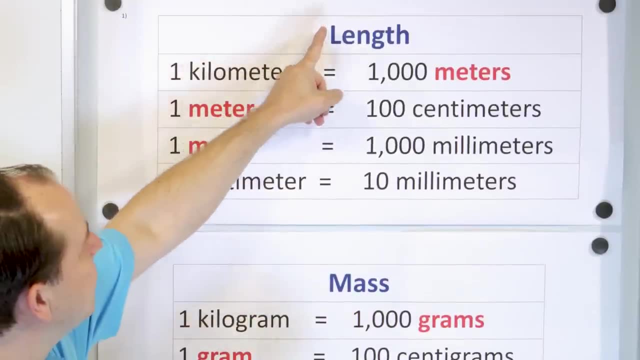 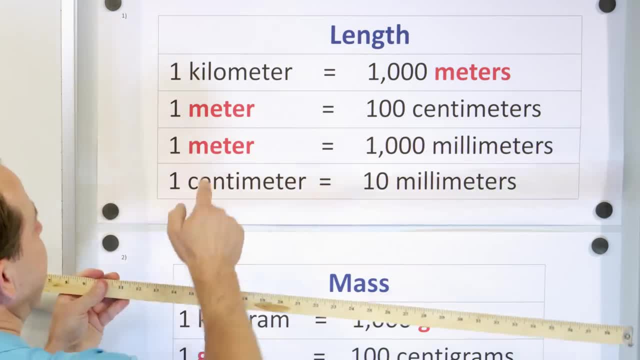 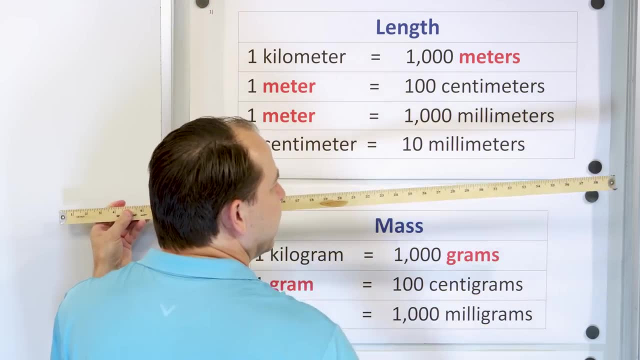 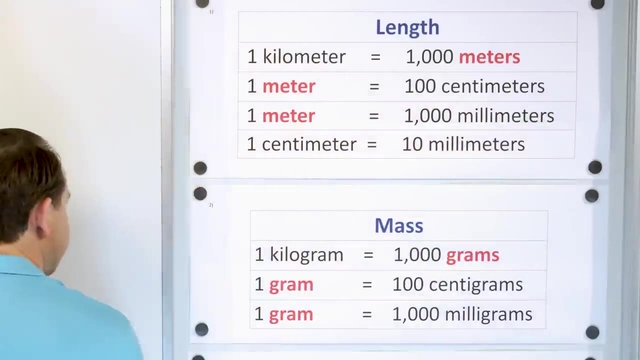 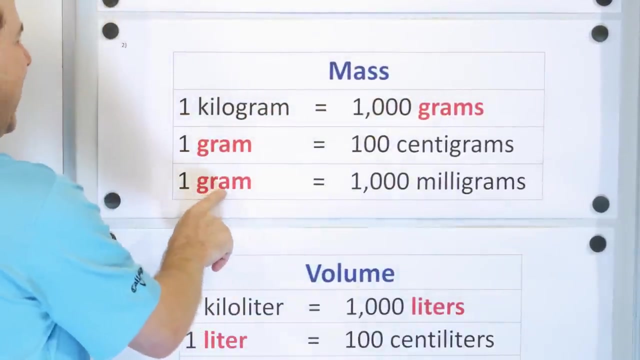 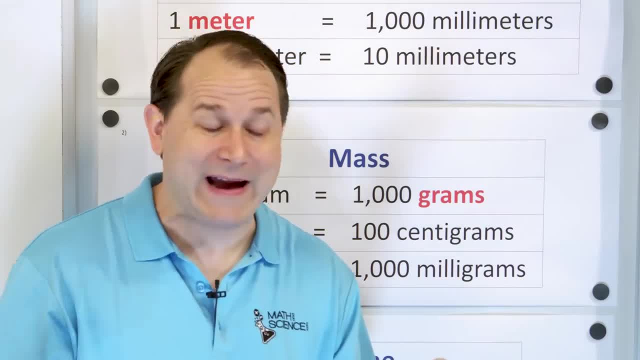 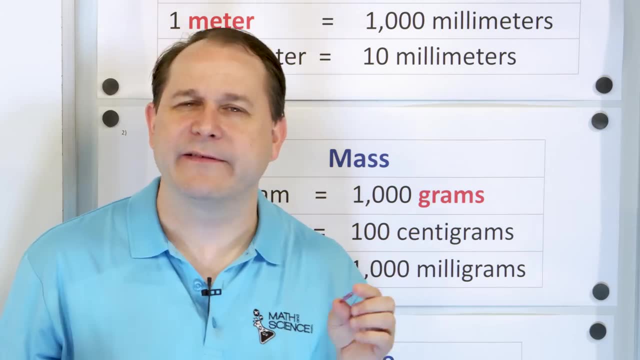 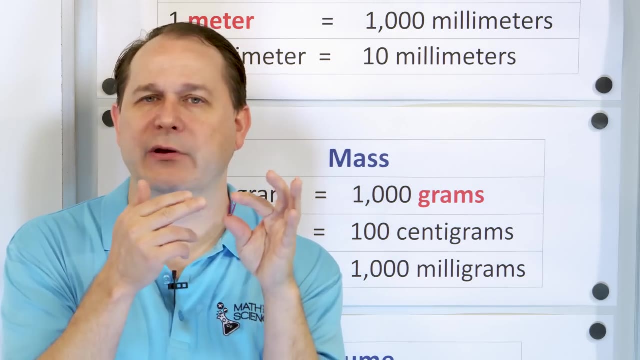 The paperclip that I'm holding up is one gram, and the basic unit of one meter is this stick here. All right. Now, exactly what is mass? Some people think it's the same as weight. It's not really the same as weight. The unit of mass of grams is telling you how much material is in here. It's. 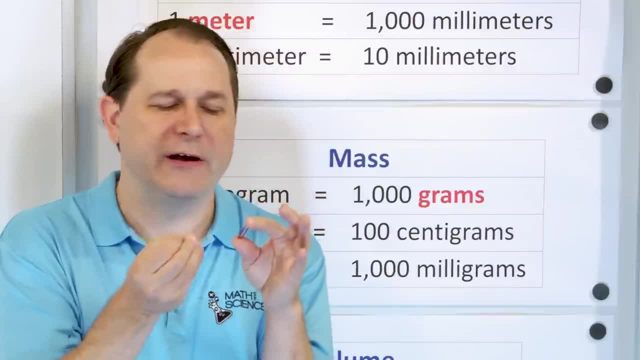 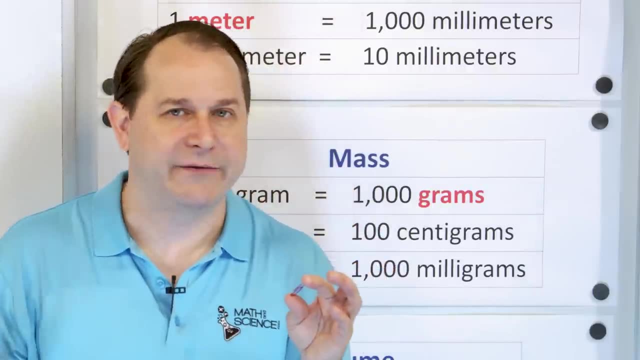 kind of telling you how many atoms and what kind of atom It's, how much mass, how much matter is inside of this thing. Now, if I take this paperclip to the moon, it will not weigh as much, but it will still have the same mass. If I take it to Jupiter, it will not weigh as much. 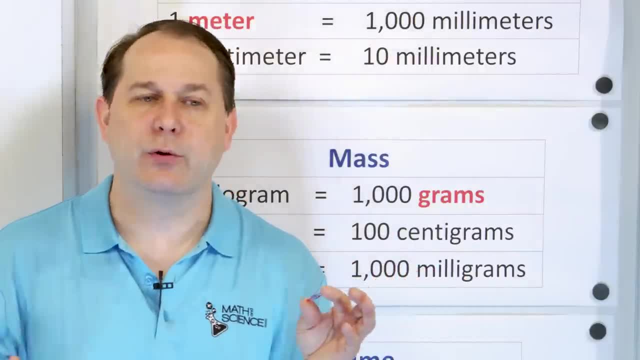 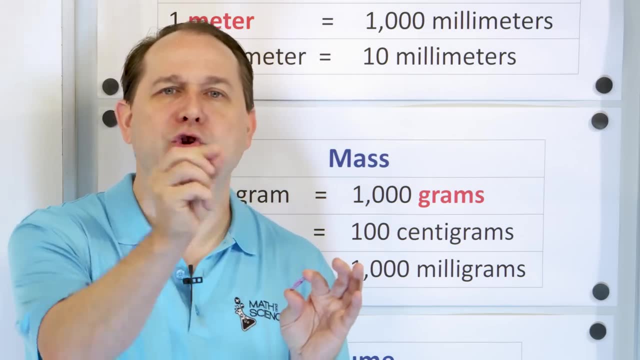 but it'll still have the same mass. If I take it to Neptune, it will not weigh the same, but it will have the same mass. So the mass of an object never changes. But when you go to different planets with different strength, gravity, the force of gravity, the weight can change. But 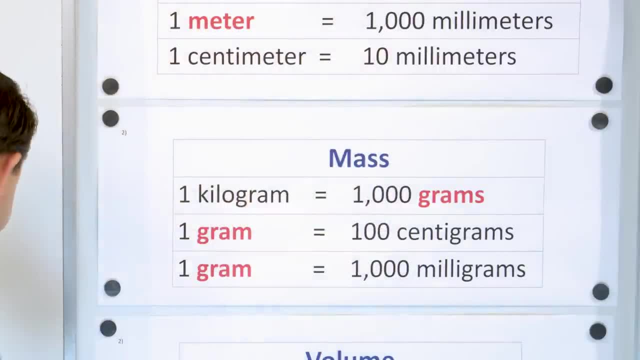 the mass never changes. The basic unit of mass is a gram. And then, finally, we have the unit of volume. Unit of volume. it doesn't talk about how much matter is in there, It talks about how much mass is in there. It talks about how much matter is in there. And then, finally, 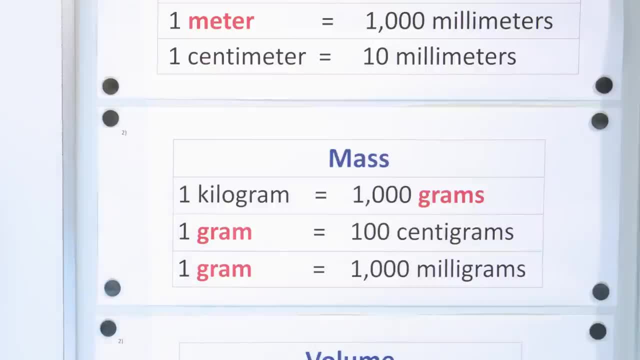 basic unit of mass is a gram. And then, finally, we have the unit of volume. Unit of volume. it doesn't talk about how much matter is in there, It talks about how much matter changes. 84 00 Gruy결. 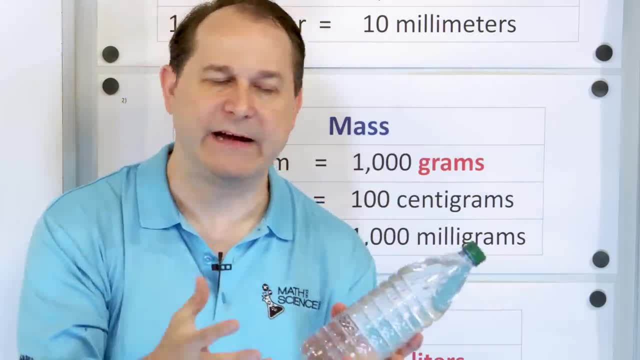 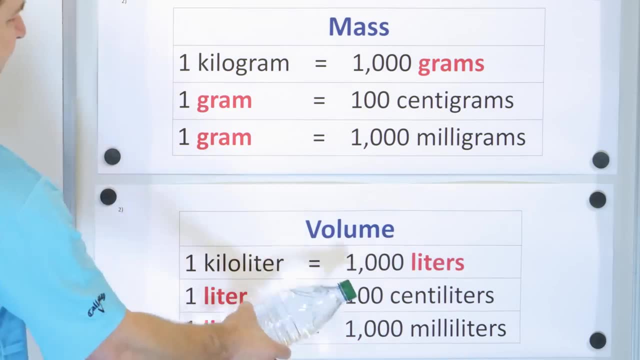 space something occupies. How much space in our world does it take? The unit of volume is the basic unit of volume and the metric system is called the liter, And this right here is one liter here. So if you can kind of imagine drinking something like this, this: 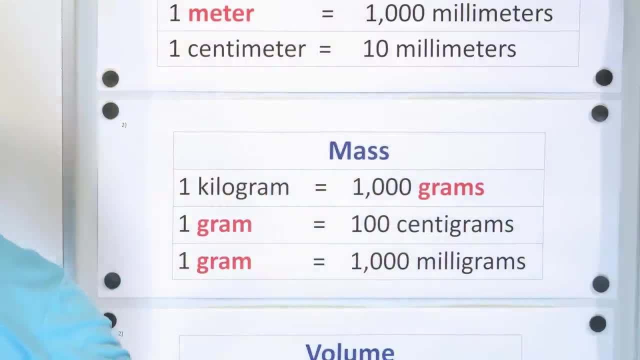 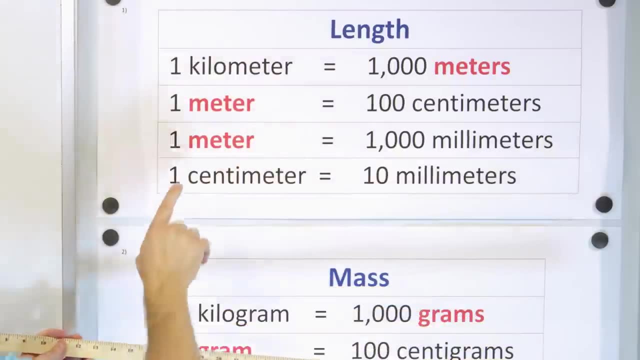 is one liter, All right. So those are the three main units that we're going to be talking about Now. let's go a little more detail here. You see this chart. we have meters, meters, meters. All right, We have to learn a little bit more. You see, we have kilometer, kilo. 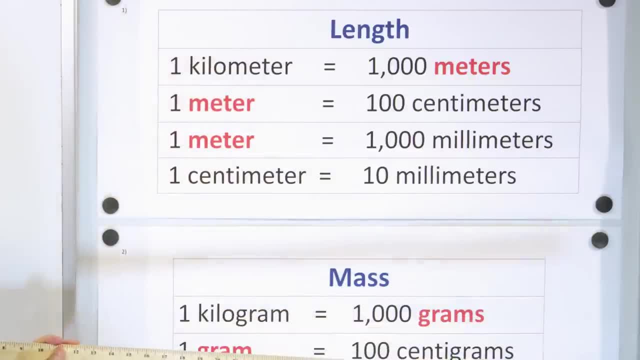 the prefix kilo means 1,000 of something. So one kilometer is just 1,000 of these things called meters. Kilo means 1,000. So it's very simple. You see, one kilometer is 1,000 of. 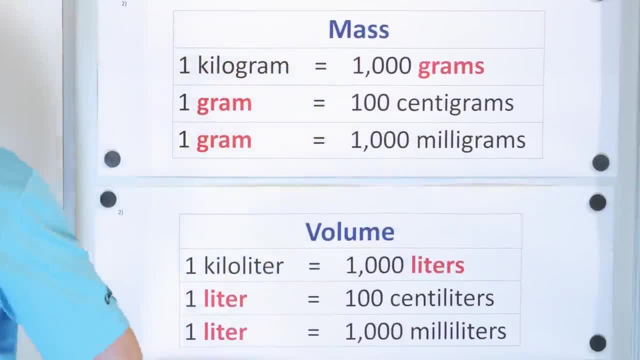 these meters right. One kilogram is just 1,000 of these little grams. which are these smaller units, the size, the amount of mass in this paperclip? One kilogram is just 1,000 of these things. One kilometer is 1,000 of these. 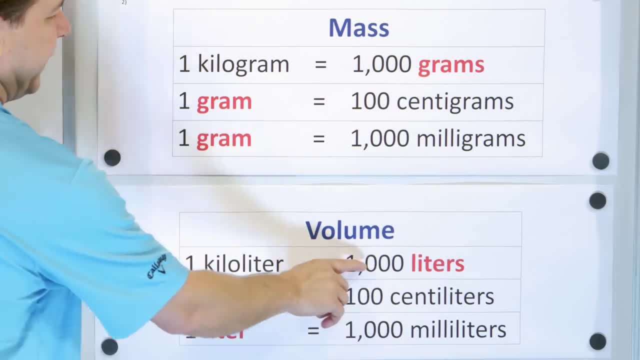 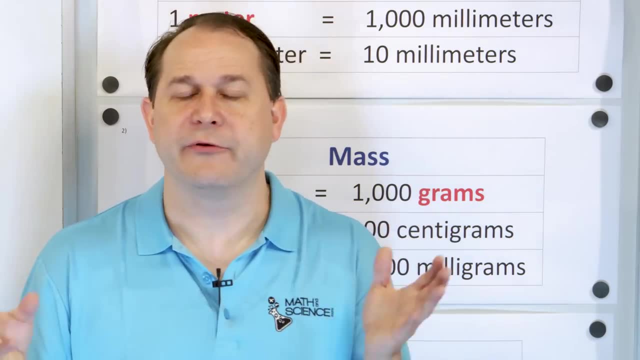 So what do you think a kiloliter will be? It's just going to be 1,000 of these liters. So it's very easy to talk about small and large numbers in the metric system by using the prefixes. If I tell you I have two liters, you know, it's something you can hold in your 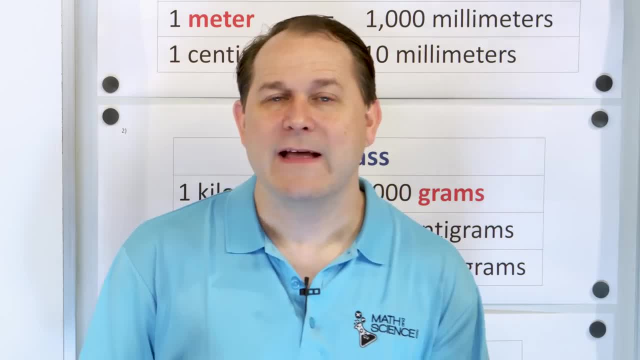 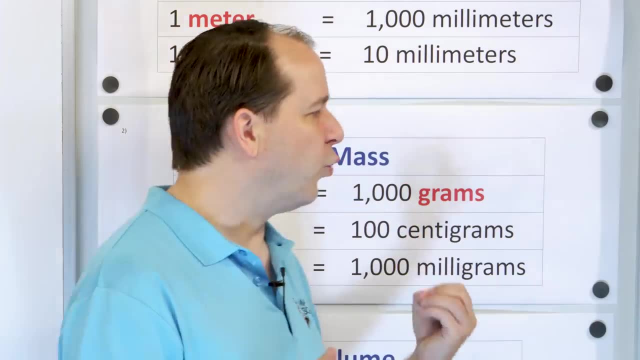 hand right. If I tell you I have two kiloliters, then you know it's 2,000 liters, because kilo means 1,000. And so you can easily talk about sizes of things just by the word. So that's. 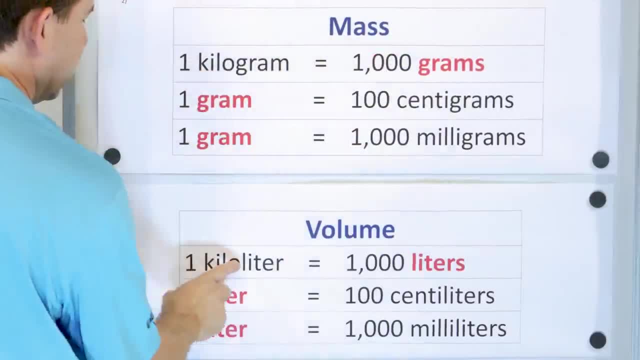 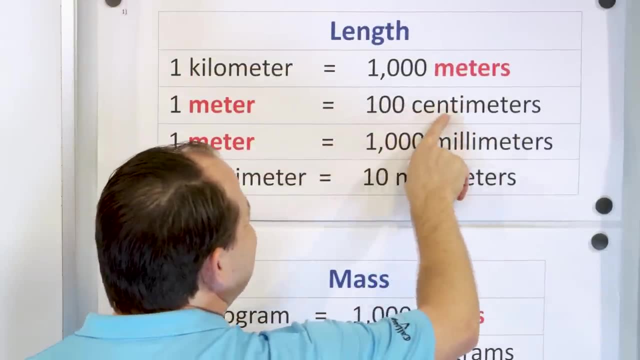 kilo. Kilo means 1,000.. 1,000 meters. kilogram, 1,000 grams, kiloliter, 1,000 liters. all right, Now let's talk about the prefix centi. When you see centi, what does it mean? It doesn't. 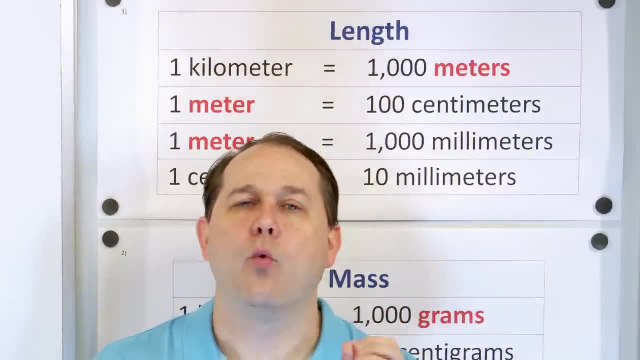 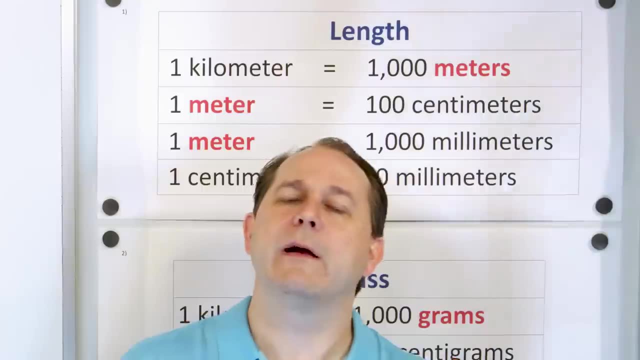 mean what a lot of people think it means. Centi means 100 times smaller. So when I say I have a centimeter, it means I have something 100 times smaller than a meter. You see, kilo means 1,000 times bigger than a meter And centi means 100 times smaller than a meter. 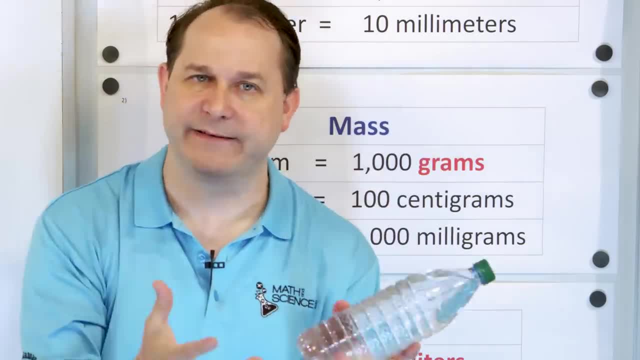 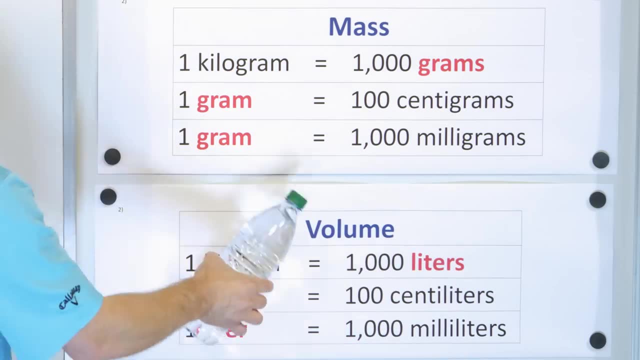 how much space something occupies, How much space in our world does it take? The unit of volume is the basic unit of volume in the metric system is called the liter And this right here is one liter here. So if you can kind of imagine drinking something like this, 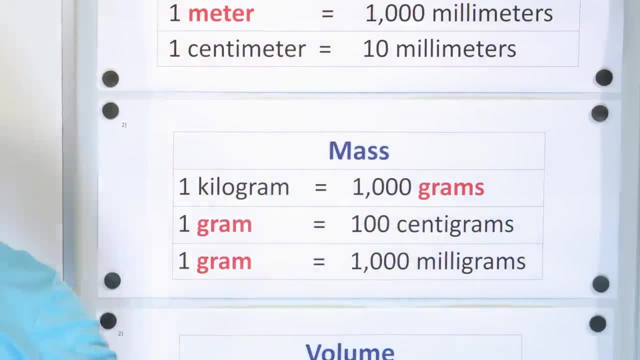 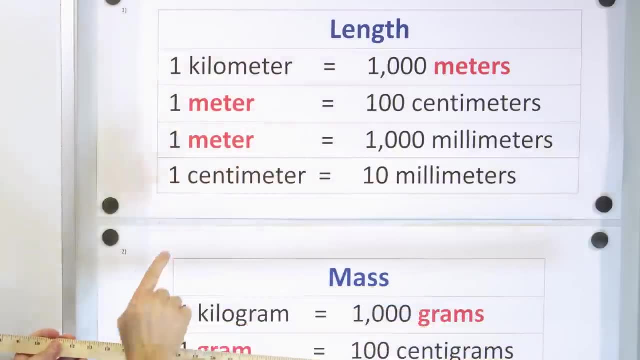 this is one liter, All right. so those are the three main units that we're going to be talking about Now. let's go a little more detail here. You see this chart. We have meters, meters, meters. All right, we have to learn a little bit more. 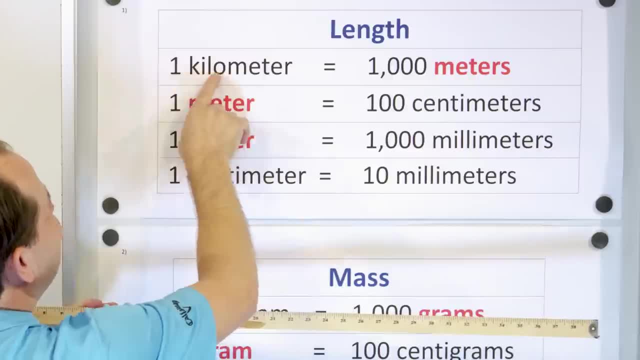 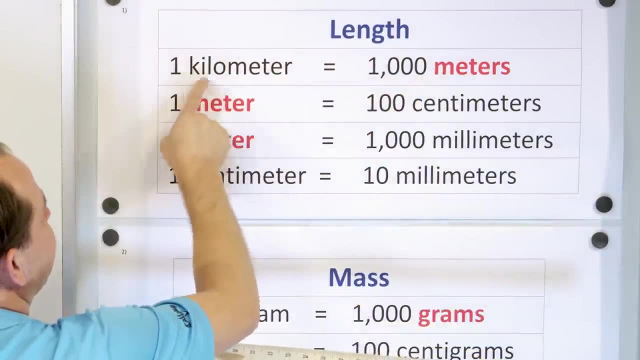 You see we have kilometer, Kilo. the prefix kilo means 1,000 of something. So one kilometer is just 1,000 of these things called meters. Kilo means 1,000, so it's very simple. 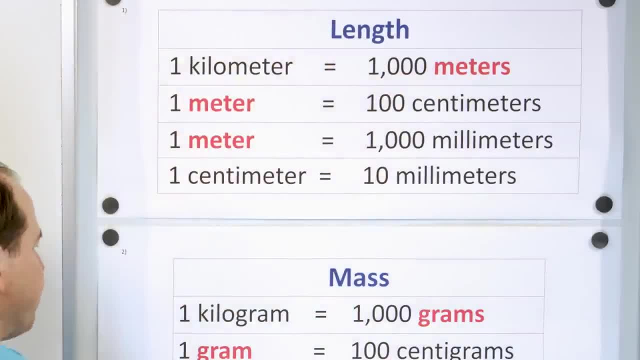 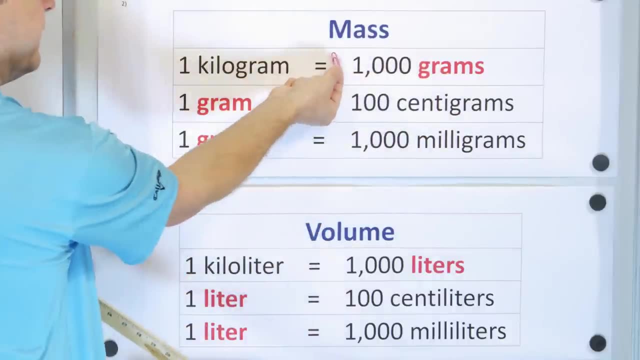 You see, one kilometer is 1,000 of these meters, right? One kilogram is just 1,000 of these little grams. which are these smaller units, the size, the amount of mass in this paperclip? One kilogram is just 1,000 of these things. 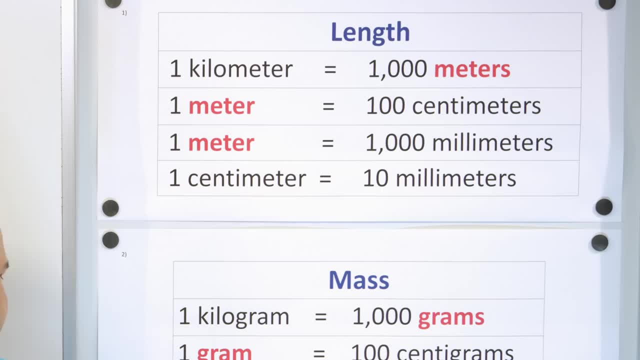 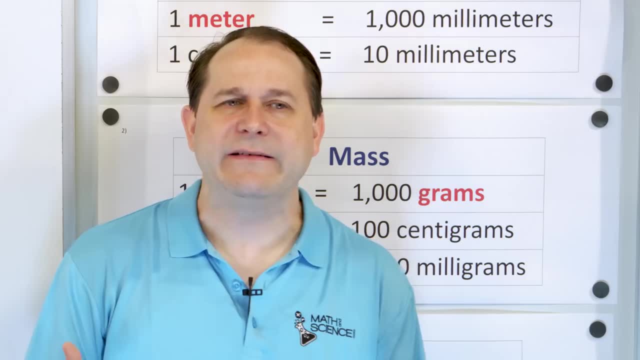 One kilometer is 1,000.. One kilogram is just 1,000 of these meters. So what do you think a kiloliter will be? It's just going to be 1,000 of these liters. So it's very easy to talk about small and large numbers. 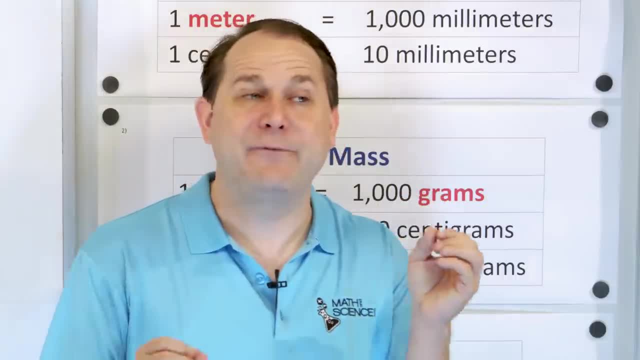 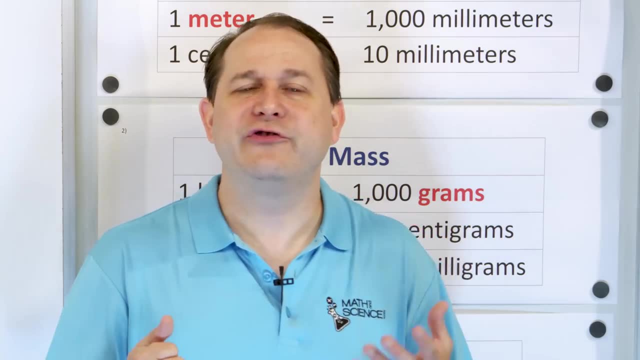 in the metric system by using the prefixes. If I tell you I have two liters, you know it's something you can hold in your hand, right? If I tell you I have two kiloliters, then you know it's 2,000 liters, because kilo means 1,000.. 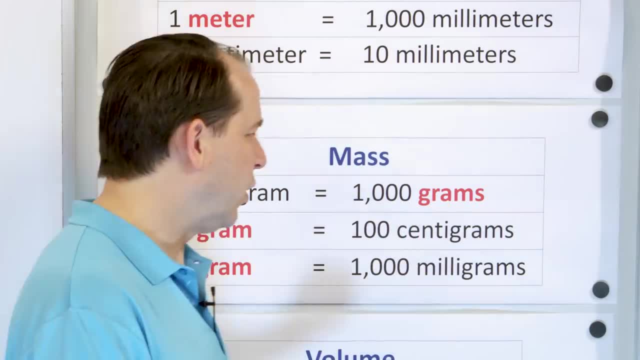 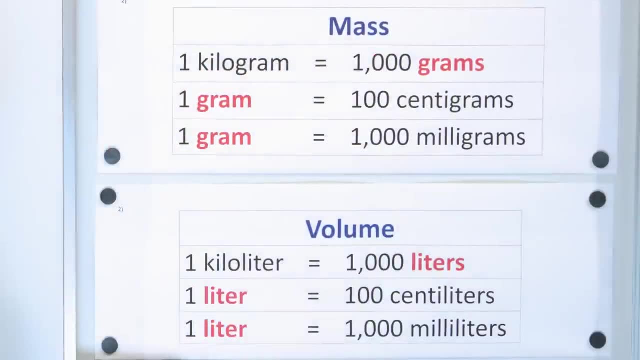 And so you can easily talk about sizes of things just by the word. So that's kilo. Kilo means 1,000.. 1,000 meters, kilogram, 1,000 grams, Kiloliter, 1,000 liters. all right, 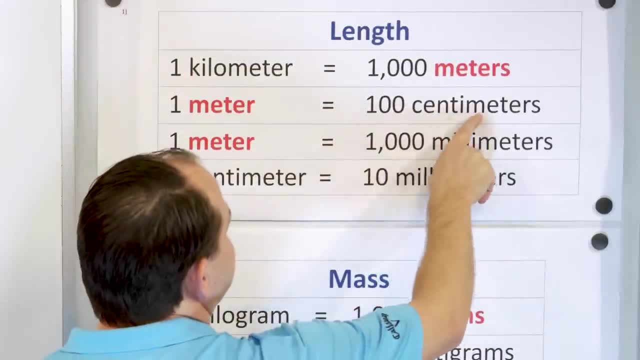 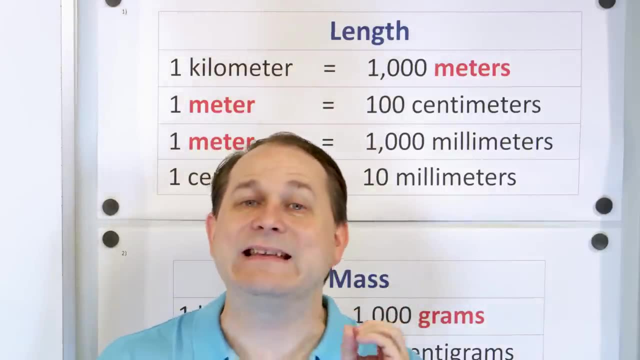 Now let's talk about the prefix centi. When you see centi, what does it mean? It doesn't mean what a lot of people think it means. Centi means 100 times smaller. So when I say I have a centimeter, 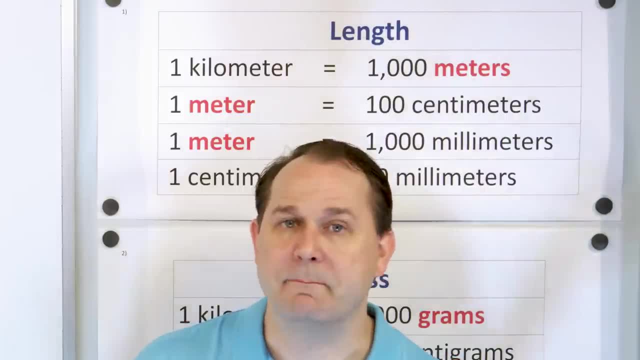 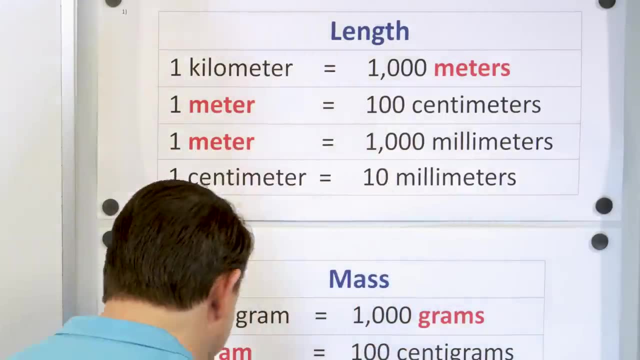 it means I have something 100 times smaller than a meter. You see, kilo means 1,000 times bigger than a meter and centi means 100 times smaller. So on my meter stick here on my meter stick, see, here's a meter from all the way here to here is a meter. 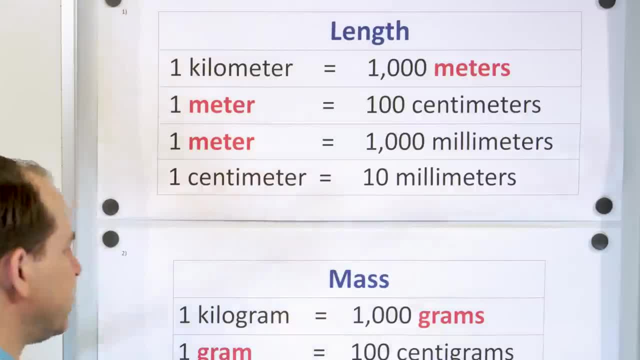 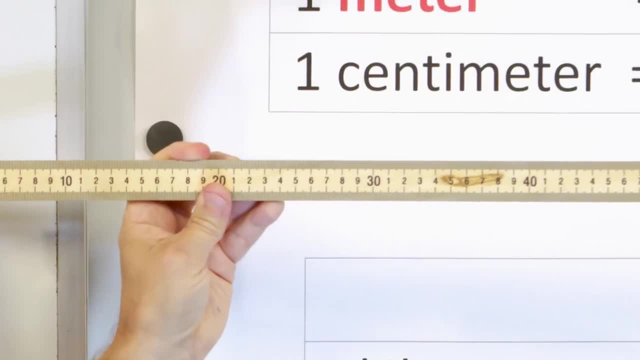 Centi means 100 times smaller. So on my meter stick, here on my meter stick, see, here's a meter. From all the way here to here is a meter, But if you look closely you probably can't see it on the camera. This meter stick is divided into 100 markings that go all the 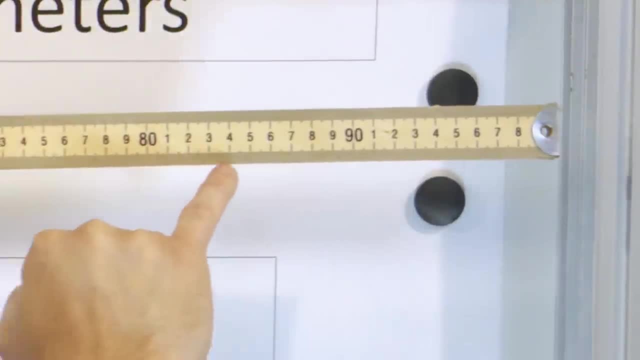 way to the end. Here's 40,, 50, 60,, 70,, 80. And you have the numbers in here and the 90 and then 100. So if you take this meter stick and chop it into 100 little pieces, one of 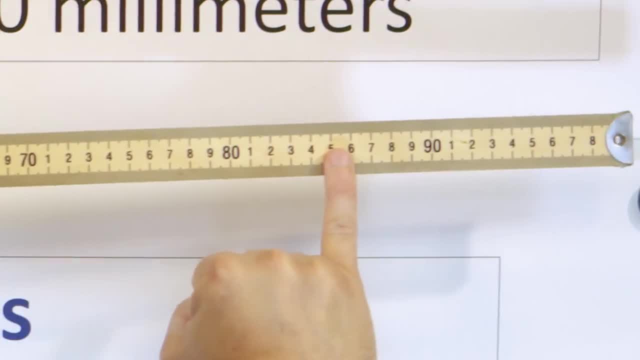 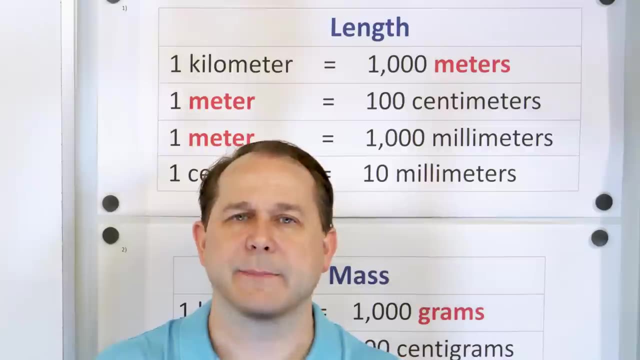 those little pieces about the width of my finger. the width of my finger here is called a centimeter. Centimeter is 100 times smaller than the base unit. Everything is related to the base unit. Here is a meter. Centimeter is 100 times smaller Now because centimeter is 100 times. 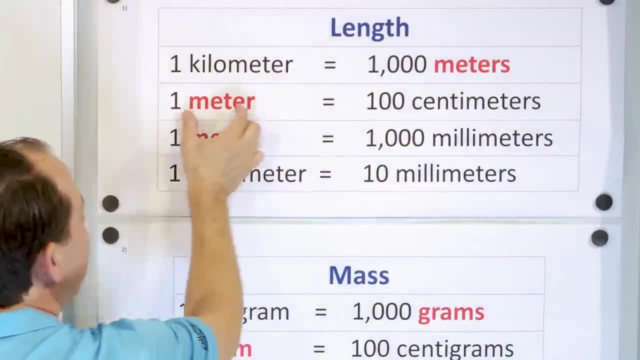 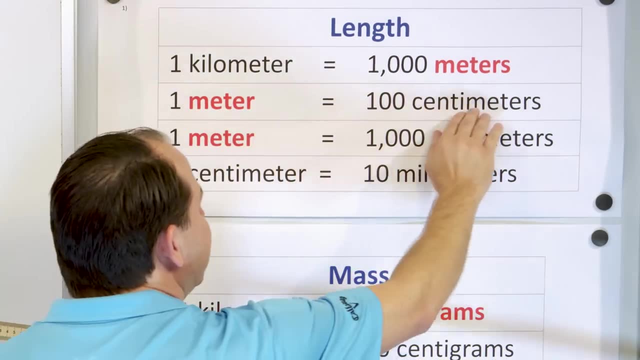 smaller. it takes 100 of these little bitty centimeters to make one meter. That's what this is showing you: 100 of these little centimeters makes one meter. Now, if that's what's happening for length, what do you think is happening in terms of mass grams? Remember the basic. 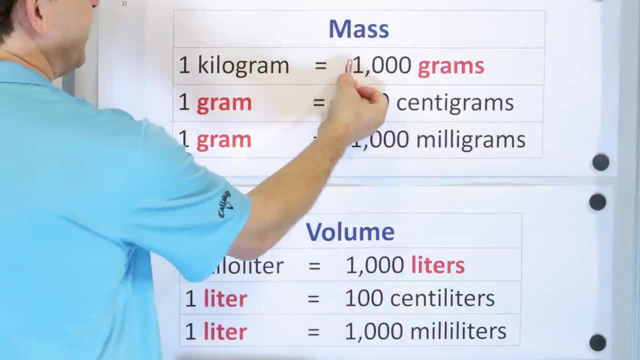 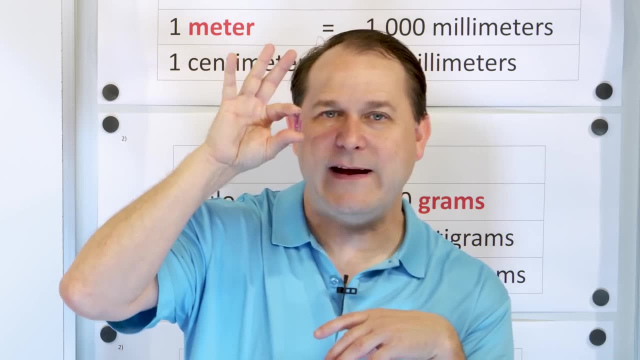 unit of mass is this paperclip Gram. So if I have something called a centigram, it's 100 times smaller than this little thing right in mass. So it's going to take 100 centigrams to be the same as one gram, because 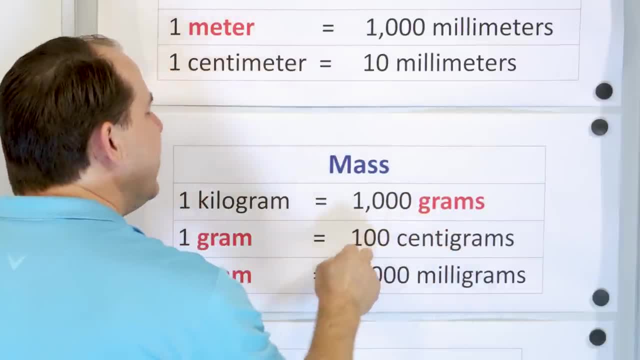 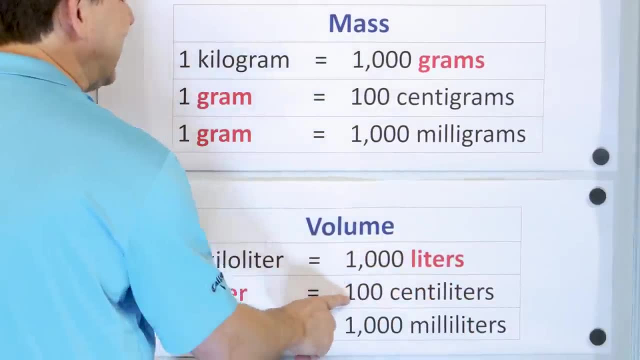 these centigrams are tiny, tiny, tiny. They're 100 times smaller than this. So it takes 100 of these centigrams to make one gram. Same thing for liters: 100 centiliters. I need 100 of these tiny little centiliters to equal one liter. Remember the prefix: centi means. 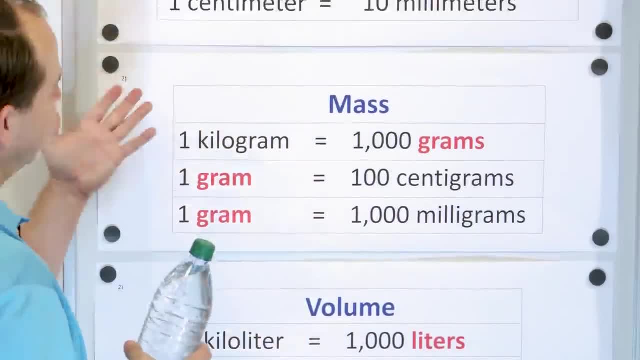 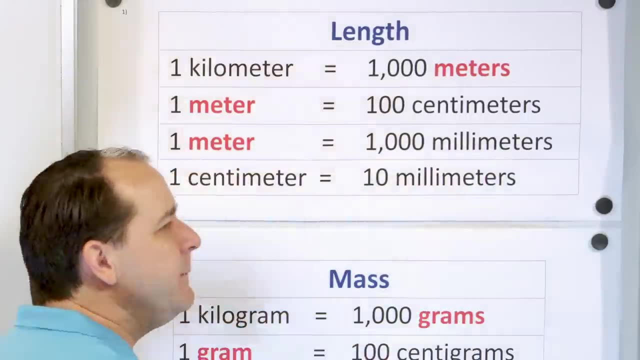 1,000 times smaller, all right. And then the last one, the last big one we're going to talk about is millimeters. I know everybody's probably heard of millimeters. So what does milli mean? The prefix milli? 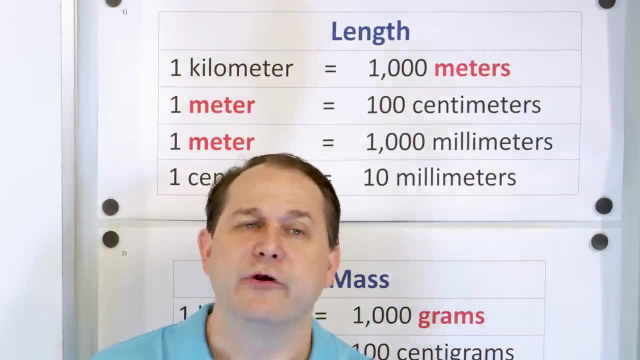 means 1,000 times smaller, right? So one millimeter is tiny. Think of millipede, Think of centipede. even right, Centipede is 100 times smaller. Millipede is 1,000 times smaller, So there's. 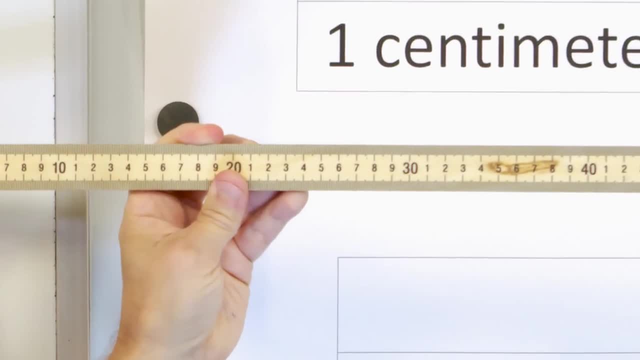 But if you look closely you probably can't see it on the camera. This meter stick is divided into 100 markings that go all the way to the end. Here's 40,, 50,, 60,, 70,, 80,. 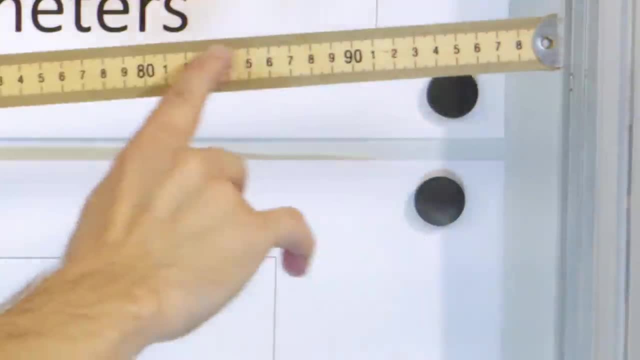 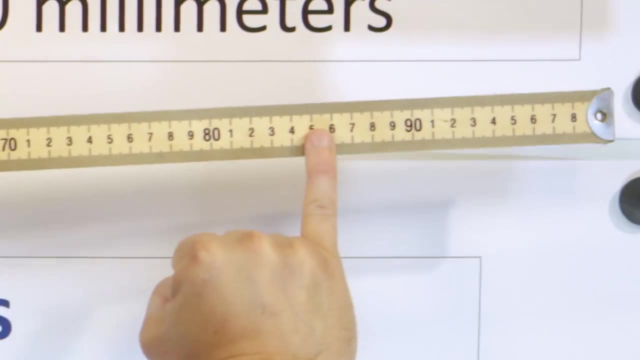 and you have the numbers in here and then 90, and then 100.. So if you take this meter stick and chop it into 100 little pieces, one of those little pieces about the width of my finger, the width of my finger here- 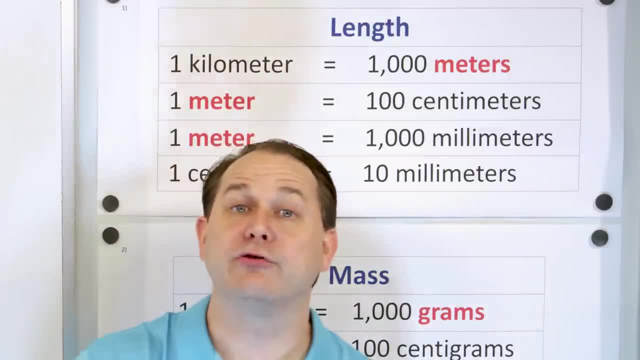 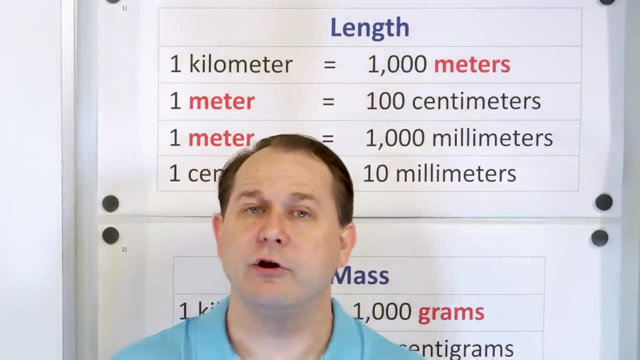 is called a centimeter. Centimeter is 100 times smaller than the base unit. Everything is related to the base unit. Here is a meter. Centimeter is 100 times smaller. Now, because centimeter is 100 times smaller, it takes 100 of these little bitty centimeters. 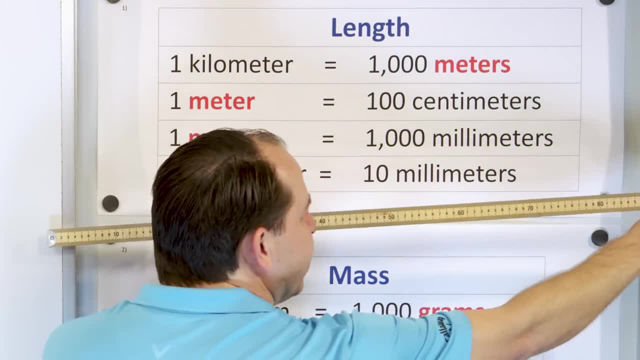 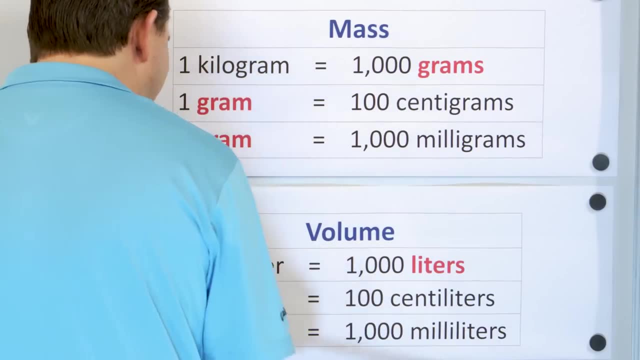 to make one meter. That's what this is showing you: 100 of these little centimeters makes one meter. Now, if that's what's happening for length, what do you think is happening in terms of mass grams? Remember the basic unit. 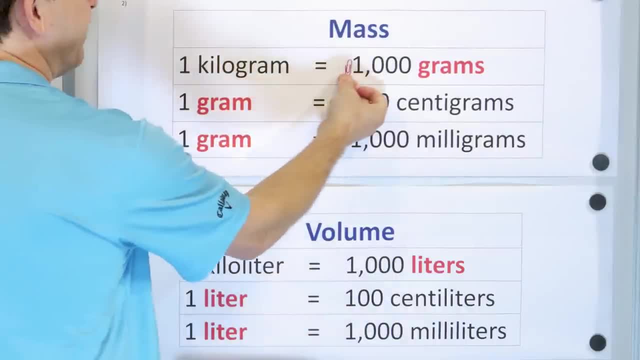 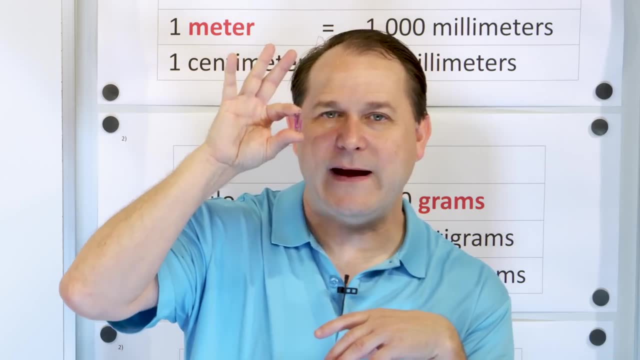 remember, the basic unit of mass is this paperclip, a gram. So if I have something called a centigram, it's 100 times smaller than this little thing right in mass. So it's gonna take 100 centigrams. 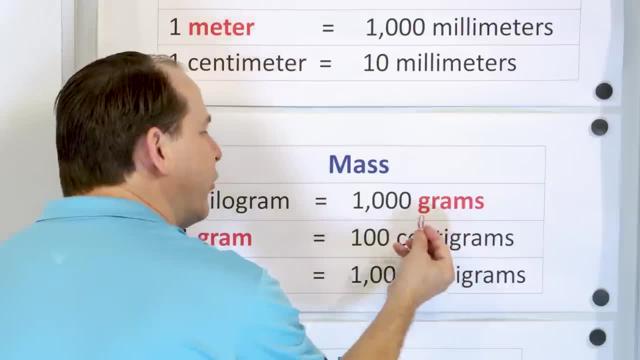 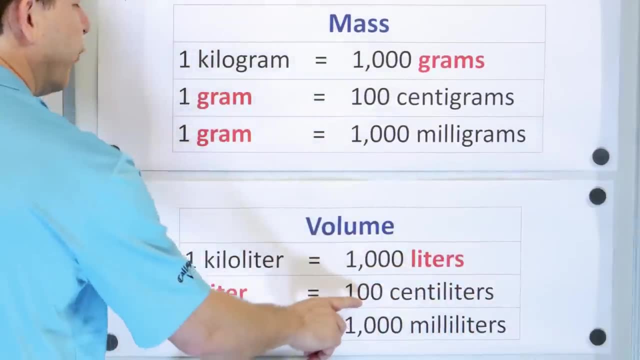 to be the same as one gram, because these centigrams are tiny, tiny, tiny. They're 100 times smaller than this, So it takes 100 of these centigrams to make one gram. Same thing for liters: 100 centiliters. I need 100 of these. 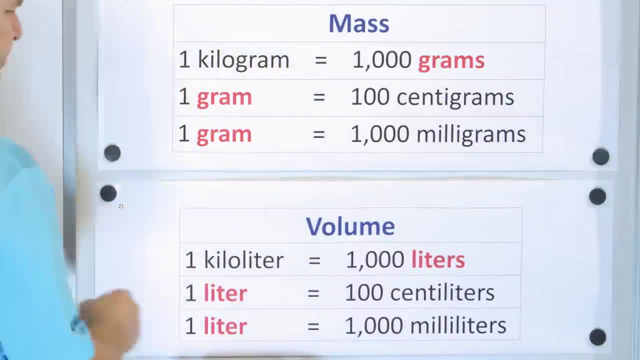 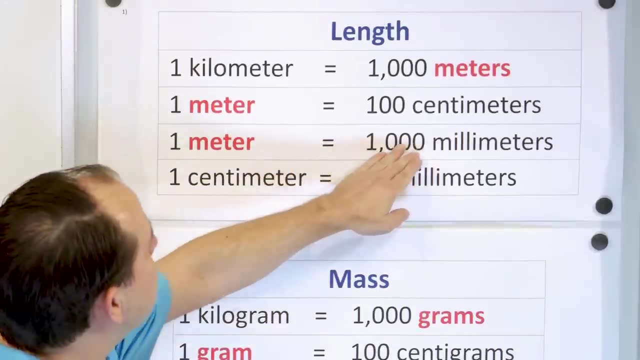 tiny little centiliters to equal one liter. Remember the prefix: centi means 100 times smaller, all right. And then the last one, the last big one we're gonna talk about is millimeters. I know everybody's probably heard of millimeters. 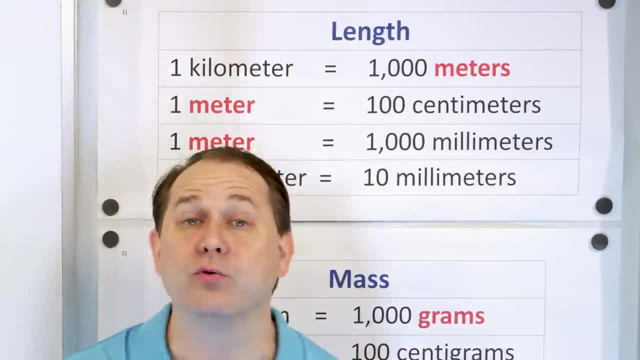 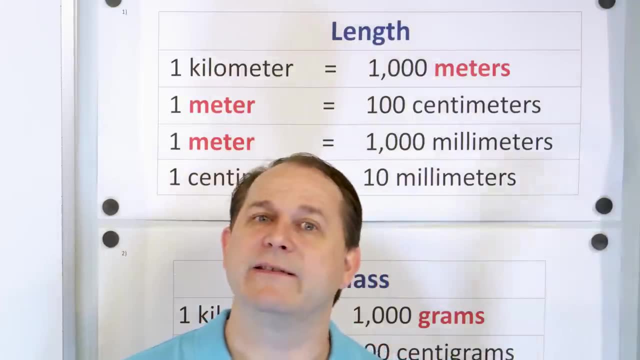 So what does milli mean? The prefix milli means 1,000 times smaller, right. So one millimeter is tiny. Think of millipede, think of centipede. even right, Centipede's 100 times smaller. 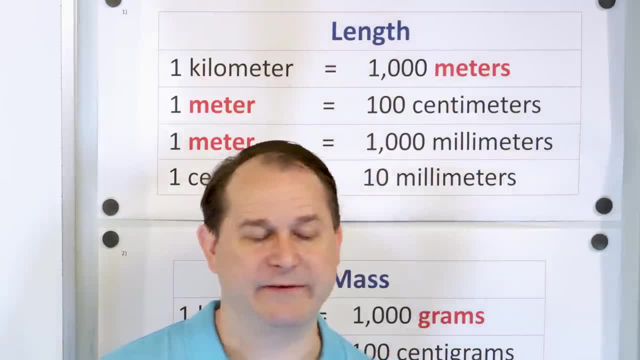 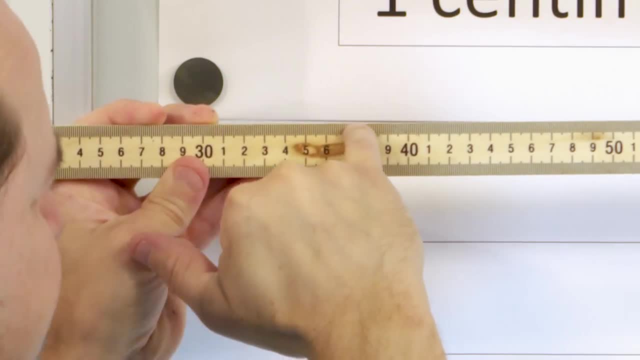 Millipede is 1,000 times smaller, So there's no way you're gonna see this on the camera. but if you get an actual meter stick, there's little bitty marks across the top that you're not gonna be able to see on the screen. 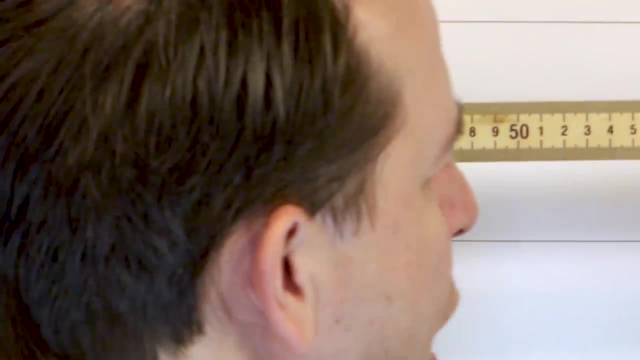 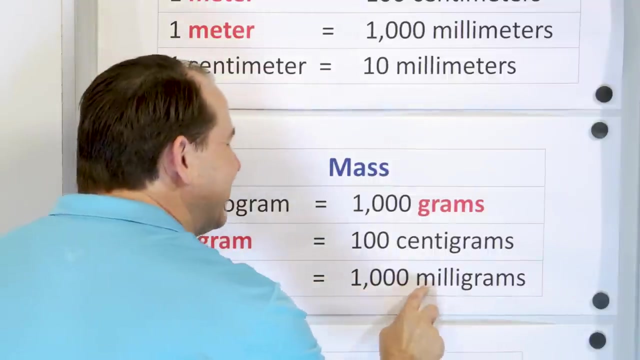 but I can see them here, And there's 1,000 of these little markings that go all the way from here to here. So 1,000 of these tiny, tiny millimeters will equal one meter, And 1,000 of these tiny, tiny milligrams. 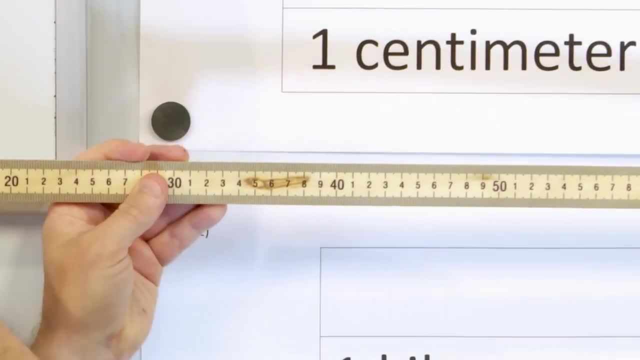 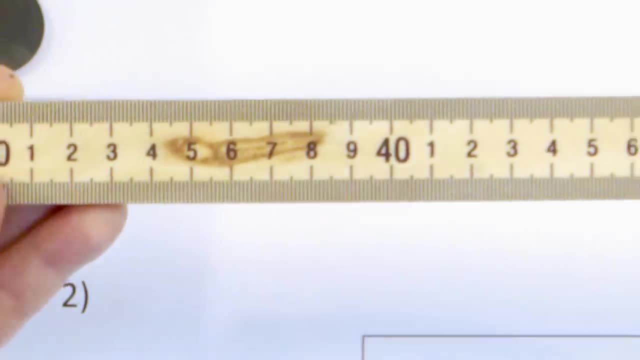 no way you're going to see this on the camera, but if you get an actual meter stick, there's little bitty marks across the top that you're not going to be able to see on the screen, but I can see them here, And there's 1,000 of these little markings that go all the way. 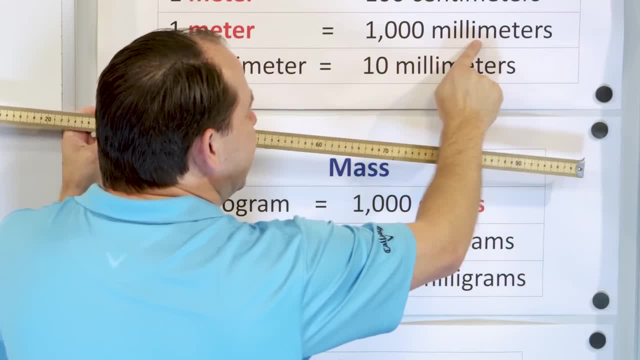 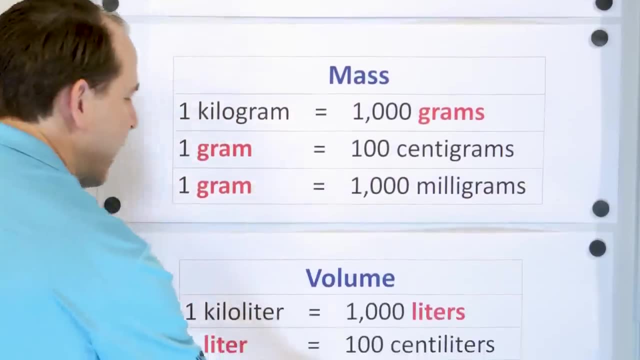 from here to here. So 1,000 of these tiny, tiny millimeters will equal one meter, And 1,000 of these tiny tiny milligrams is the same as one gram, And 1,000 of these tiny tiny milliliters is the same as one liter. So the main thing I want you to pull out of 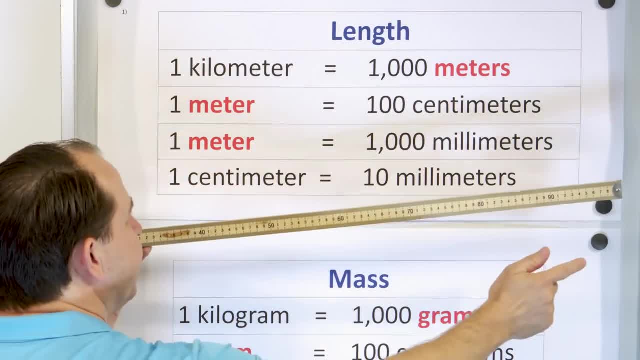 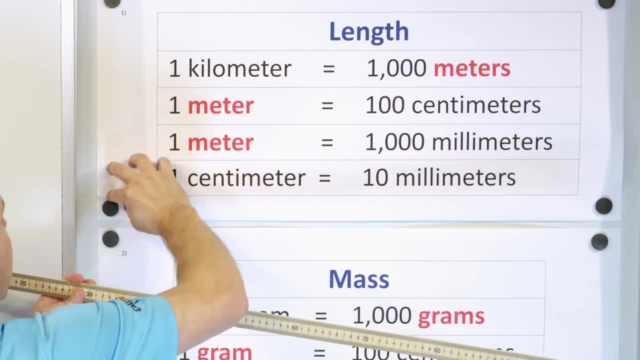 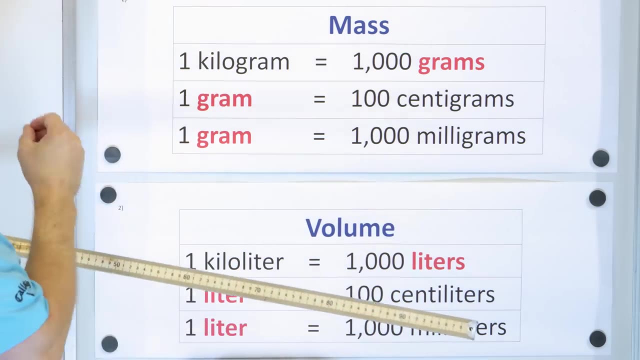 this is the base unit of length, is this thing called a meter? And when we have a kilometer, 1,000 times the length of this, because a kilo means 1,000 times bigger right, And then we have kilogram, 1,000 times of a gram, and then kiloliter, 1,000 liters, So kilo. 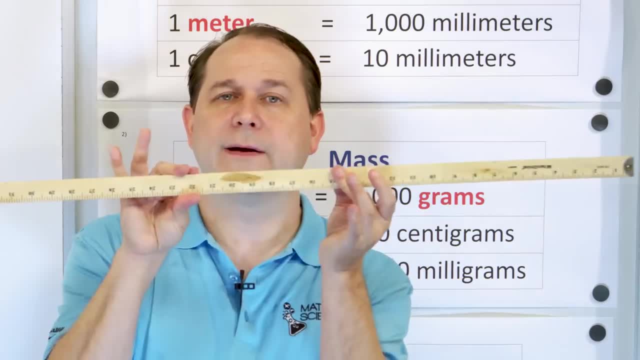 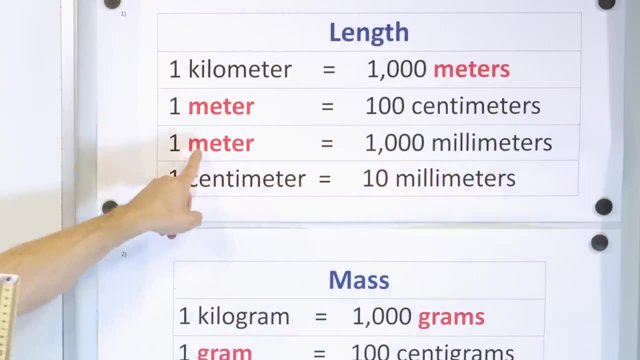 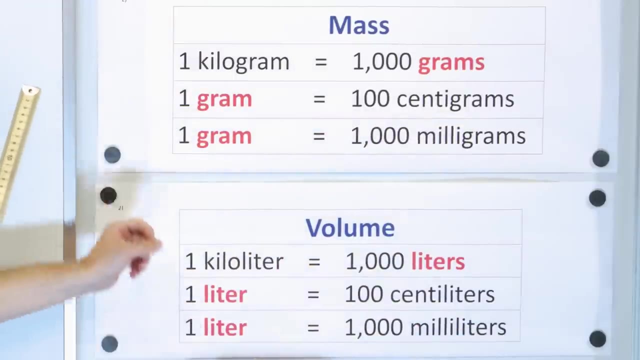 means 1,000 times larger than whatever the base unit is. Milli means 1,000 times smaller. So it takes 1,000 of these millimeters to equal a meter. It takes 1,000 of these milligrams to equal a gram. It takes 1,000 of these milliliters to equal a liter, And then for centi it's. 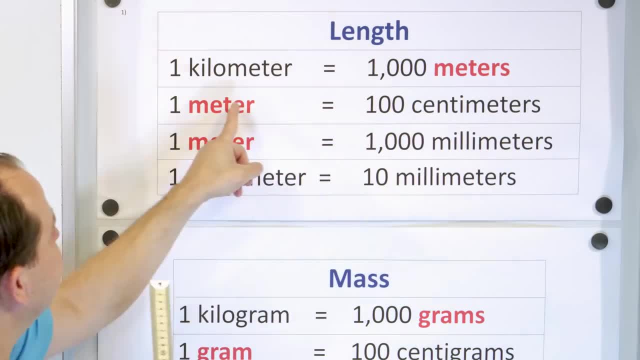 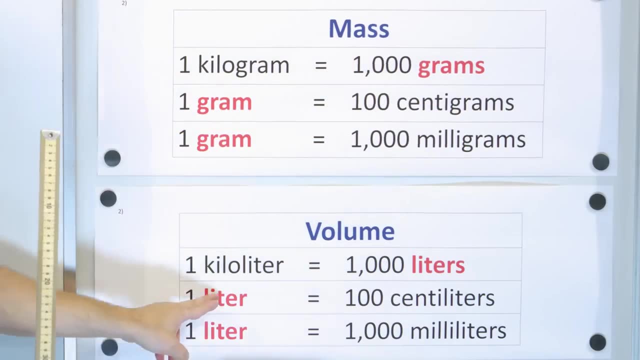 100 times smaller. So it takes 100 of these centimeters to equal a meter. which are these markings? the width of my finger is a centimeter And it takes 100 of these centigrams to equal a gram. And it takes 100 of these centiliters to equal a liter. And then I have one more. 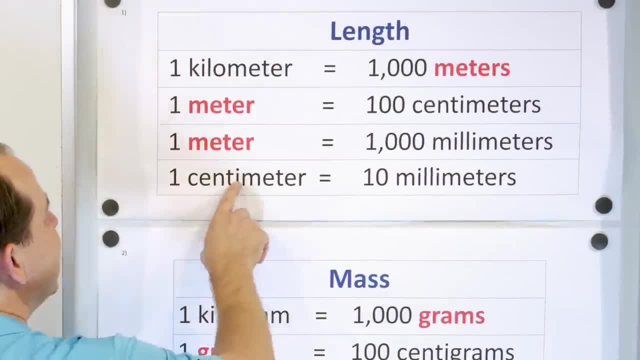 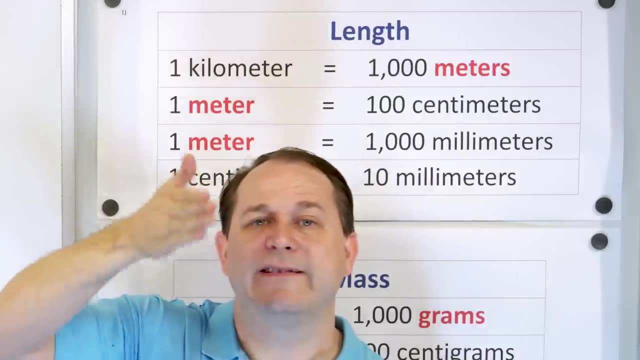 up here that we also use quite a bit as well, And that is that one centimeter is 10 millimeters And you can see that on there. If you, if you look at a centimeter on a meter stick, you can see that there's 10 little millimeter markings between there. So this one here is: 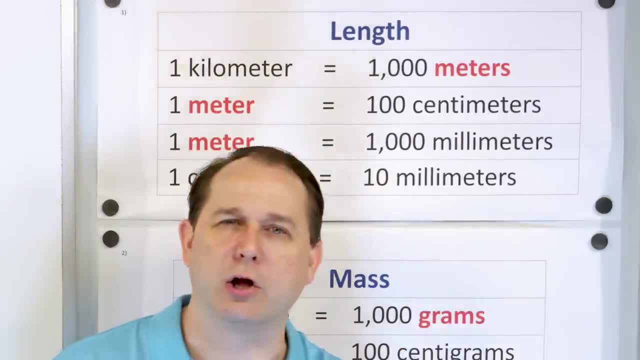 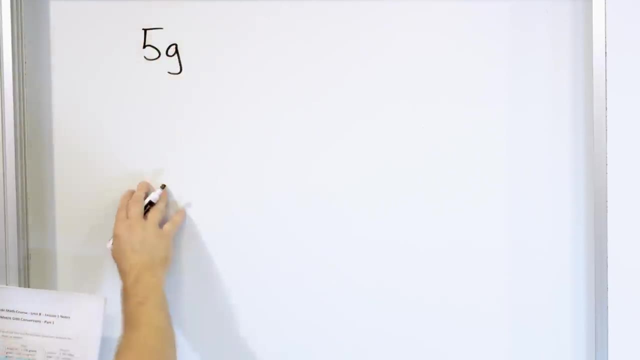 separate from the others. that one centimeter is equal to 10 of these smaller things called millimeters. So now that we have all of that kind of background out of the way, we're ready to start solving our problems. All right, For our first problem. I want to start off with a unit of five grams. 5g means 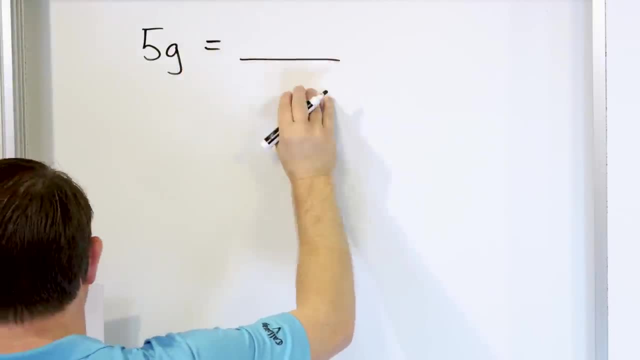 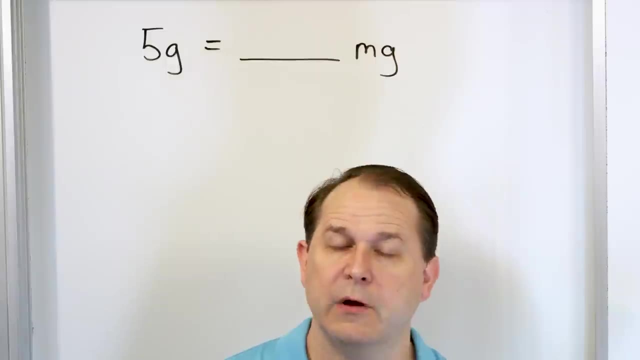 five grams And I want you to convert that to some number of milligrams. Now, a lot of students, when they look at something like this, they just freeze up and they don't know what to do. So the first step is to know. I want to go from grams to milligrams, And if you don't, 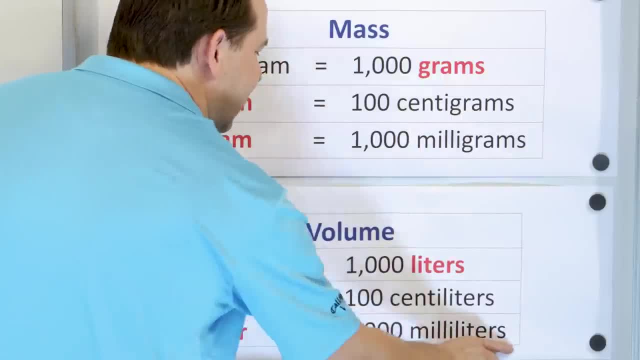 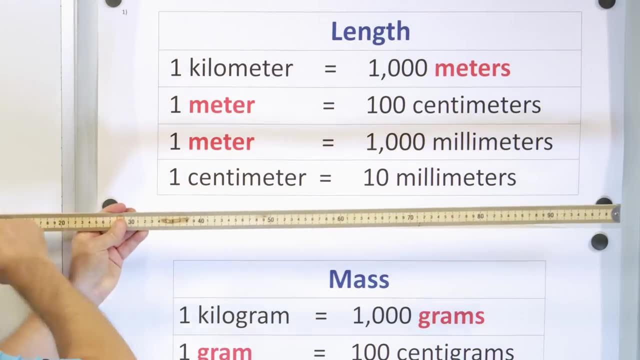 is the same as one gram, And 1,000 of these tiny, tiny milliliters is the same as one liter. So the main thing I want you to pull out of this is the base unit of length. is this thing called a meter? 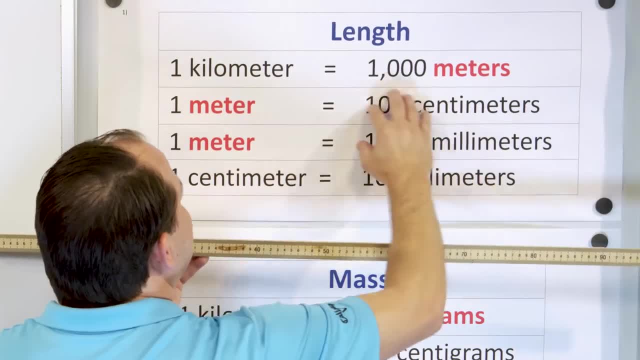 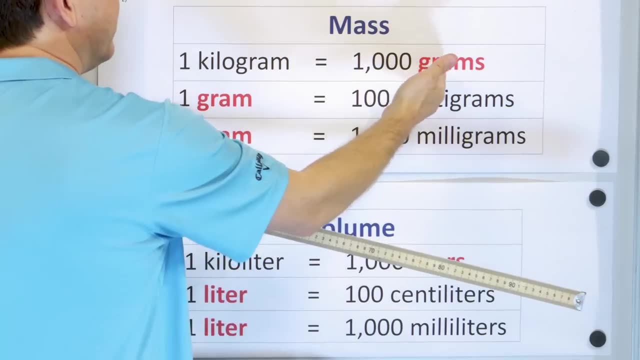 And when we have a kilometer it's 1,000 times the length of this, because a kilo means 1,000 times bigger right. And then we have kilogram 1,000 times of a gram, and then kiloliter- 1,000 liters. 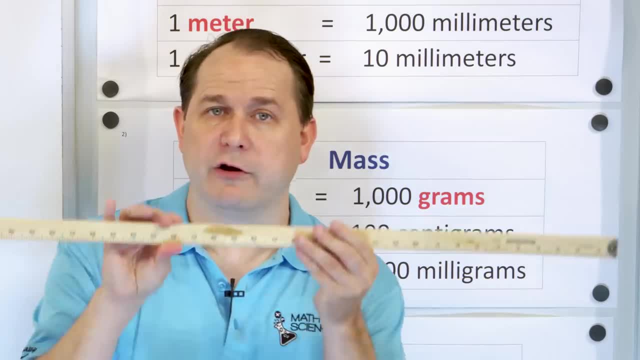 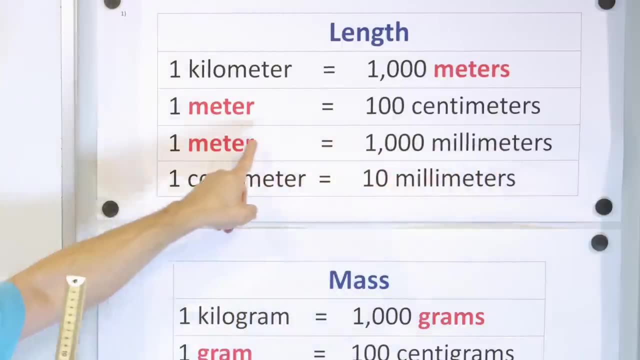 So kilo means 1,000 times larger than whatever the base unit is. Milli means 1,000 times smaller, So it takes 1,000 of these millimeters to equal a meter. It takes 1,000 of these milligrams to equal a gram. 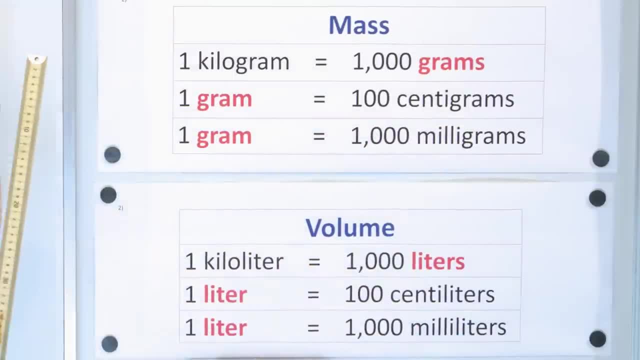 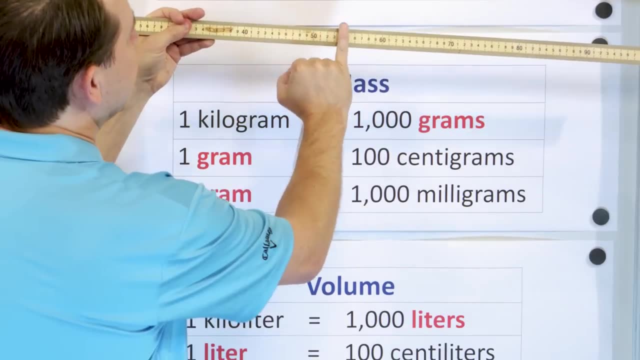 It takes 1,000 of these millimeters to equal a gram. And then for centi it's 100 times smaller. So it takes 100 of these centimeters to equal a meter. which are these markings? the width of my finger is a centimeter. 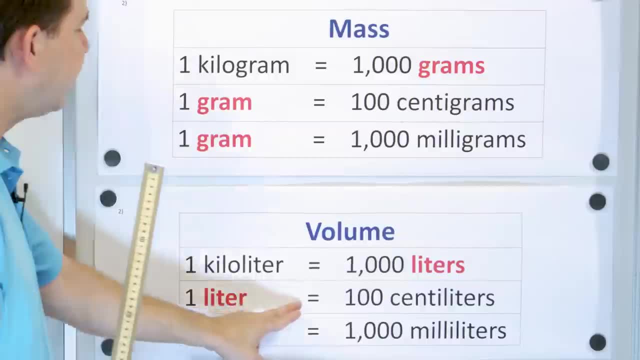 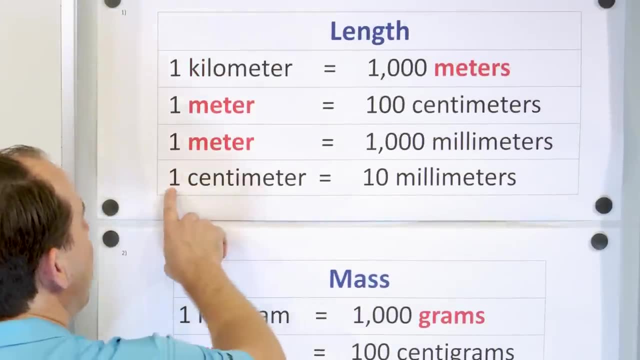 And it takes 100 of these centigrams to equal a gram, And it takes 100 of these centiliters to equal a liter. And then I have one more up here that we also use quite a bit as well, And that is that one centimeter is 10 millimeters. 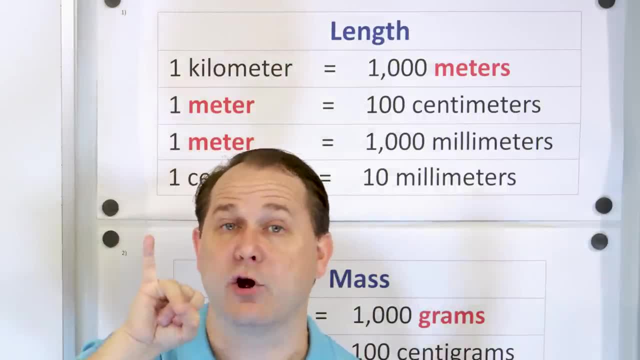 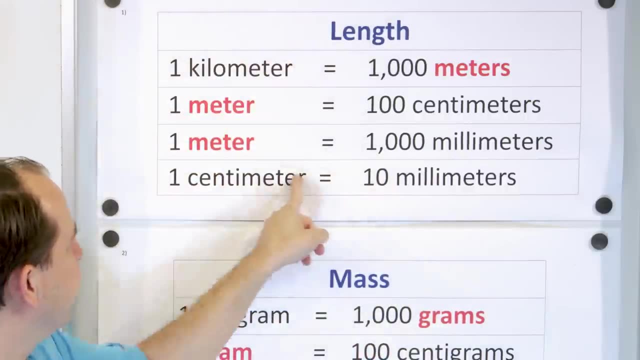 And you can see that on there. If you look at a centimeter on a meter stick, you can see that there's 10 little millimeter markings Between there. So this one here is kind of separate from the others. That one centimeter is equal to 10 of these smaller things. 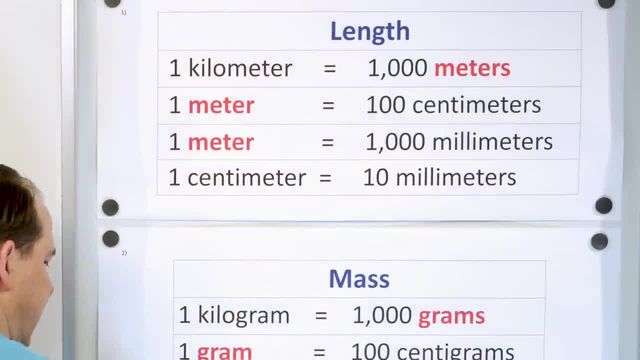 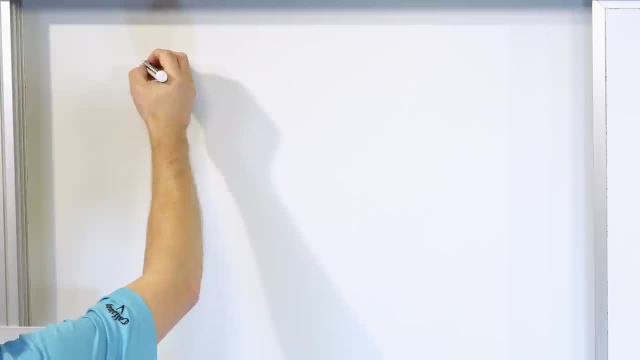 called millimeters. So now that we have all of that kind of background out of the way, we're ready to start solving our problems. All right, for our first problem. I want to start off with a unit of 5 grams. 5g means 5 grams. 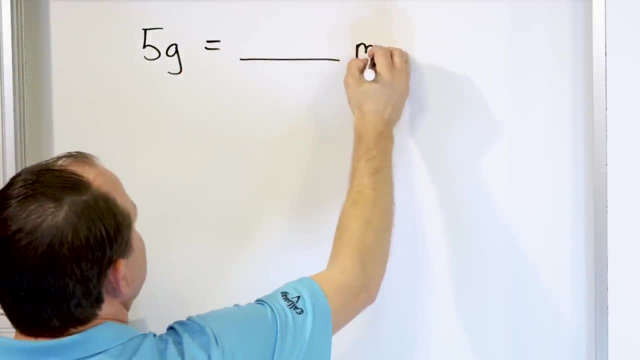 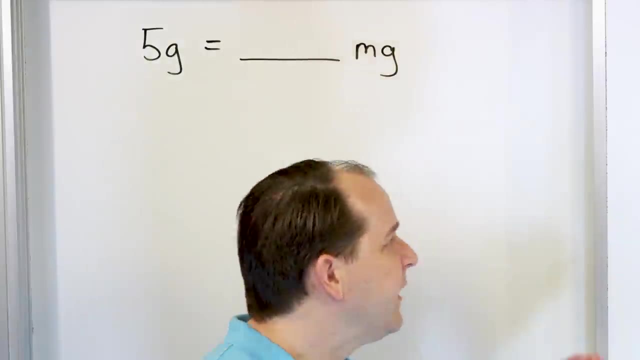 And I want you to convert that to some number of milligrams. Now, a lot of students, when they look at something like this, they just freeze up and they don't know what to do. The very first step is to know. I want to go from grams to milligrams. 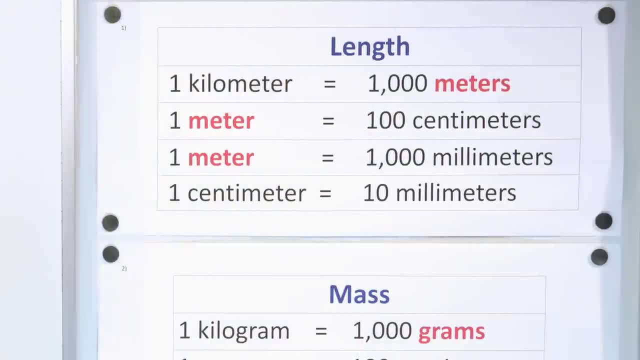 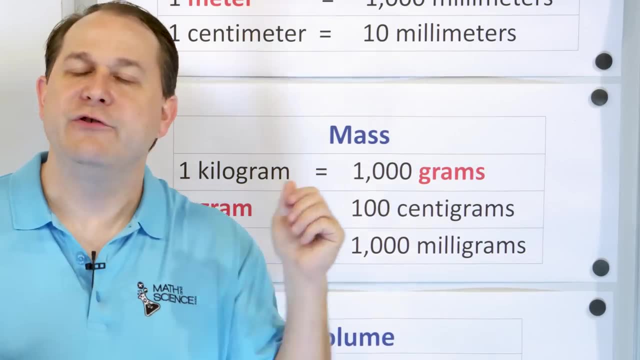 And if you don't remember then go back to the table. We go down to mass and we're looking at grams and milligrams. So here's grams and here's milligrams. So if you don't remember then you just look at the table. 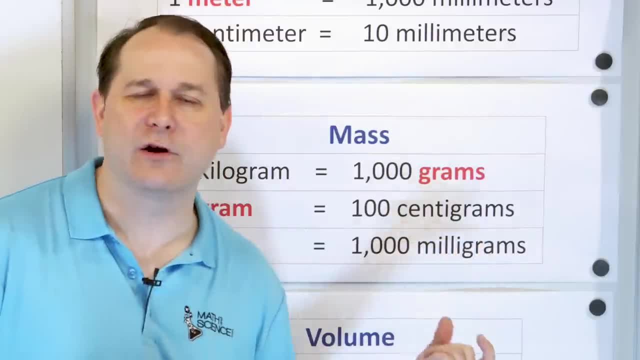 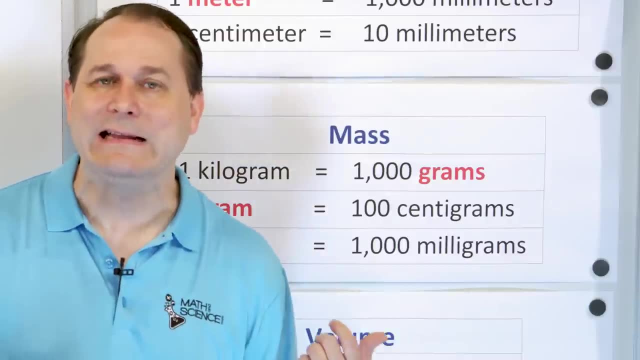 One gram is the same as a thousand of these tiny, tiny things called milligrams, Because a milligram is a thousand times smaller than a gram. So to get one gram I need a thousand of these tiny, tiny things to get there. 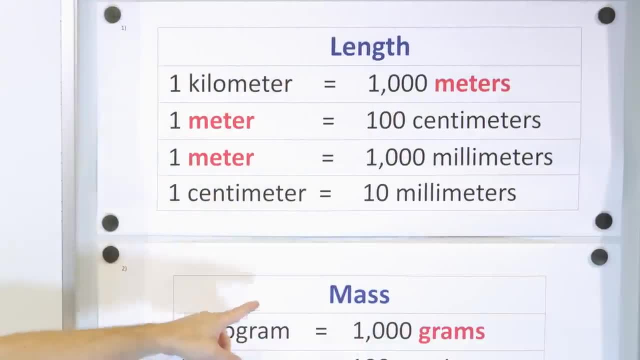 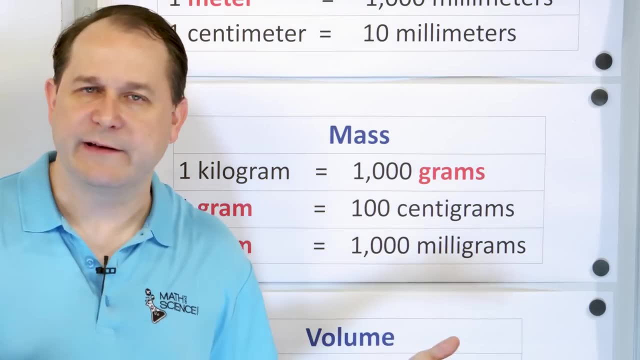 remember, then go back to the table. We go down to mass and we're looking at grams and milligrams. So here's grams and here's milligrams. So if you don't remember, then you just look at the table. One gram is the same as a thousand of these tiny, tiny things called milligrams. 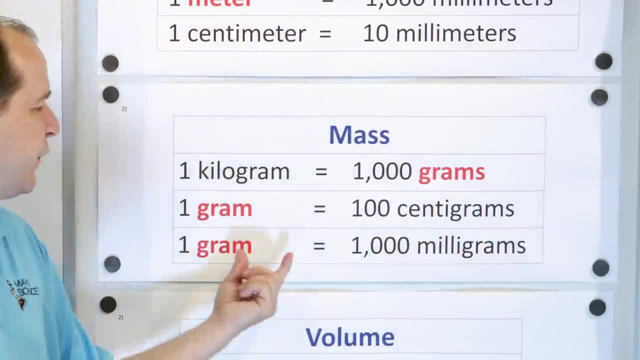 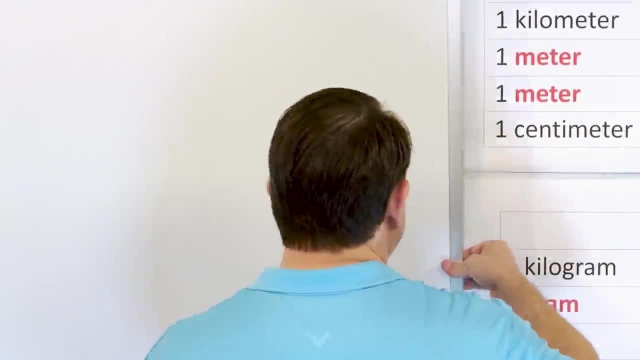 because a milligram is a thousand times smaller than a gram. So to get one gram, I need a thousand of these tiny tiny things to get there. So one gram is one thousand milligrams. Now what you need to do is figure out a way to multiply or divide to make this thing work. 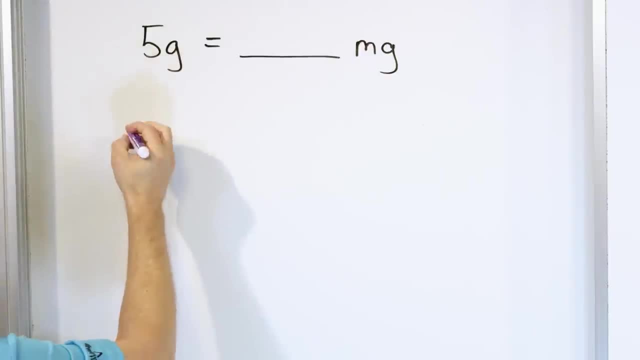 This is how I want you to solve every unit conversion problem. I want you to write down what you have been given five grams, draw a line under it and draw a vertical line next to it, And right here I'm going to write down: one gram is 1000 milligrams. Now the 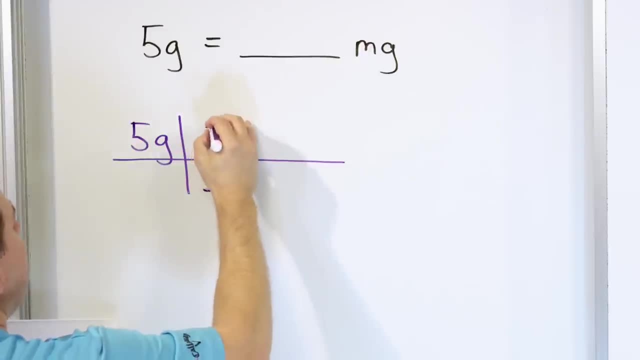 way I'm going to write it down is I'm going to put one gram on the bottom and 1000 mg milligrams. This thing right here is the conversion factor. One gram, 1000 milligrams. That comes straight off my chart. Now I could 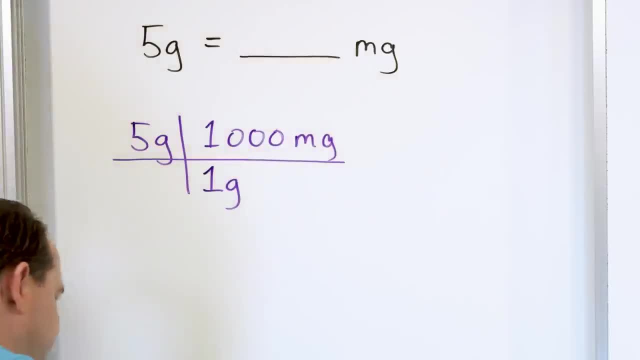 write it like this. I could flip it over and write it upside down, but we are going to see in a minute why we're writing it this way. When we write it this way, with a gram on the bottom and a gram on the top, the grams cancel each other. The reason the grams cancel: 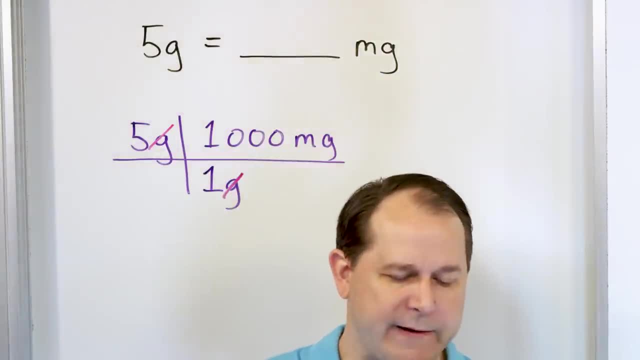 each other when they're on the bottom and the top is just like fractions. When you have a, you know, a zero on the top and a zero on the bottom of a fraction, that's going to have numbers. you can cancel the zeros Because, basically, what you can think about doing, 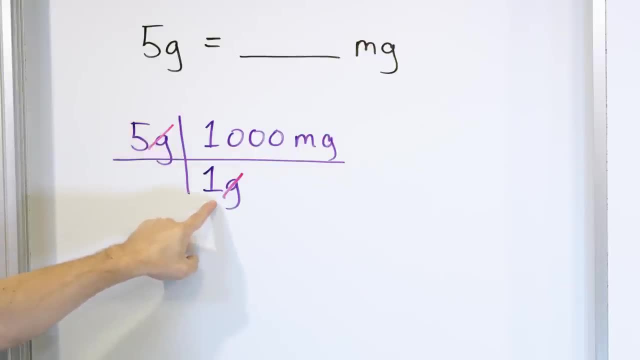 is. you can divide the top by grams and the bottom by grams and it gets rid of them, Just like any fraction. you can divide top and bottom by whatever you want to get rid of it. I could divide this by grams and this by grams and it will get rid of the grams. 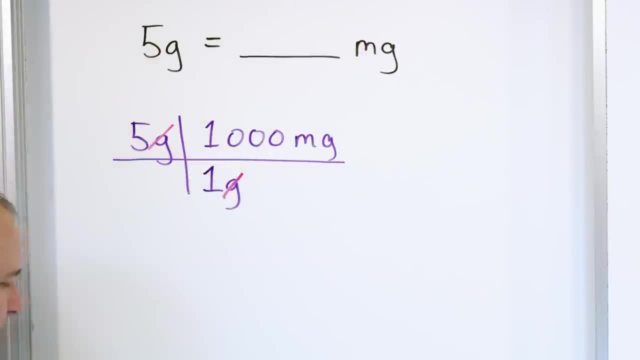 An easier way to think of it is: if you see grams on the top and on the bottom, you just get rid of them. Now, the only unit I have left is milligrams. So what this is telling me is that to go from here to here, I need to take the five. 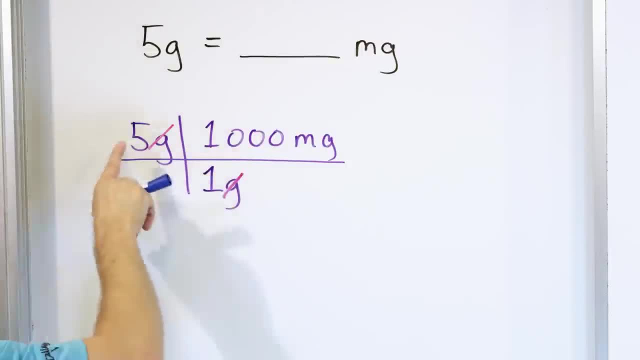 One, Multiply by a thousand and then divide by one. Everything on the top gets multiplied and everything on the bottom you divide by that. So what is five times a thousand? Well, the easiest way to think about that, you can write it down: five times a thousand. but 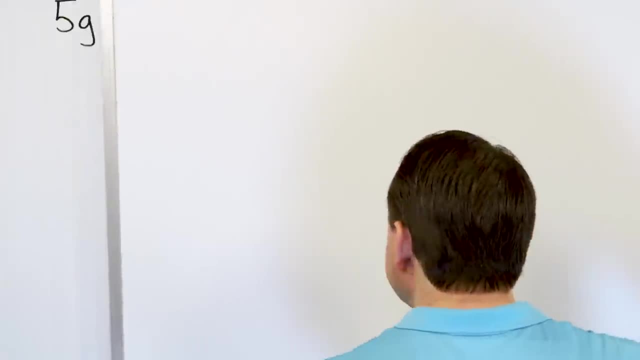 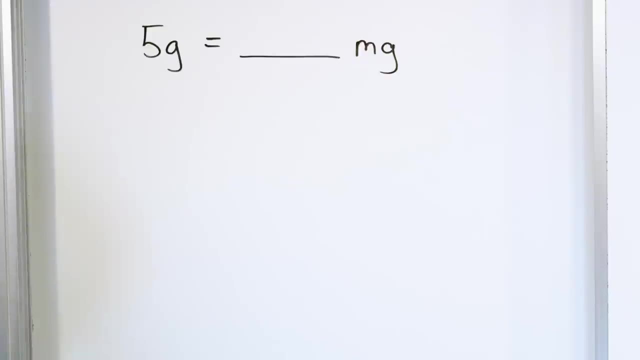 So one gram is one thousand milligrams. Now what you need to do is figure out a way to multiply or divide to make this thing work. This is how I want you to solve every unit conversion problem. I want you to write down what you have been given. 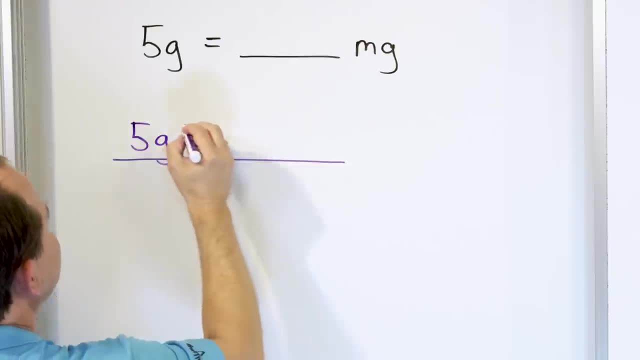 five grams, draw a line under it and draw a vertical line next to it, And right here I'm going to write down: one gram is one thousand milligrams. Now, the way I'm going to write it down is I'm going to put one gram on the bottom. 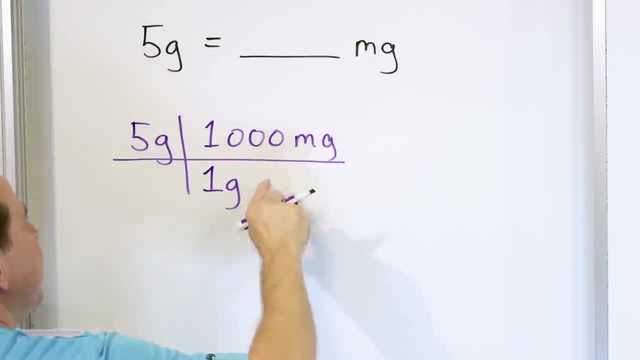 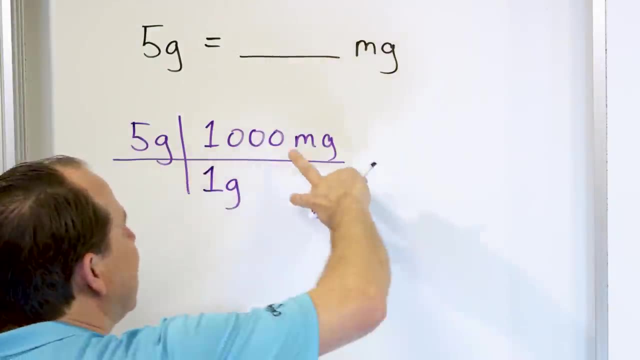 and one thousand mg milligrams. This thing right here is the conversion factor: One gram, one thousand milligrams. That comes straight off my chart. Now I could write it like this. I could flip it over and write it upside down: 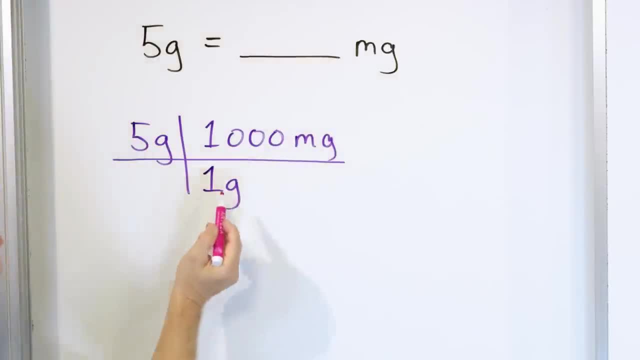 but we are going to see in a minute why we're writing it this way. When we write it this way, with a gram on the bottom and a gram on the top, the grams cancel each other. The reason: the grams cancel each other when they're on the bottom and the top. 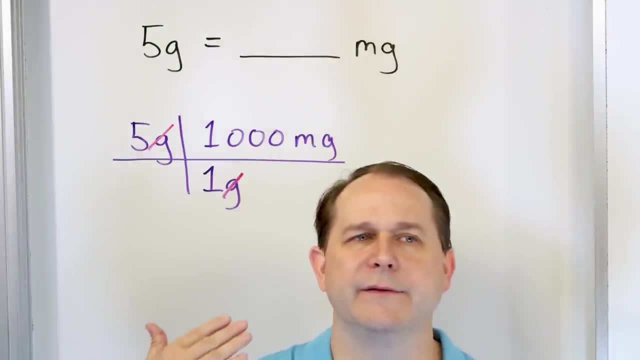 is just like fractions: When you have a zero on the top and a zero on the bottom of a fraction that has numbers, you can cancel the zeros, Because basically, what you can think about doing is you can divide the top by grams and the bottom by grams. 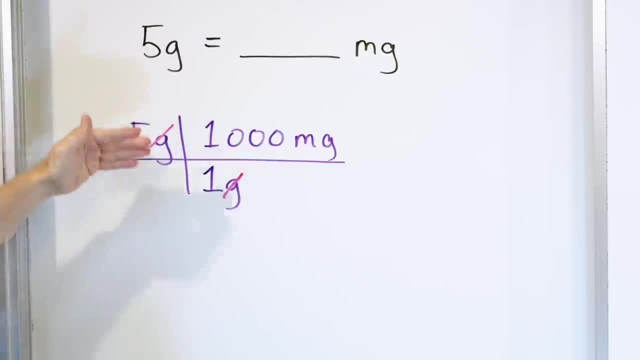 and it gets rid of them. Just like any fraction, you can divide top and bottom by whatever you want to get rid of it. I could divide this by grams and this by grams and it will get rid of the grams. An easier way to think of it is if you see grams on the top. 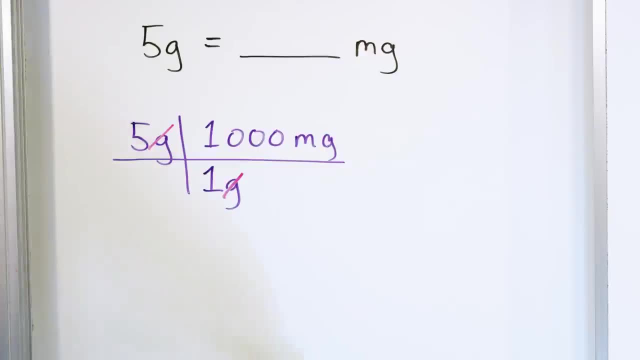 and on the bottom, you just get rid of them. Now, the only unit I have left is milligrams. So what this is telling me is that to go from here to here, I need to take the five, multiply by 1,000, and then divide by one. 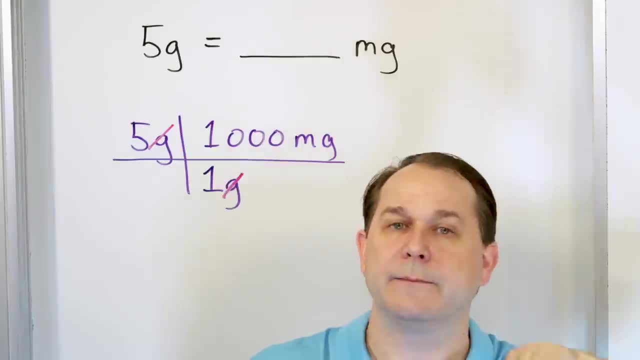 Everything on the top gets multiplied and everything on the bottom you divide by that. So what is five times 1,000?? Well, the easiest way to think about that, you can write it down: five times 1,000,. 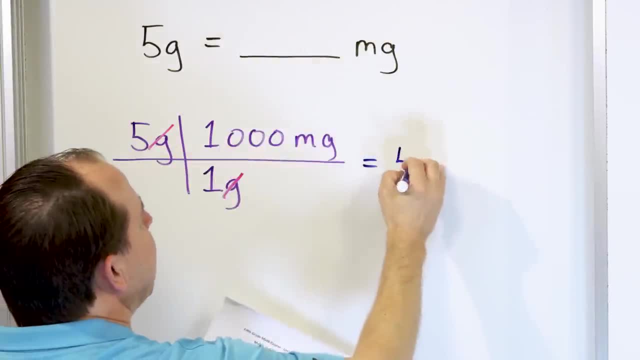 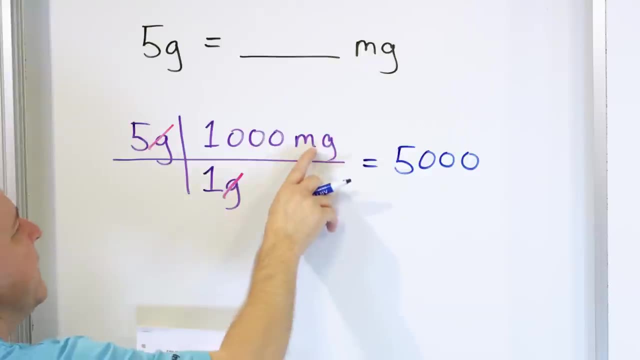 but just cover up the zeros. Five times one is five, And then, since I covered up the zeros, I have to add the zeros back in, So it's 5,000.. Five times 1,000 is 5,000.. 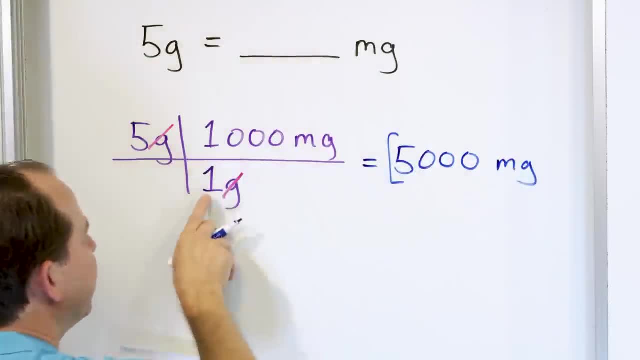 The only unit left is milligrams, And I've divided by one here, which doesn't change anything. So what I've done is I've taken five times 1,000, and then I divided by one. Now I could go down here and write five times 1,000. 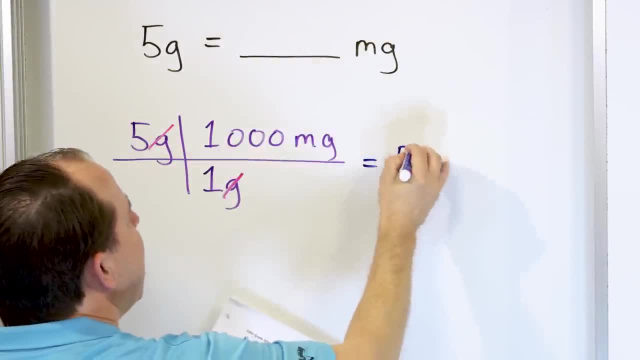 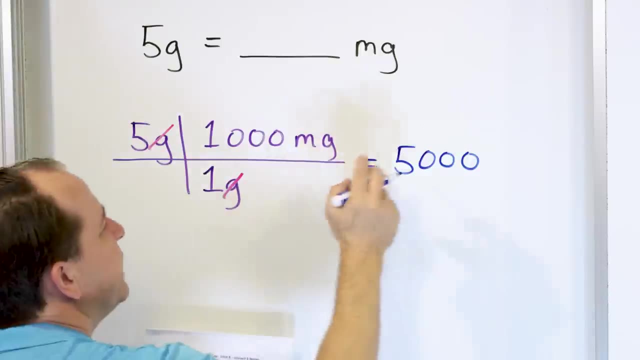 just cover up the zeros. Five times one is five, And then, since I covered up the zeros, I have to add the zeros back in, So it's five thousand. Five times a thousand is five thousand. The only unit left is milligrams. 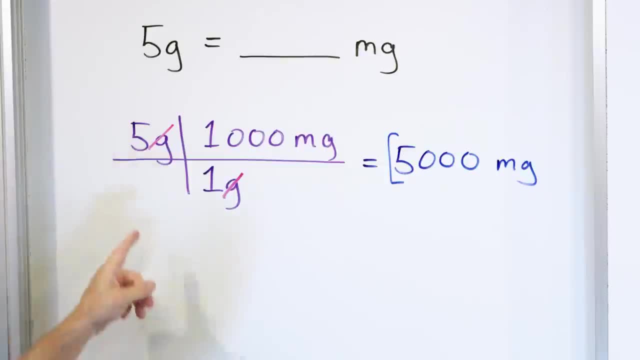 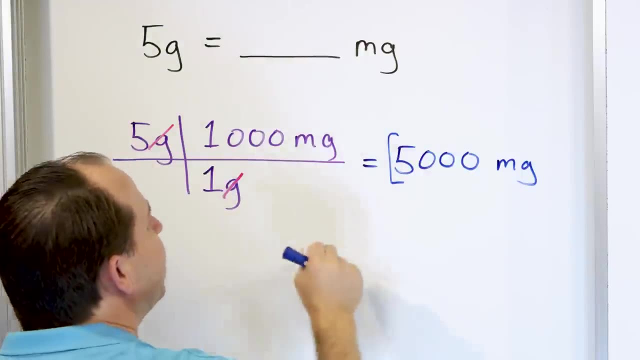 And I've divided by one here, Which doesn't change anything. So what I've done is I've taken five times a thousand and then I divided by one. Now I could go down here and write five times a thousand and do it all, but I'm trying to also show you how to multiply and divide by powers of ten When. 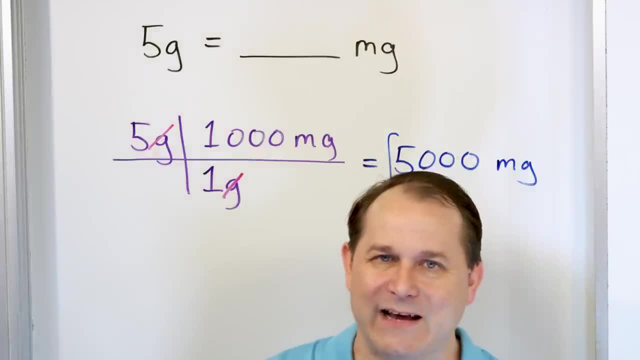 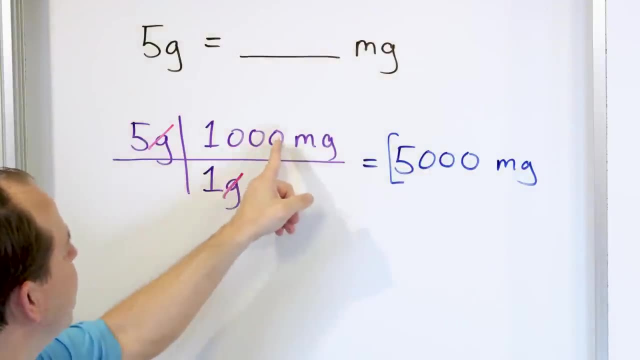 you multiply by a power of ten- meaning you multiply by ten or a hundred or a thousand or ten thousand or a hundred thousand- then it's very easy, because all you do is ignore the zeros- Five times one is five- and then you add the zeros back in, So when you multiply, 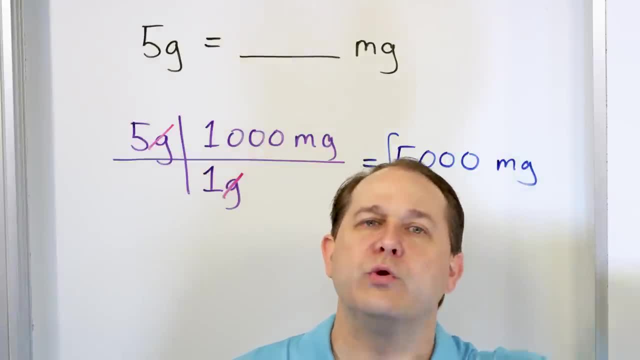 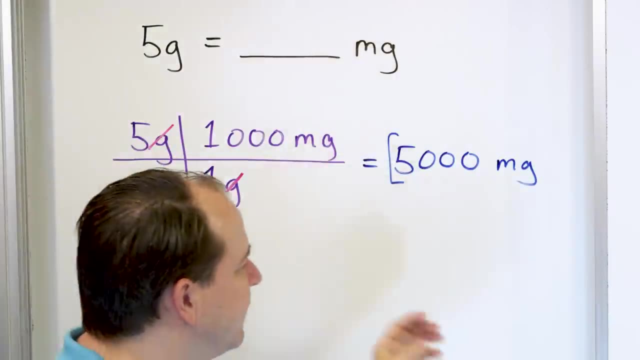 by powers of ten. it's very simple. You just add the zeros at the end When you divide by powers of ten. we'll see what we do here in just a minute. But for here we are telling ourselves that five grams is five thousand milligrams. Does that make sense? Well, I know here that one gram is the same. 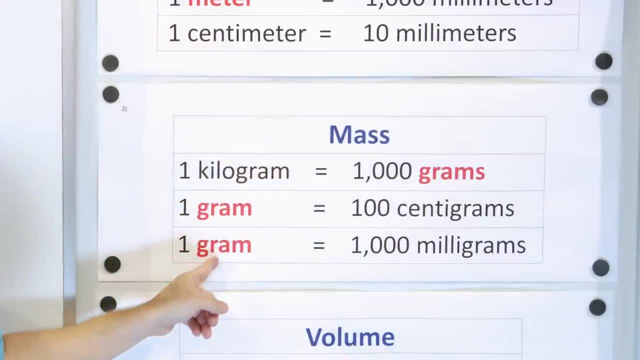 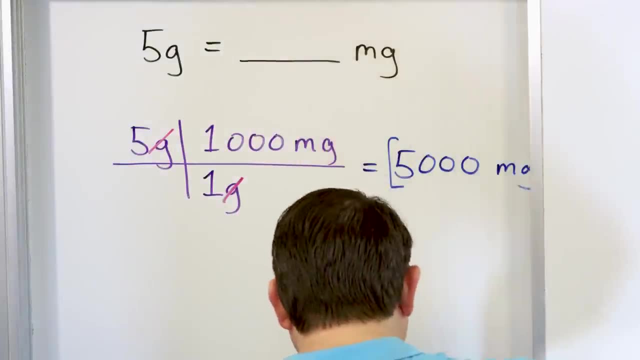 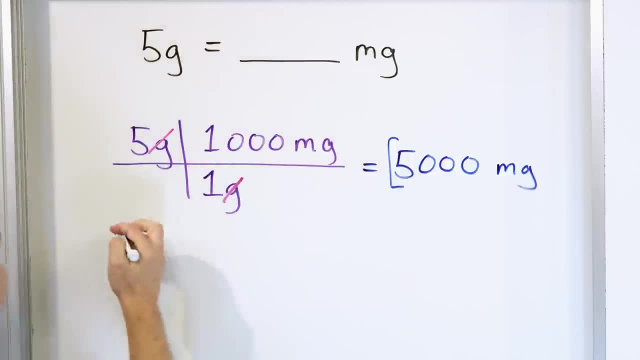 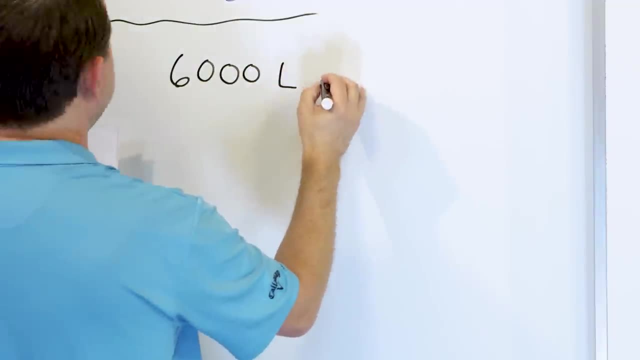 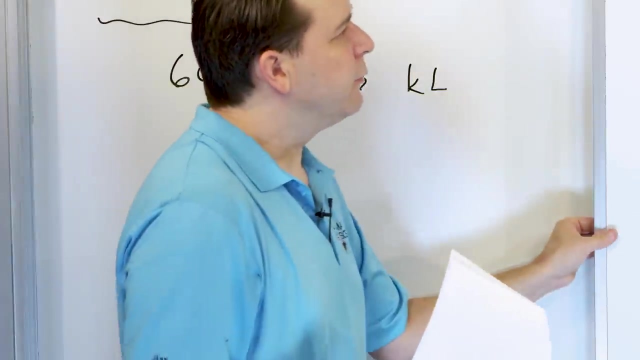 talking, but here in the beginning I just want to make sure everybody's on the same page. Next problem: let's say I have 6,000 liters and I want to convert that to kiloliters, So I need to go between liters and kiloliters. So let's go back to our chart and think about: 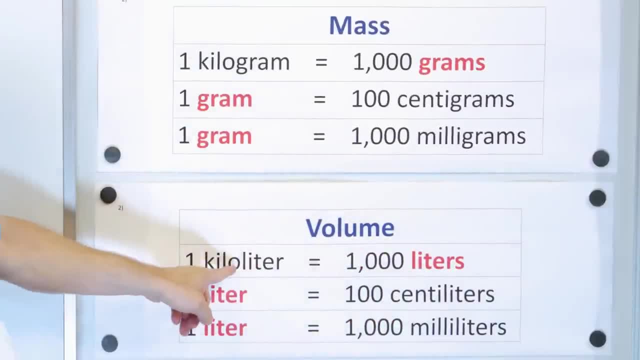 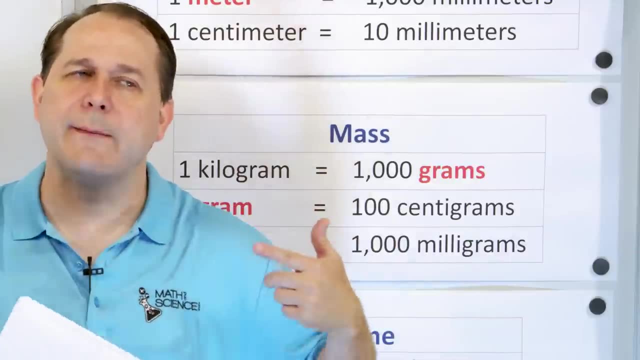 it. We're looking at liters and we're looking at liters and kiloliters. Now this is telling us that one kiloliter is the same as 1,000 liters. Now I'm using my chart, but actually, once I start learning them, I don't really need the chart, because I know that kilo means. 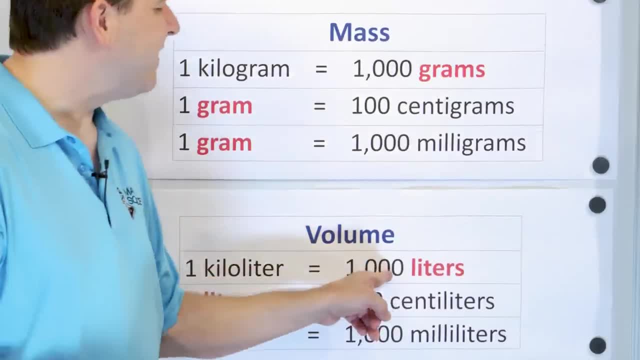 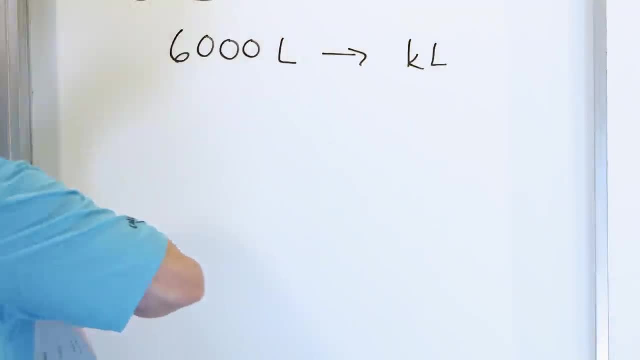 1,000 times bigger. So one kiloliter must be 1,000 of these liters. So one kiloliter is 1,000 liters. Now how do I arrange it? I first write down what I know: 6,000 liters. 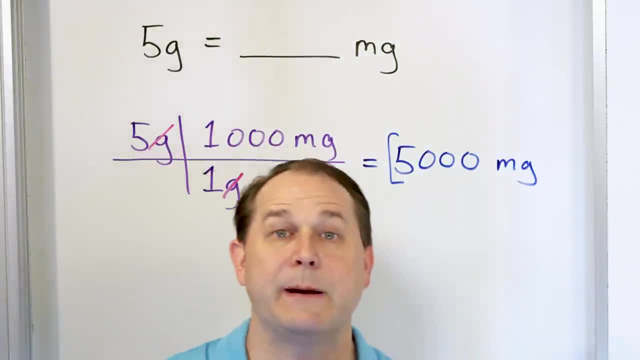 and do it all, but I'm trying to also show you how to multiply and divide by powers of 10.. When you multiply by a power of 10,, meaning you multiply by 10, or 100, or 1,000,. 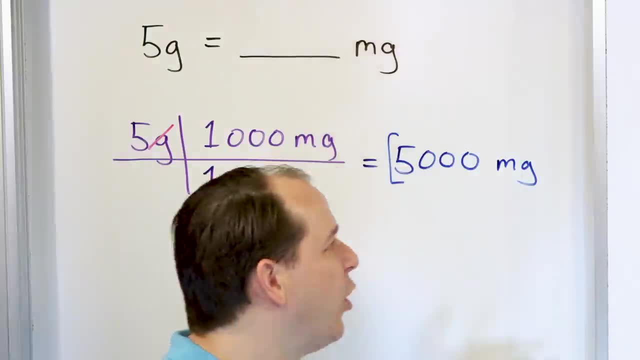 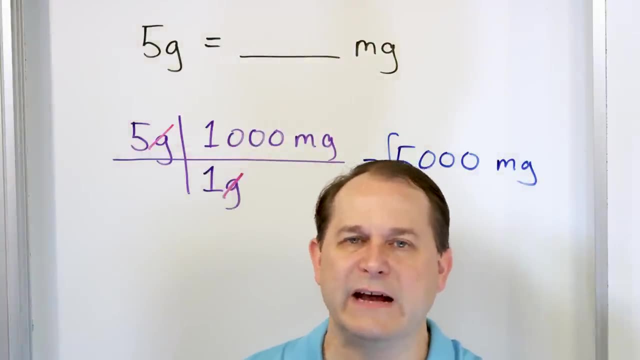 or 10,000, or 100,000,, then it's very easy, because all you do is ignore the zeros. Five times one is five, and then you add the zeros back in. So when you multiply by powers of 10, it's very simple. 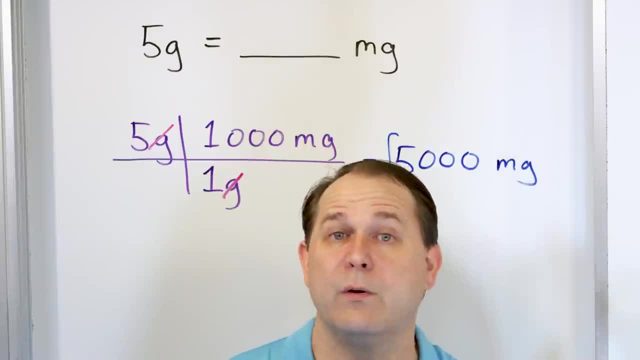 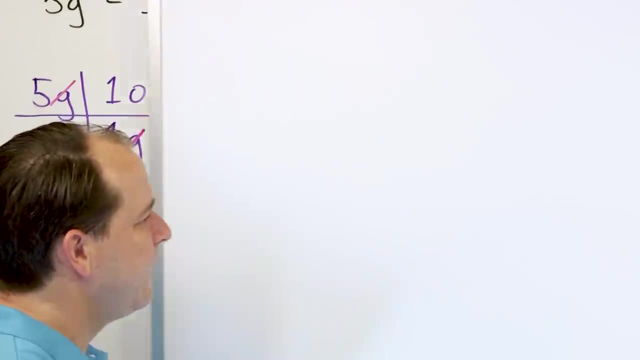 You just add the zeros at the end When you divide by powers of 10, we'll see what we do here in just a minute. But for here we are telling ourselves that five grams is 5,000 milligrams. Does that make sense? 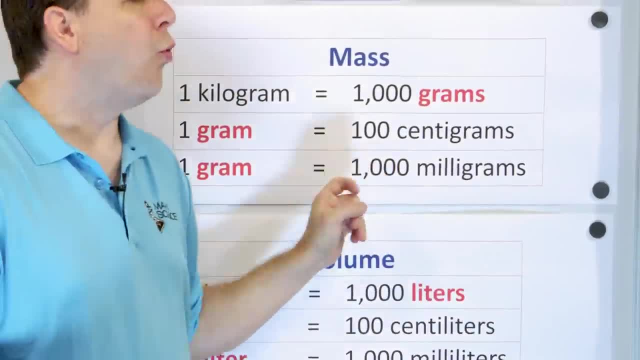 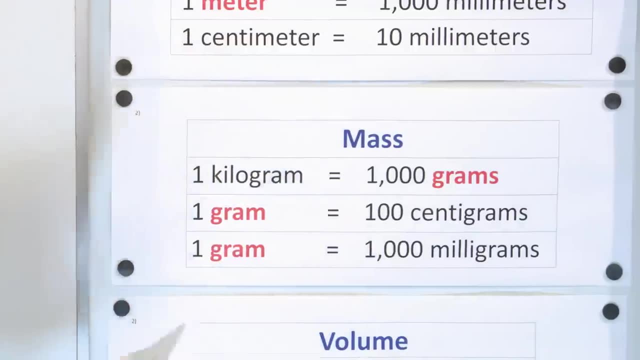 Well, I know here that one gram is the same as 1,000 milligrams. So if I have five of these grams, I must have 5,000 of these milligrams, And that is the final answer As we go through these problems. 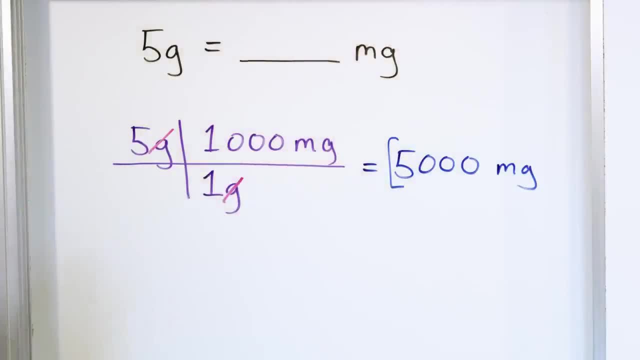 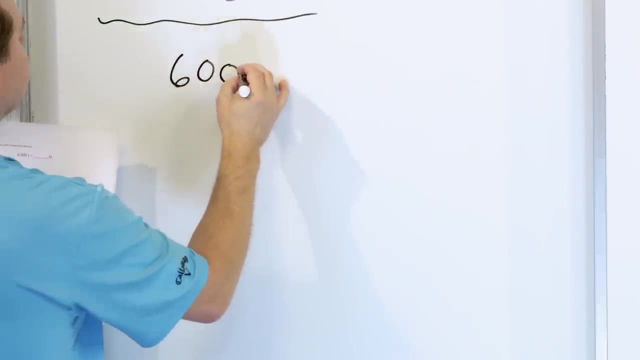 I'll be able to do less and less and less talking, But here in the beginning I just want to make sure everybody's on the same page. Next problem: Let's say I have 6,000 liters and I want to convert that to kiloliters. 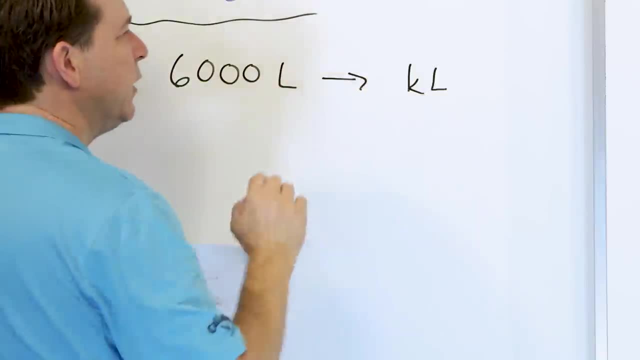 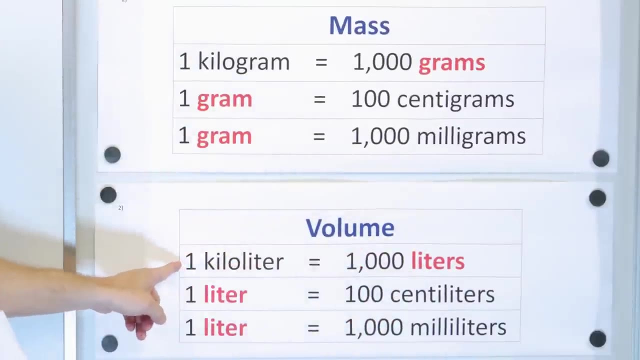 Kiloliters. So I need to go between liters and kiloliters. So let's go back to our chart and think about it. We're looking at liters and we're looking at liters and kiloliters. Now this is telling us that one kiloliter 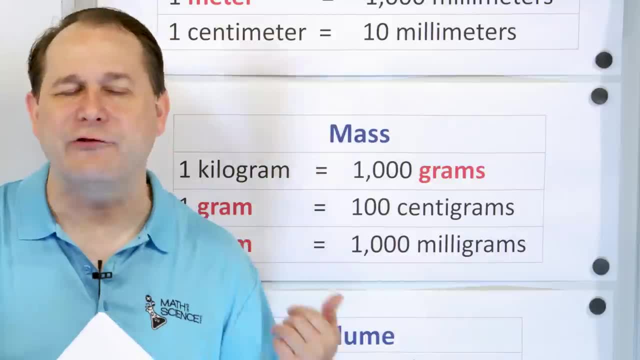 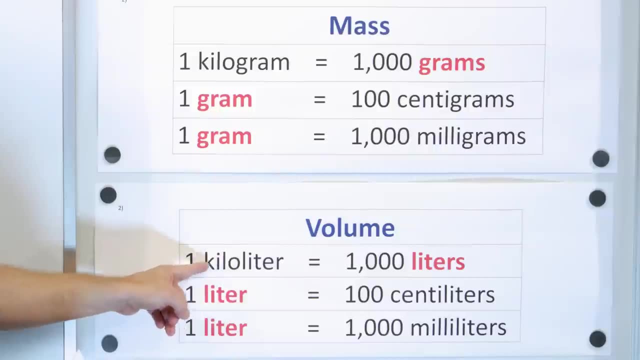 is the same as 1,000 milligrams. Now I'm using my chart, but actually once I start learning them, I don't really need the chart, because I know that kilo means 1,000 times bigger. So one kiloliter must be 1,000 of these liters. 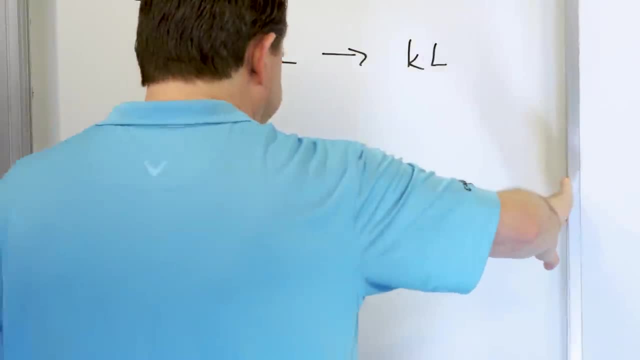 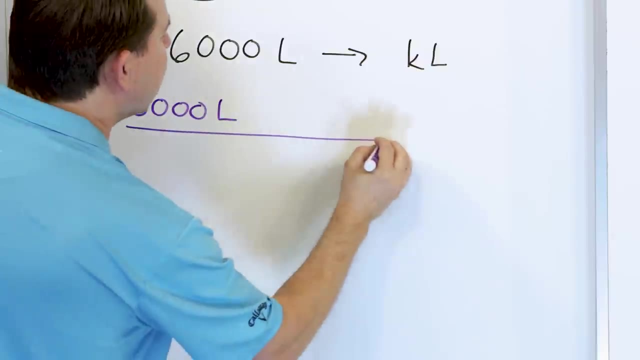 So one kiloliter is 1,000 liters. Now how do I arrange it? I first write down what I know- 6,000 liters- draw a horizontal line and then draw a vertical line. Now I know that one kiloliter is 1,000 liters. 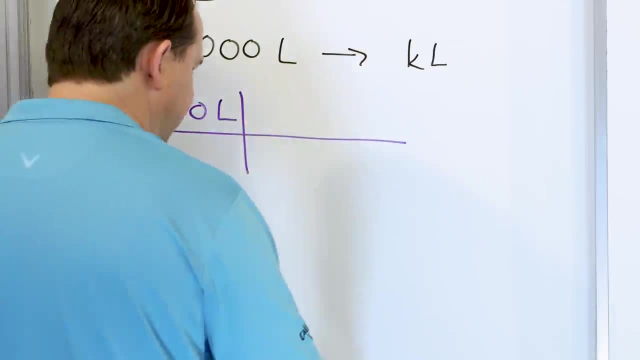 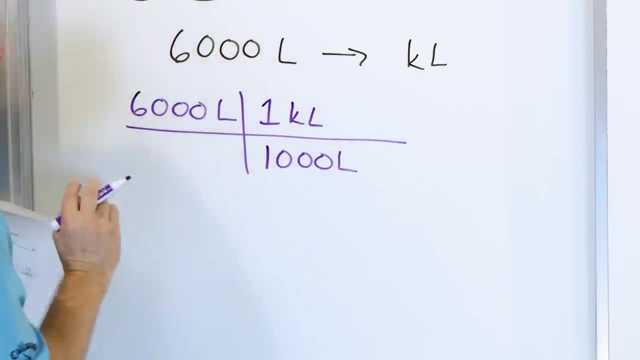 Now I could put the kiloliters: the kiloliter on the top or the kiloliter on the bottom. The way that you need to write it is that one kiloliter is 1,000 liters. Why do I write it this way? 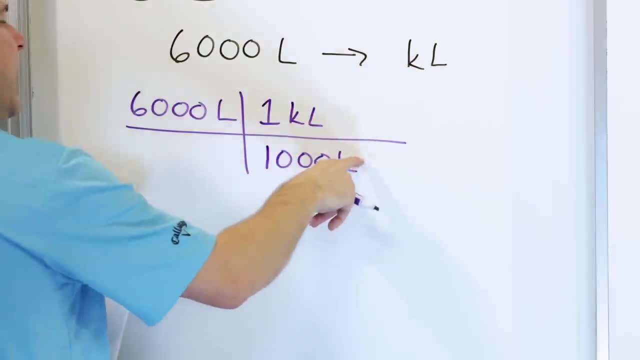 I could flip it over and have the kiloliters on the bottom and then the 1,000 liters on the top. but if I do that, nothing will cancel. You see, it only cancels if I have something on the top. 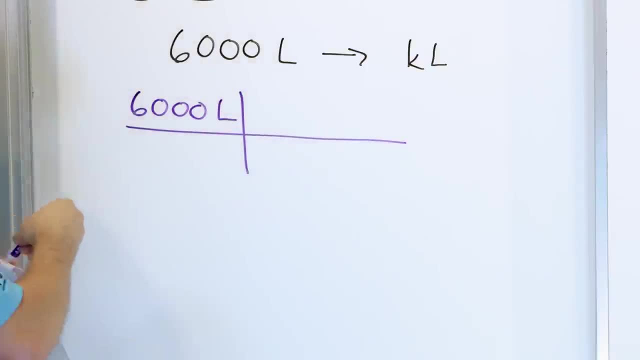 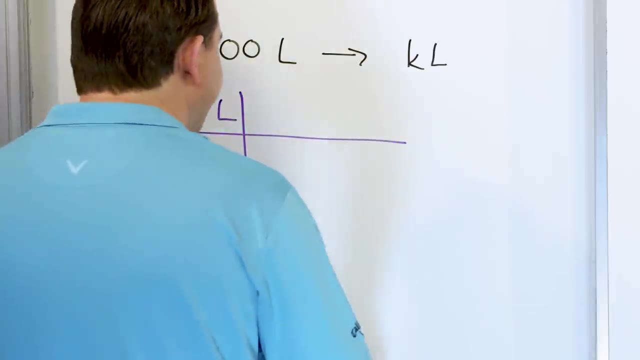 draw a horizontal line and then draw a vertical line. Now I know that one kiloliter is 1,000 liters. Now I could put the kiloliter on the top or the kiloliter on the bottom. Okay, The way that you need to write it is that one kiloliter is 1,000 liters. Why do I write? 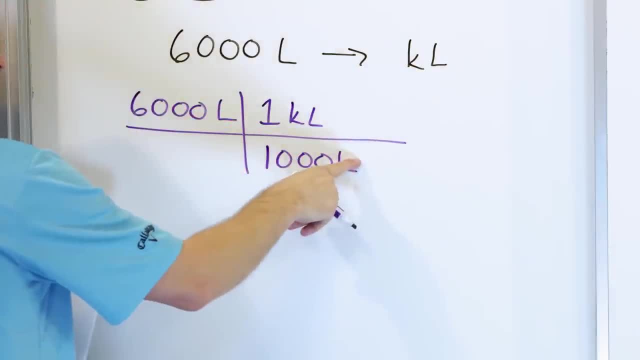 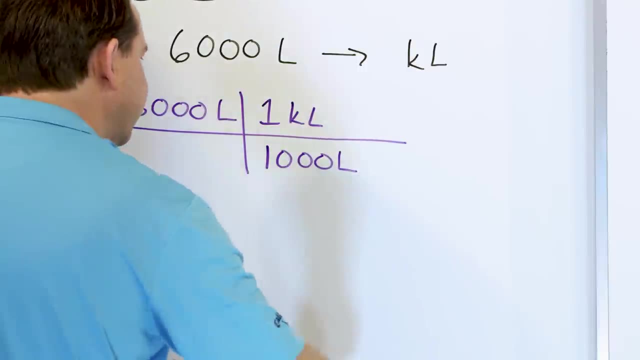 it this way: I could flip it over and have the kiloliters on the bottom and then the 1,000 liters on the top. But if I do that, nothing will cancel. You see, it only cancels if I have something on the top and something on the bottom. Liters will cancel with liters. 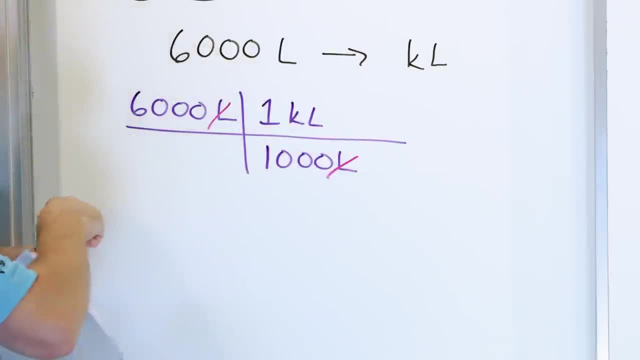 If I flipped it over, nothing would cancel. I would have kiloliters here, and that would be wrong. So what is this telling me that I need to do? It's telling me that what I need to do is take 6,000 and multiply by 1. Everything on the top gets multiplied Once. 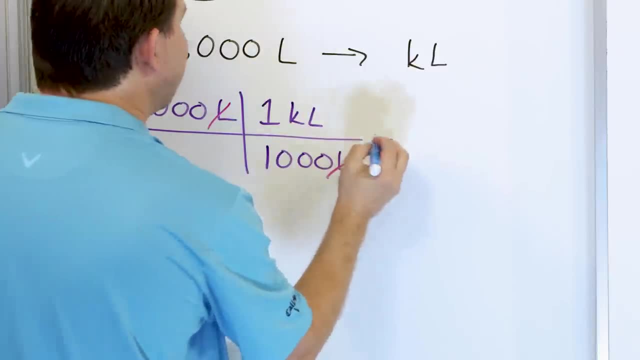 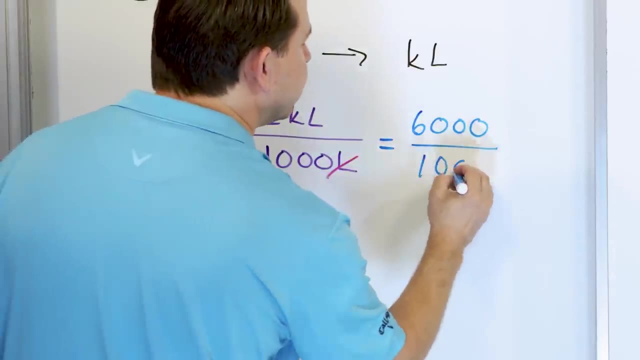 I do that, then I divide by everything on the bottom. So what am I going to actually have? 6,000 times 1? on the top is 6,000.. And then on the bottom I still have to divide by 1,000.. 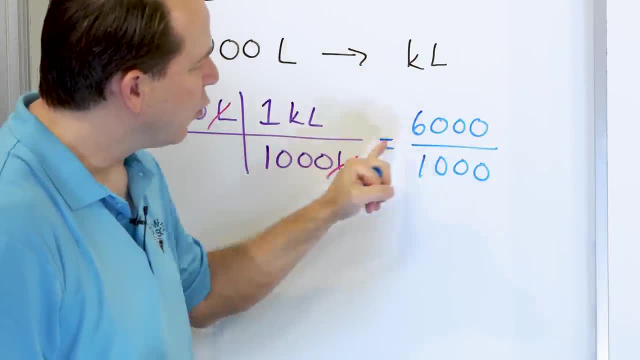 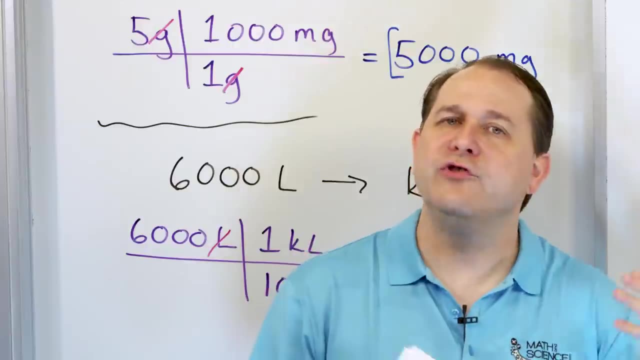 So here I have kind of a fraction: 6,000 over or divided by 1,000.. So you can do the long division. You can write down 6,000, put your division house, divide by 1,000. You can do. 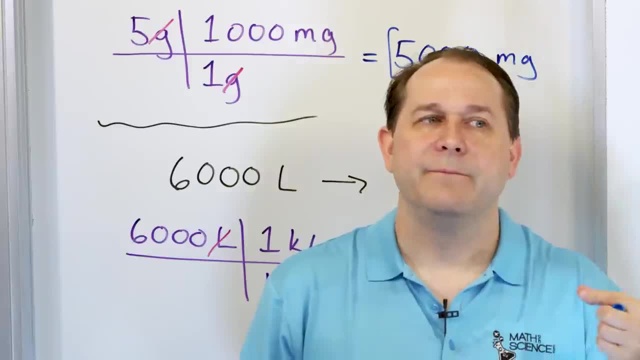 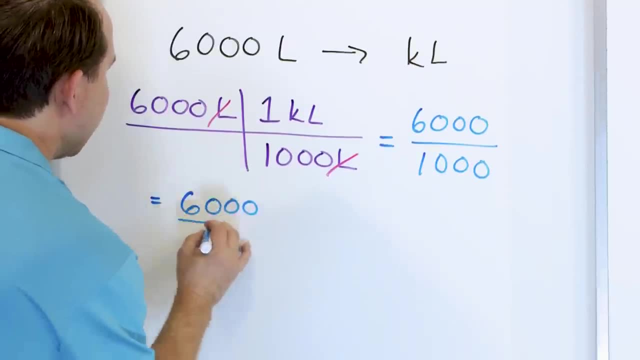 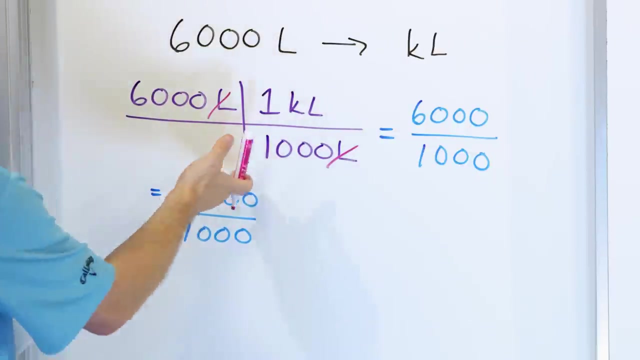 all that, Or you can listen to what I'm telling you about multiplying and dividing by powers of 10. Because here I have 6,000 on the top and I have 1,000 on the bottom, And when you're dividing numbers like this, if I have something on the top and the bottom I can cancel. So 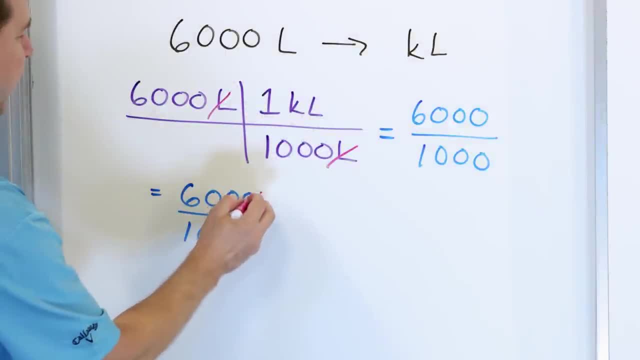 anytime you have zeros in the top and zeros in the bottom, I can cancel this zero with this one. This zero will cancel with this one. This zero will cancel with this one. What will I actually have left? I will have a 6 on the top and divided by a 1 on the bottom. 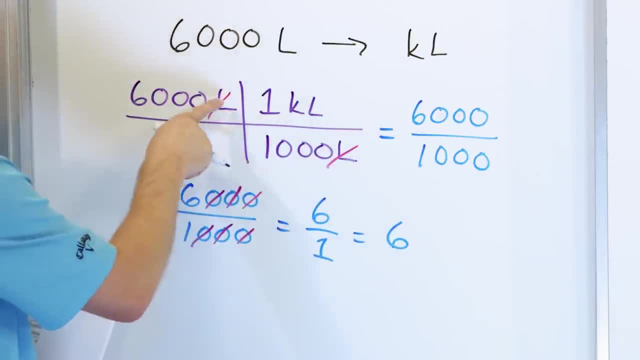 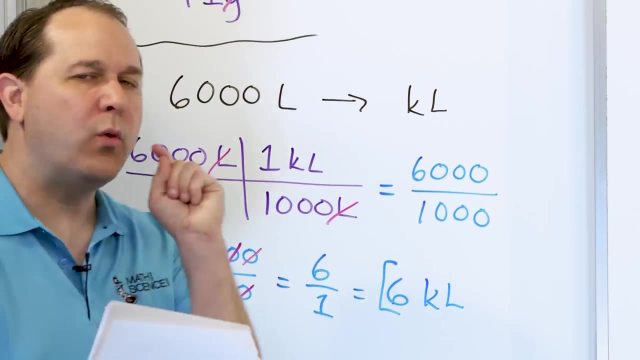 And so the answer will be 6.. And the only unit I have left, because the liters cancel with the liters- is kiloliters. Now let's see if this makes sense. We know that 1 kiloliter is 1,000 liters, So if I 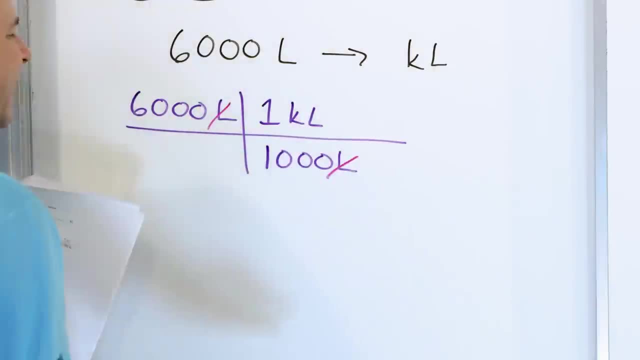 and something on the bottom: Liters will cancel with liters. If I flipped it over, nothing would cancel. I would have kiloliters here and that would be wrong. So what is this telling me that I need to do? It's telling me that what I need to do is take 6,000. 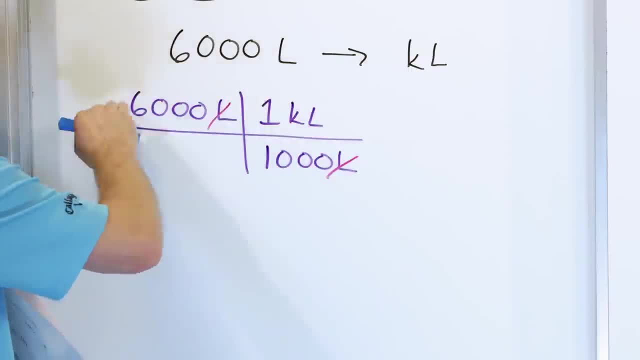 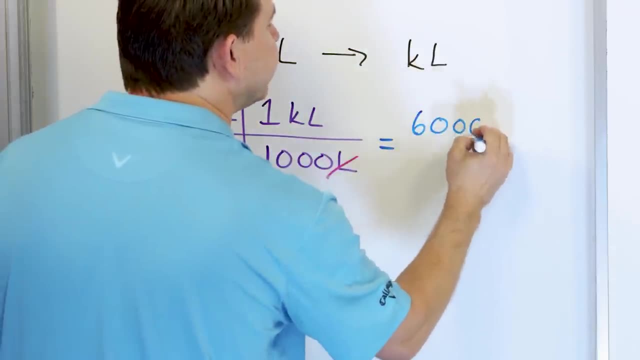 and multiply by 1.. Everything on the top gets multiplied Once I do that, then I divide by everything on the bottom. So what am I going to actually have? 6,000 times 1 on the top is 6,000,. 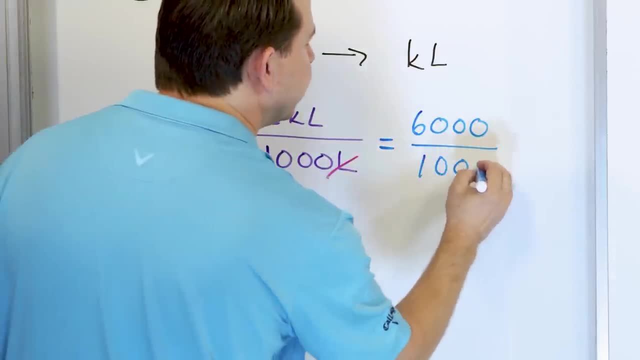 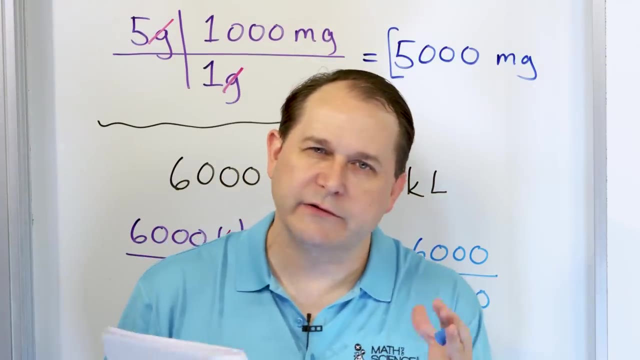 and then on the bottom I still have to divide by 1,000. So here I have kind of a fraction, 6,000 over or divided by 1,000. So you can do the long division, You can write down 6,000, put your division house. 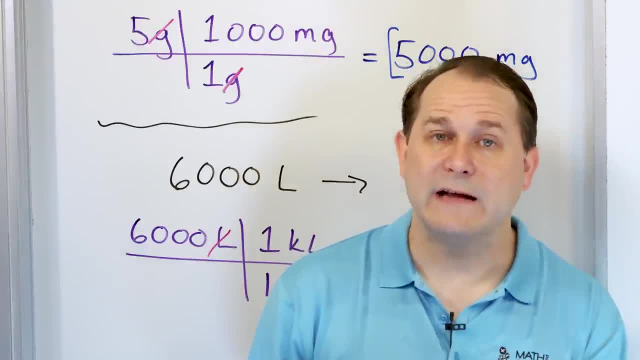 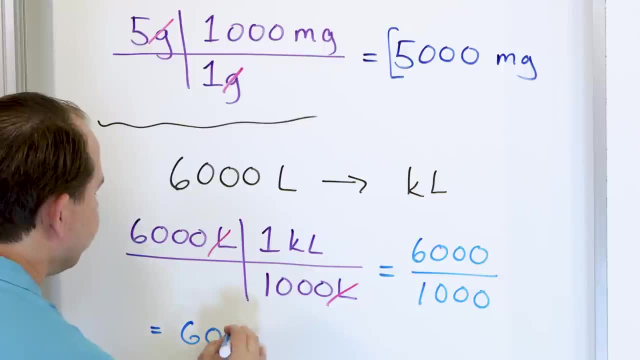 divide by 1,000, you can do all that, Or you can listen to what I'm telling you about multiplying and dividing by powers of 10. Because here I have 6,000 on the top and I have 1,000 on the bottom. 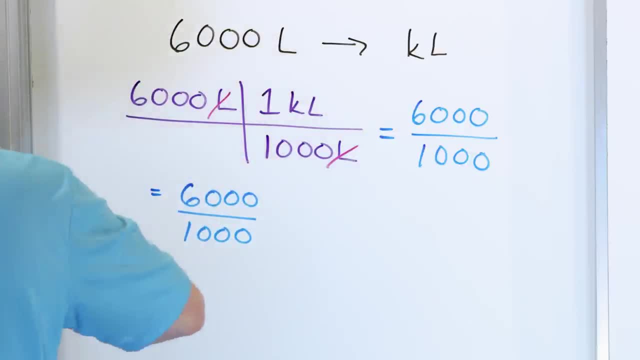 And when you're dividing numbers like this, if I have something on the top and the bottom, I can cancel. So anytime you have zeros in the top and zeros in the bottom, I can cancel this zero with this one. this zero will cancel with this one. 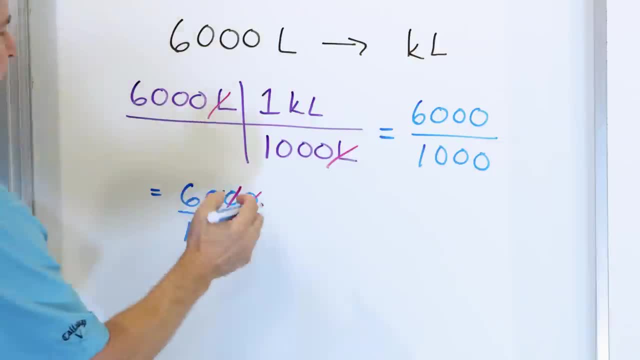 this zero will cancel with this one, And what will I actually have left? I will have a six on the top and divided by a one on the bottom, And so the answer will be six, and the only unit I have left- because the liters cancel with the liters- is kiloliters. 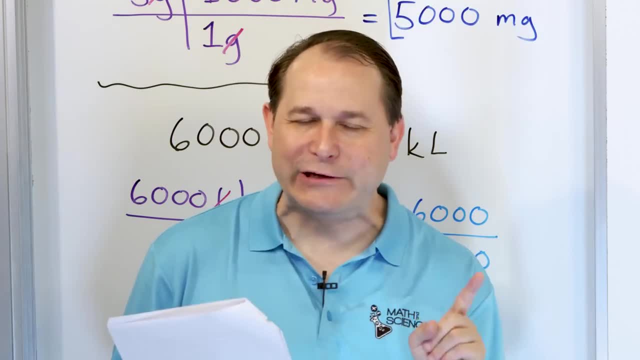 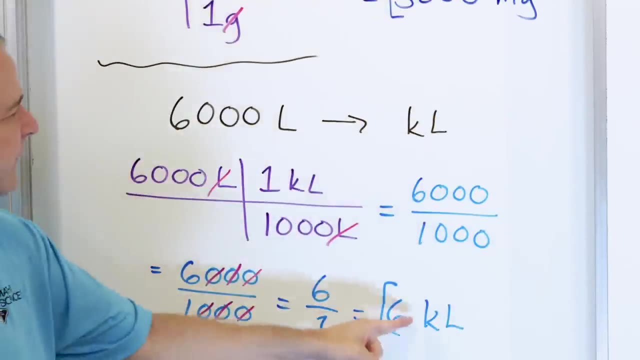 Now let's see if this makes sense. We know that one kiloliter is 1,000 liters, So if I were to have six of these kiloliters, it should be 6,000 liters, And so this unit conversion makes sense. 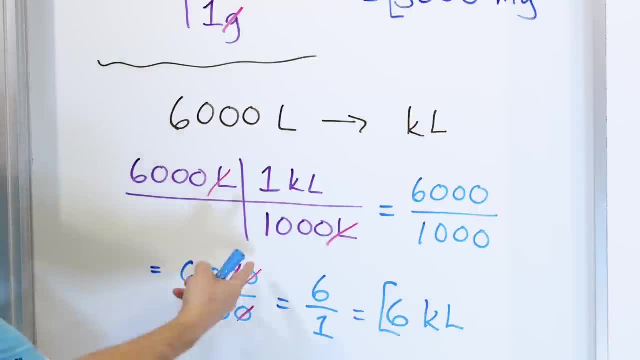 Now, before I go to the next problem, I want to explain why this is okay. Why can we strike zeros like this? The reason is because this is a fraction. It's division, but we're writing it as a fraction: 6,000 divided by 1,000, or 6,000 over 1,000.. 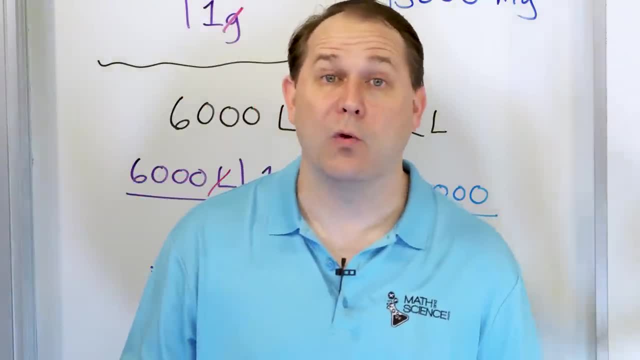 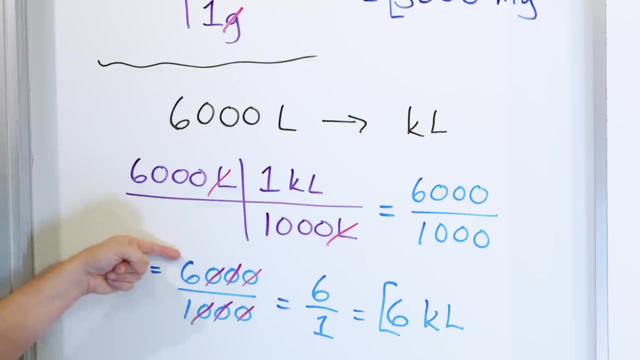 I can simplify fractions by dividing top and bottom by anything I want. So if I take this top and divide by 1,000, and then take this bottom and divide it also by 1,000, 6,000 divided by 1,000 is six. 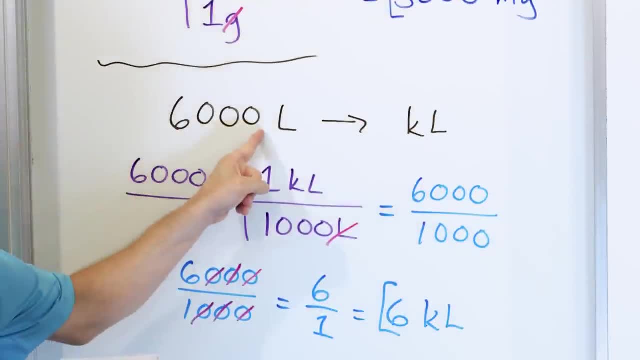 were to have 6 of these kiloliters, it should be 6,000 liters, And so this unit conversion makes sense. Now, before I go to the next problem, I want to explain why this is okay. Why can we strike zeros like this? The reason is because this is a fraction, It's division, but we're 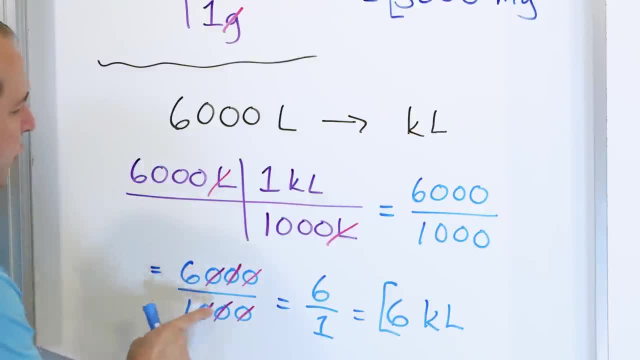 writing it as a fraction: 6,000 divided by 1,000 or 6,000 over 1,000.. I can simplify fractions by dividing top and bottom by anything I want. So if I take this top and divide by 1,000 and then take this bottom and divide it also by 1,000, 6,000 divided by 1,000 is. 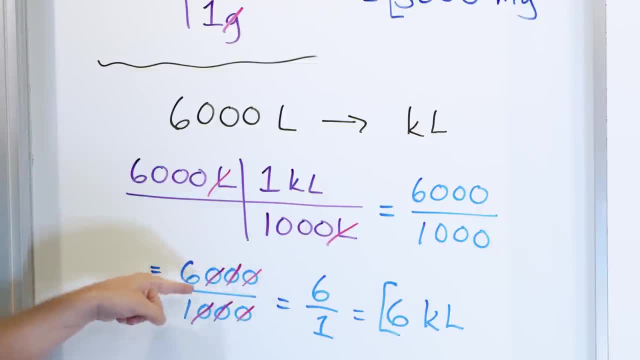 6. 1,000 divided by 1,000 is 1.. So striking the zeros is the same thing as simplifying fraction. Divide by 1,000, divide by 1,000.. And you can certainly do it that way if you. 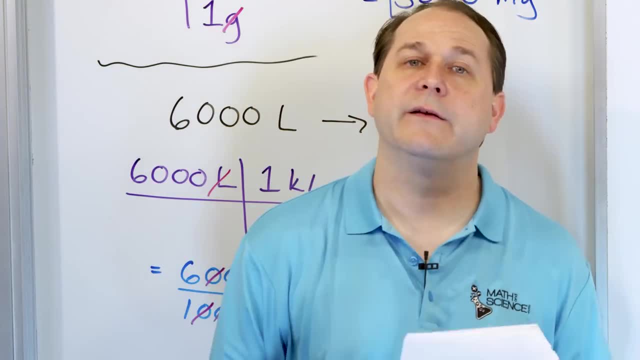 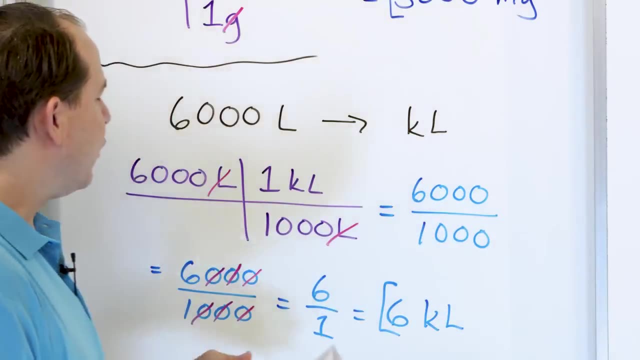 want. But I'm trying to teach you to strike through the zeros because we're going to be doing that a lot more when we get into algebra and pre-algebra and other parts of math later. So that is in a nutshell why unit conversions of metric system is so easy, Why the metric 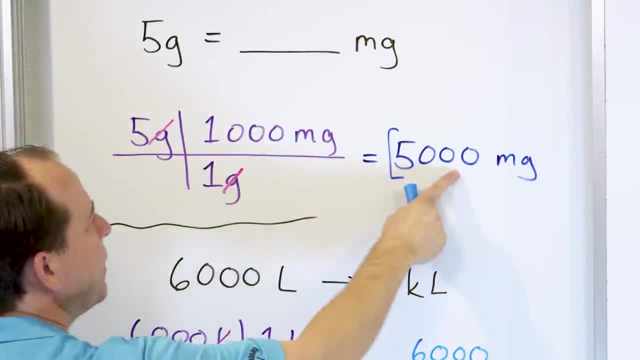 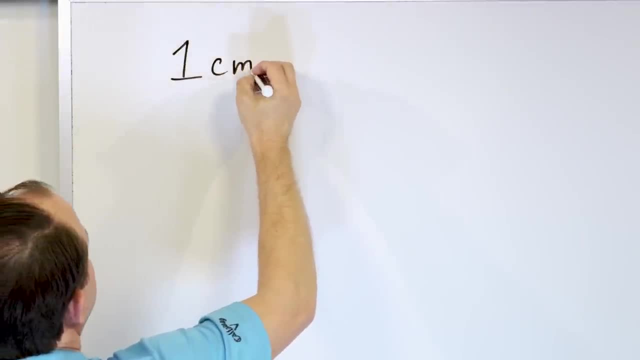 system is so much better Because when I multiply this, it's very easy to multiply. When I divide these, it's very easy to divide. All right, Let's take a look at the next problem. 1 centimeter is equal to: or. let's convert. 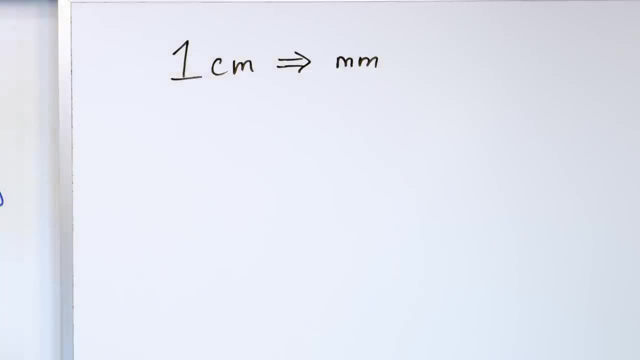 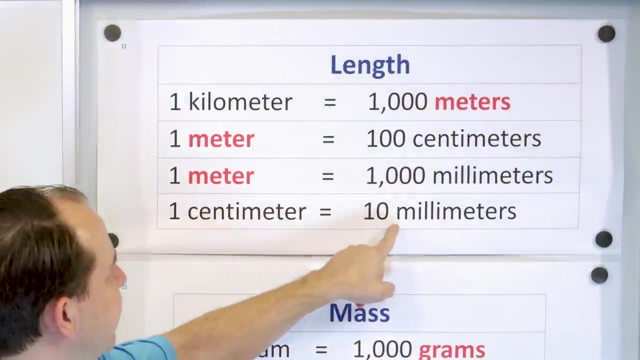 1 centimeter into how much? 1 centimeter? How many millimeters? right, 1 centimeter. We're going to go from centimeter to millimeter. Now, actually, if you look at our chart, I already wrote down that 1 centimeter is 10. 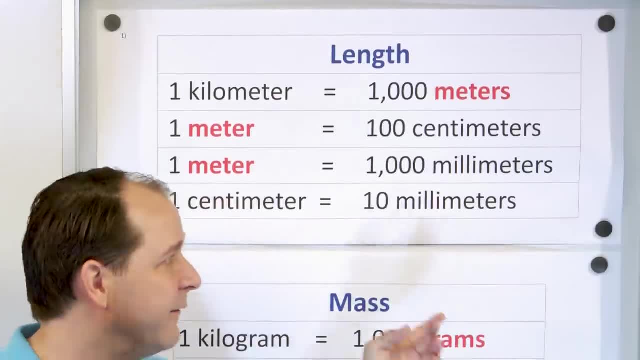 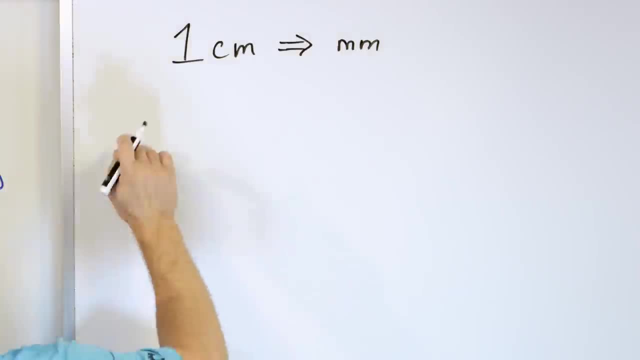 millimeters. So we already know the answer. What we want to do is prove to ourselves that this is true, So let's go ahead and do that here. What we have is: we can write down what we are given. We have 1 centimeter, And what we want to do is try to find a conversion. 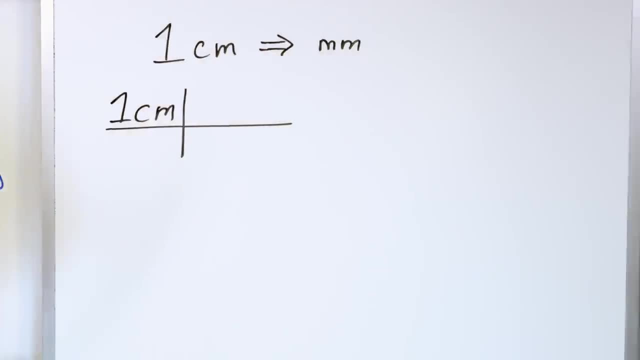 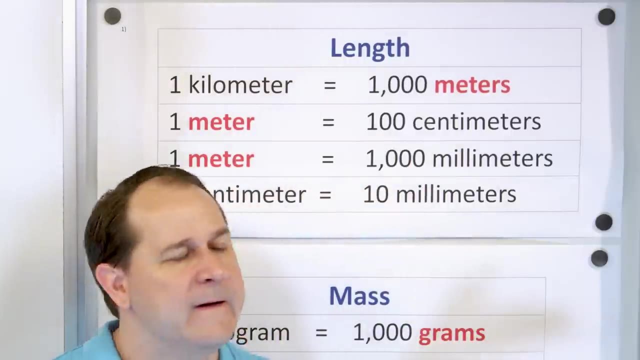 factor that goes from centimeters to millimeters. Now here we actually already have it, We already have the answer. We know that this is the answer, But we want to show and prove to ourselves without using that. So instead of going straight from centimeters to millimeters, is there any other way I could? 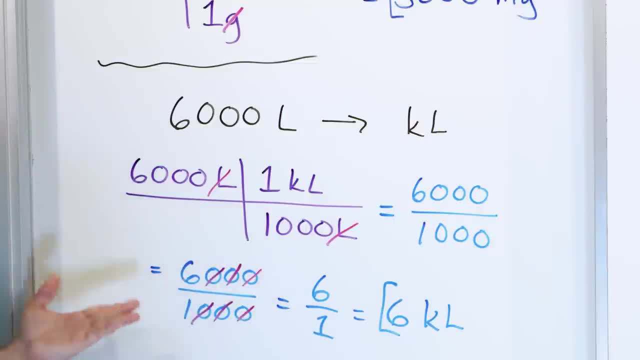 1,000 divided by 1,000 is one. So striking the zeros is the same thing as simplifying fraction: divide by 1,000, divide by 1,000. And you can certainly do it that way if you want. 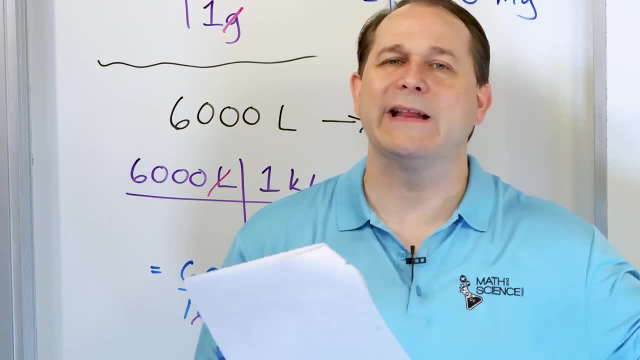 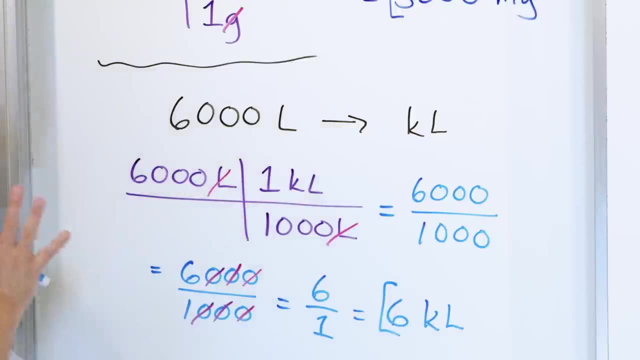 but I'm trying to teach you to strike through the zeros because we're going to be doing that a lot more when we get into algebra and pre-algebra and other parts of math later. So that is in a nutshell why unit conversions of metric system is so easy. 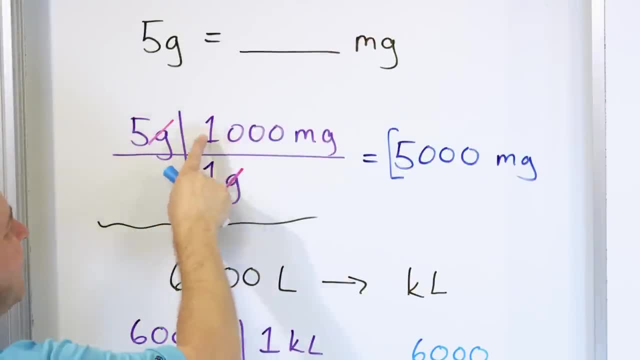 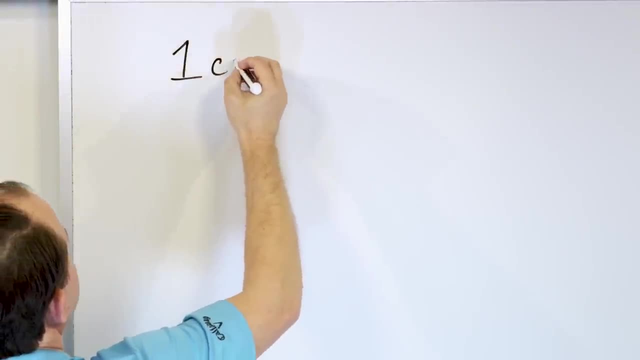 Why the metric system is so much better? because when I multiply this, it's very easy to multiply. When I divide these, it's very easy to divide. All right, let's take a look at the next problem. One centimeter is equal to. 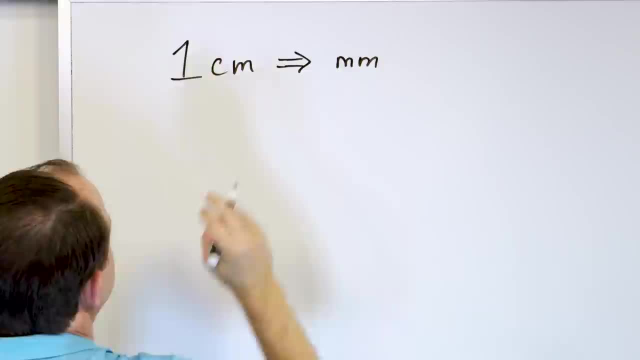 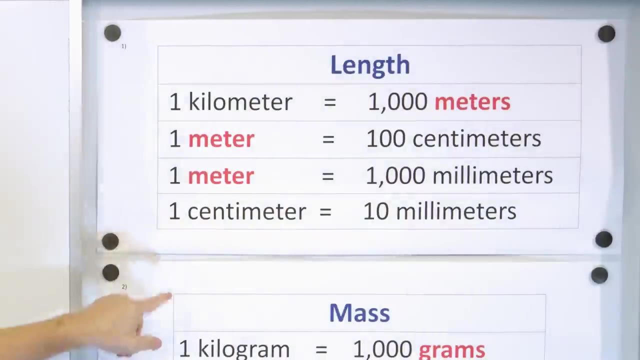 or let's convert one centimeter into how many millimeters? right, One centimeter. we're going from centimeter to millimeter. Now, actually, if you look at our chart, I already wrote down that one centimeter is 10 millimeters. 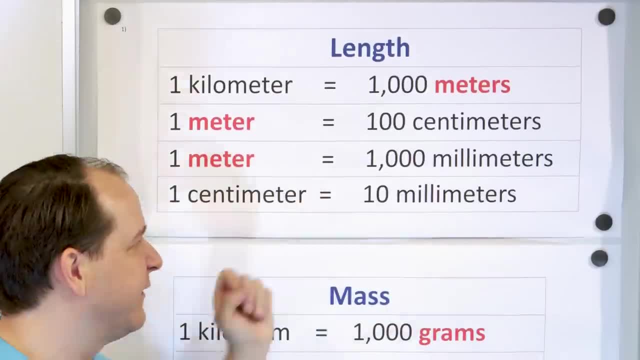 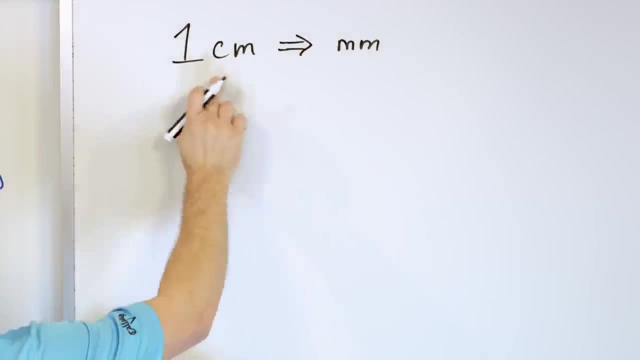 So we already know the answer. What we want to do is prove to ourselves that this is true, So let's go ahead and do that here. What we have is: we can write down what we are given. We have one centimeter, And what we want to do is try to find a conversion factor. 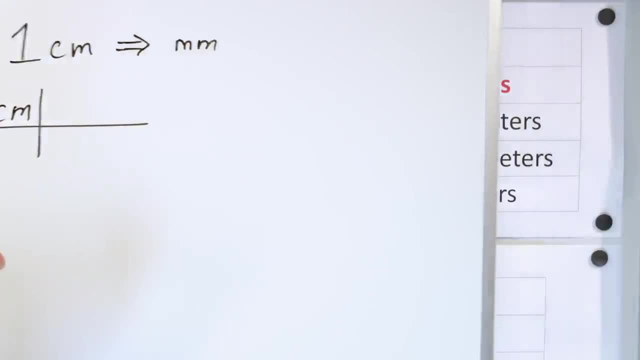 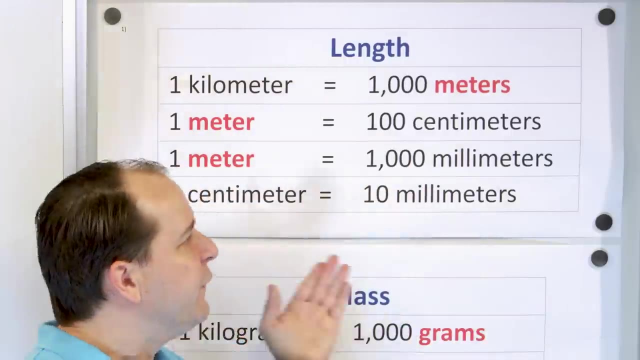 that goes from centimeters to millimeters. Now here we actually already have it. We already have the answer. We know that this is the answer, but we want to show and prove to ourselves without using that. So instead of going straight from centimeters to millimeters, 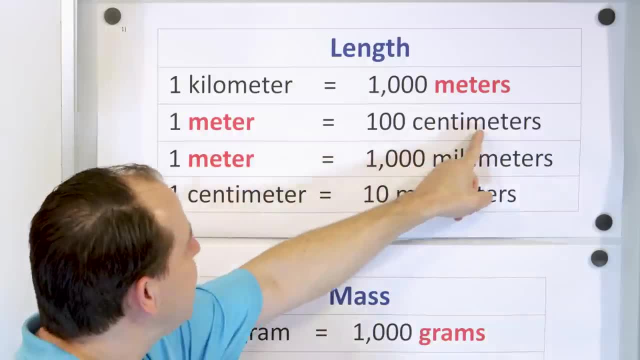 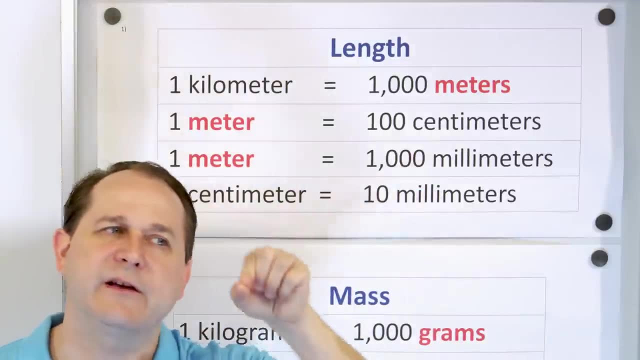 is there any other way I could get to the answer? Well, I could go from centimeters to meters and then, once I'm at meters, I could go from meters to millimeters. So you can do these conversion steps in jumps. All you have to do is jump through the tables. 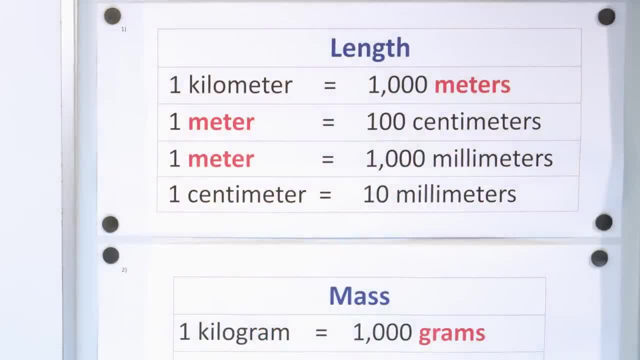 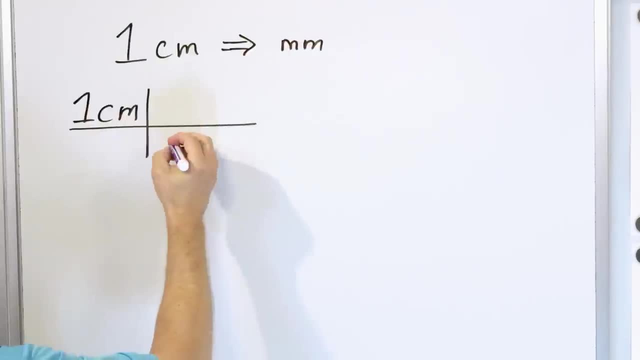 from one unit to another, All right. So if I want to go from centimeters to meters, I know that there's 100 of these centimeters in one meter, So I'm gonna write it down like this: One. I'm sorry, 100 of these centimeters. 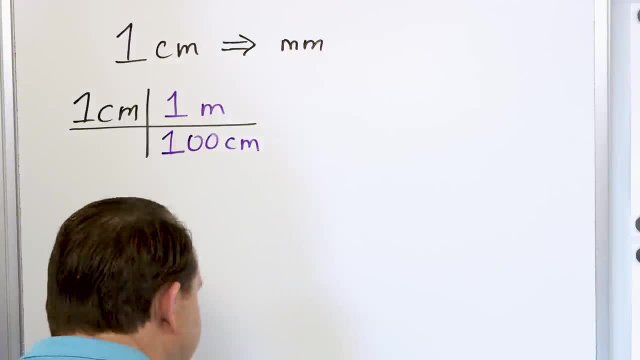 are in one of these meters. Now, why am I writing it down this way? Because if I flip it over with centimeters on the top and meters on the bottom, nothing will cancel. But this way the centimeters here will cancel with the centimeters there. 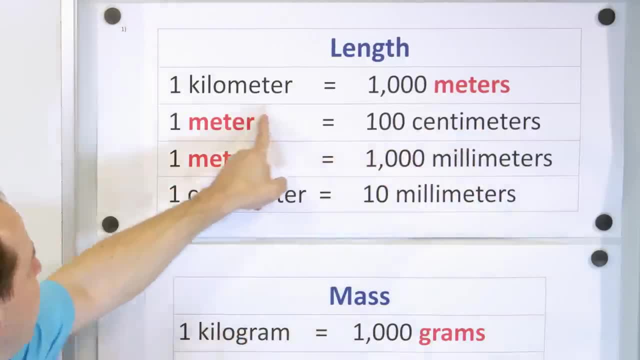 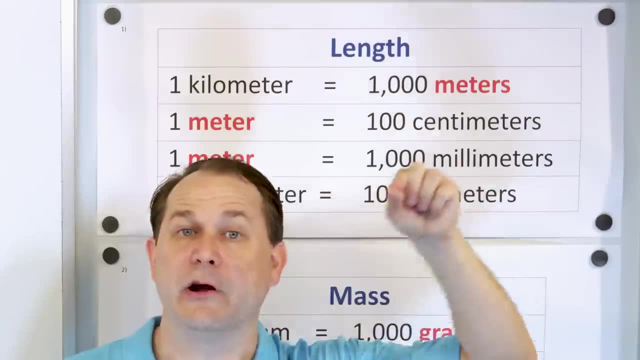 get to the answer. Well, I could go from centimeters to meters And then, once I'm at meters, I could go from meters to millimeters. So you can do these conversion steps in jumps. All you have to do is jump through the tables from one unit to another. 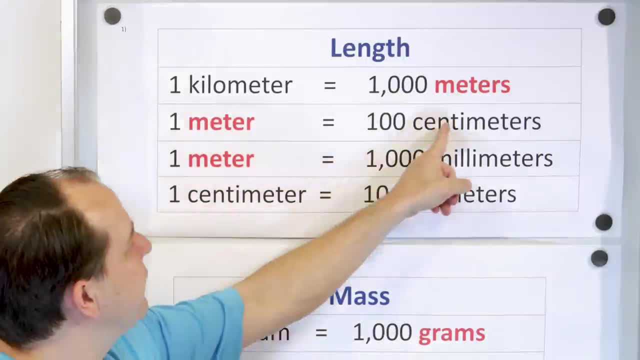 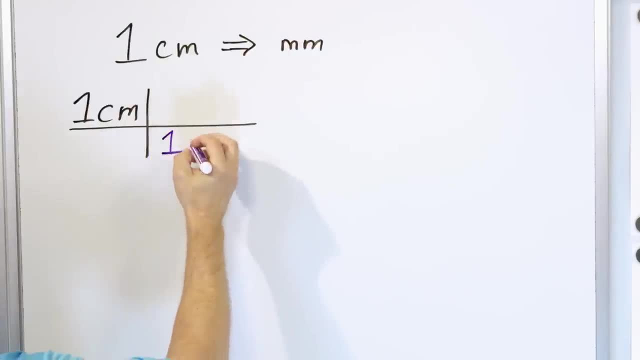 All right. So if I want to go from centimeters to meters, I know that there's 100 of these centimeters in one meter, So I'm going to write it down like this: One, I'm sorry, 100 of these centimeters. 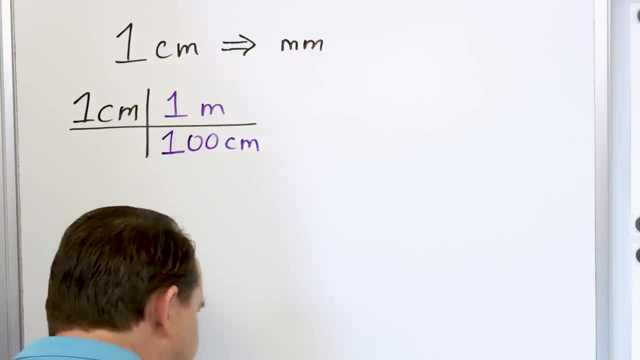 are in one of these meters. Now, why am I writing it down this way? Because if I flip it over with centimeters on the top and meters on the bottom, nothing will cancel. But this way the centimeters here will cancel with the centimeters there. Now, if I stop the, 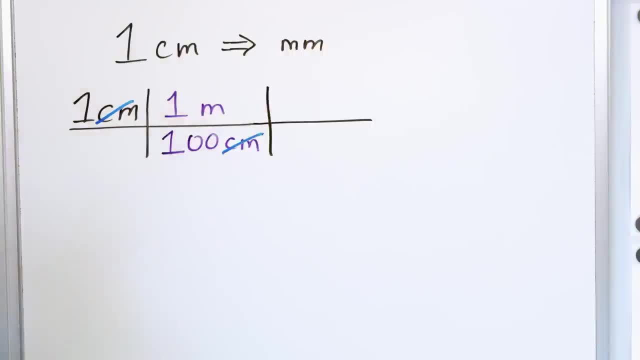 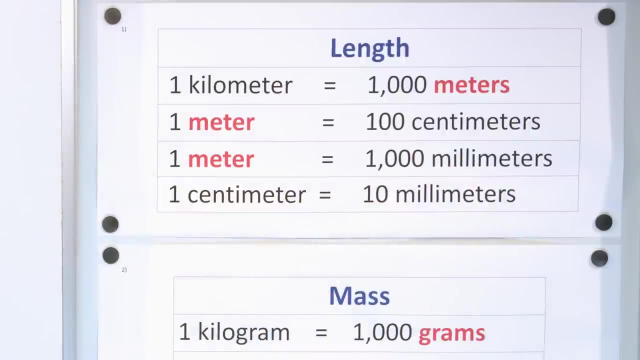 conversion here. if I just do the calculation, I'm going to end up here. I'm going to end up in meters. But I don't want to go to meters, I want to go to millimeters. I know that one meter is 1,000 of these little bitty millimetres. I have to put the one meter on the bottom. 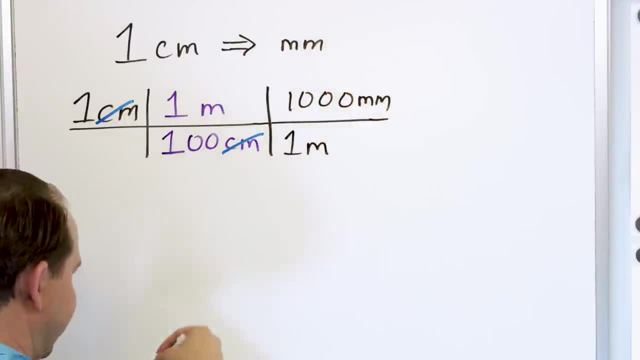 and 1,000 millimeters on the top. Why am I writing it this way? Because if I write it this way, I have this meters canceling. with this meter, If I flip it over with 1,000 millimeters on the bottom, nothing will cancel. So this is the only way to make sure that everything. 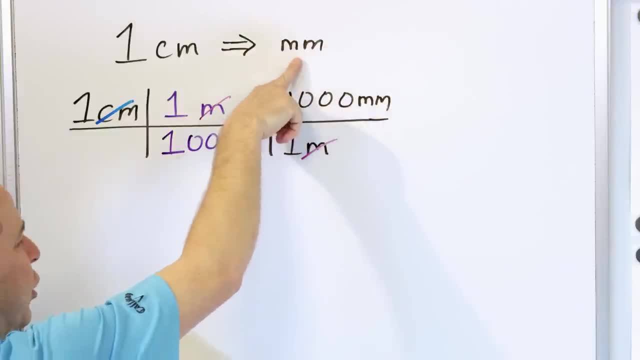 cancels, and all I have left is millimeters. That's where I want to go. Now how do I figure out the answer? I have to multiply everything on the top and then divide by everything on the bottom. So here I have: 1 times 1 is 1.. And then 1 times 1,000. 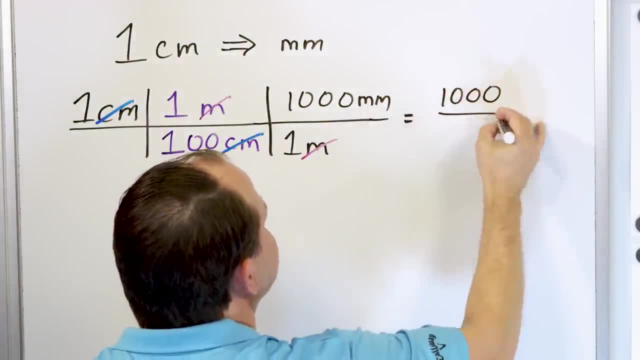 on the top will be what? 1,000. So I'll have 1,000 on the top And on the bottom I'll have 100.. I have to multiply everything on the bottom: 100 times 1 is 100. So what? I? 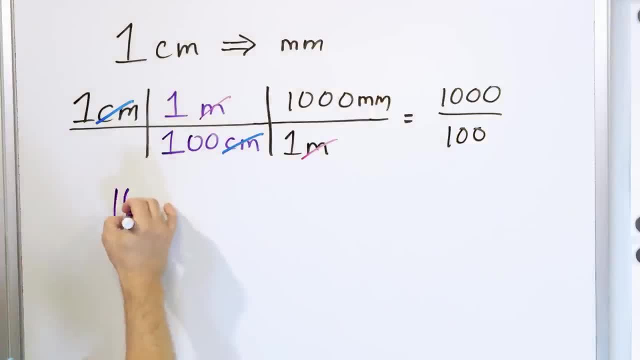 have is 1,000 on the top and 100 on the bottom. So 1,000 on the top and 100 on the bottom. Remember I told you the same thing. If you have trailing zeros like this, this zero can cancel with this one. This zero can cancel with this one. The answer that I get on the 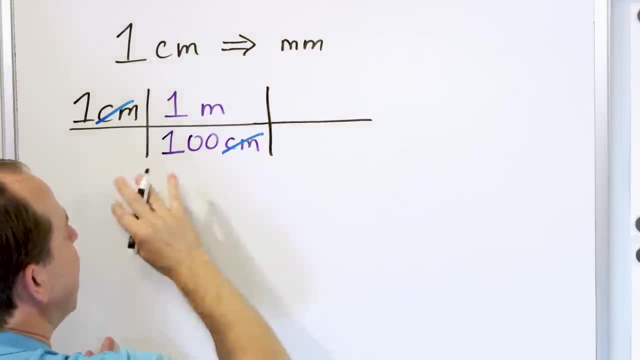 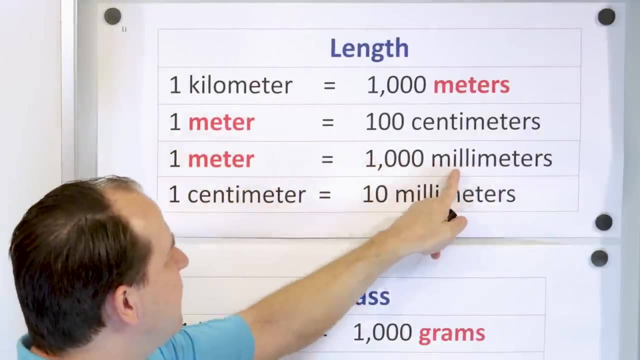 Now, if I stop the conversion here, if I just do the calculation, I'm gonna end up in meters. But I don't want to go to meters, I want to go to millimeters. I know that one meter is 1,000. 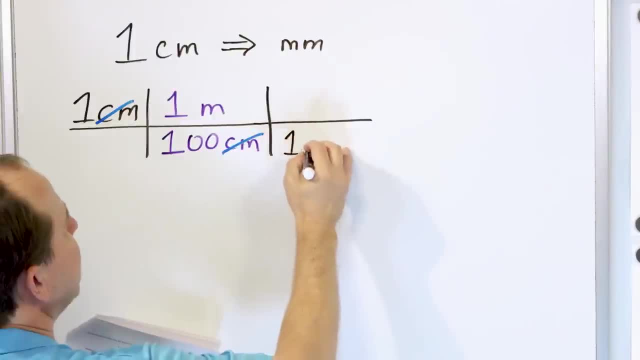 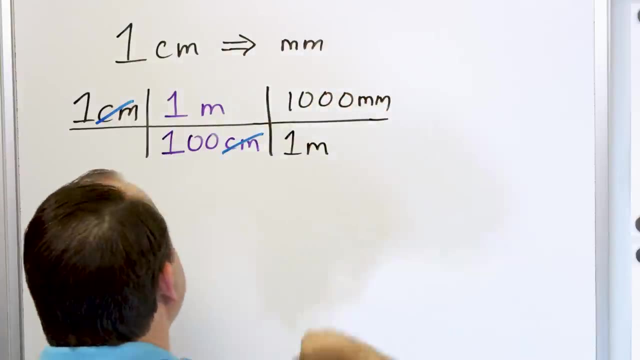 of these little bitty mill-a-meters. I have to put the one meter on the bottom and 1,000 millimeters on the top. Why am I writing it this way? Because if I write it this way, I have this meters canceling with this meter. 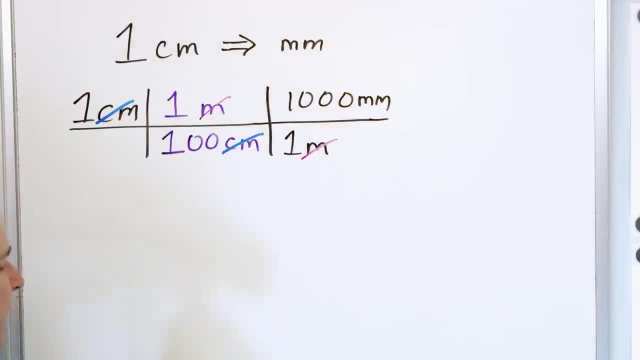 If I flip it over with 1,000 millimeters on the bottom, nothing will cancel. So this is the only way to make sure that everything cancels, and all I have left is meters. that's where I want to go Now how do I figure out the answer? I have to multiply. 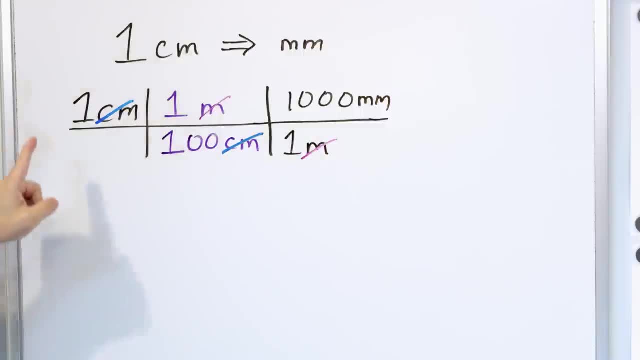 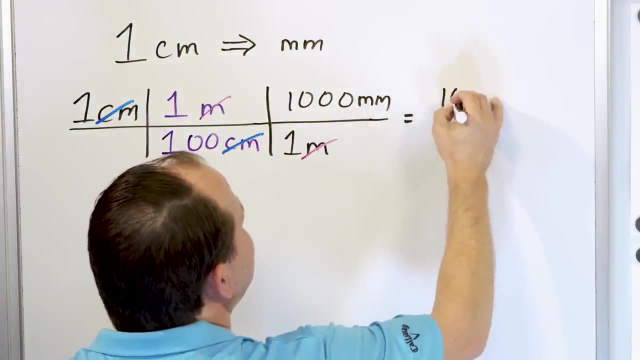 everything on the top and then divide by everything on the bottom. So here I have: 1 times 1 is 1, and then 1 times 1,000 on the top will be what 1,000.. So I'll have 1,000 on the top and on the bottom I'll have 100.. I have to multiply everything. 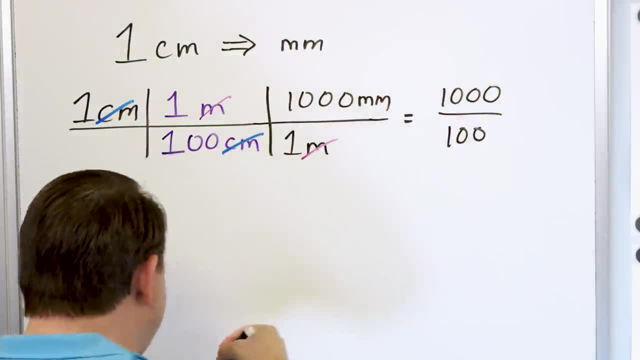 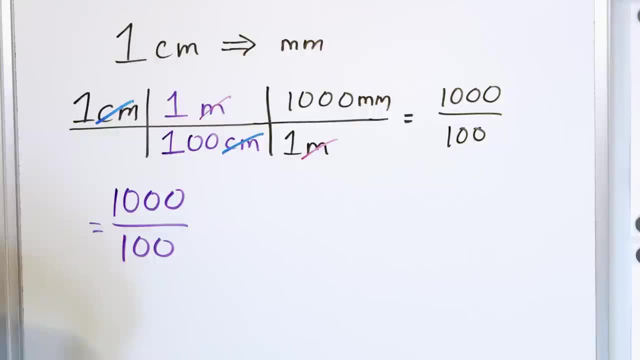 on the bottom. 100 times 1 is 100. So what I have is 1,000 on the top and 100 on the bottom. So 1,000 on the top and 100 on the bottom. Remember I told you. 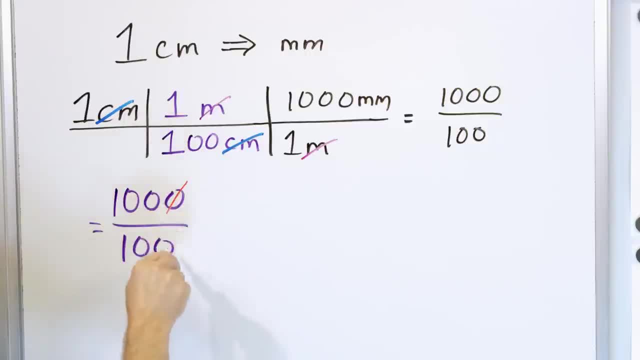 the same thing. If you have trailing zeros like this, this zero can cancel with this one, this zero can cancel with this one. The answer that I get on the top is a 10 and on the bottom is a 1, and 10 divided by 1 is 10 and the unit is 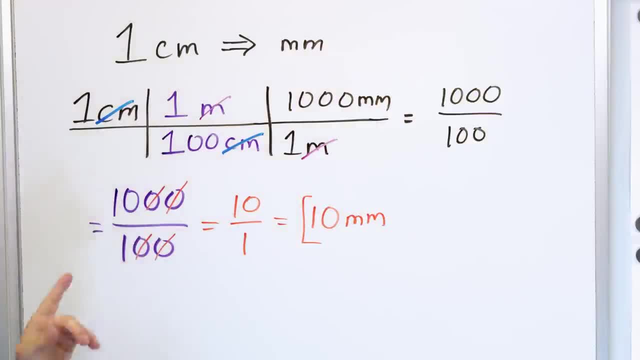 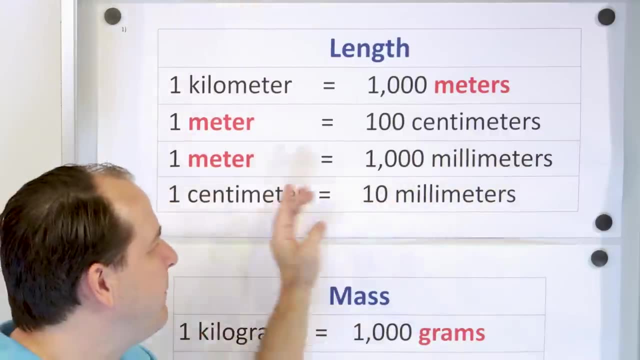 millimeters, And what we're saying is that 1 centimeter is 10 millimeters. 1 centimeter is 10 millimeters. So we've proven that what is in the chart is correct, but not by using this line, by using everything else, And so. 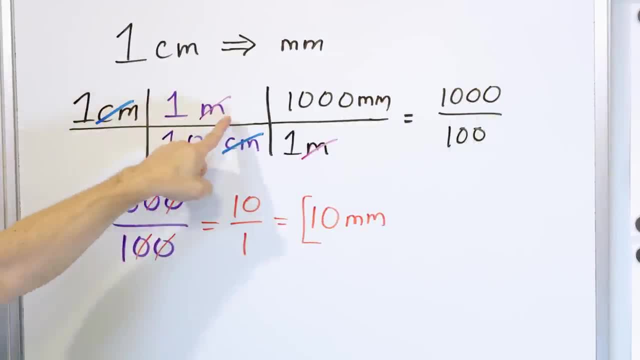 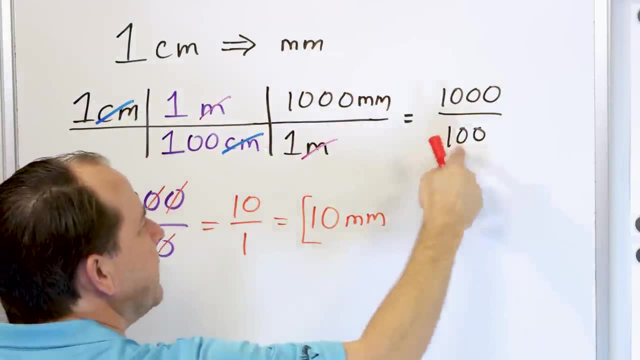 what we did is we said: well, one, we go from centimeters to meters, and then we go from meters to millimeters, and then we multiply everything on the top, multiply everything on the bottom, and then we do this division. But when we 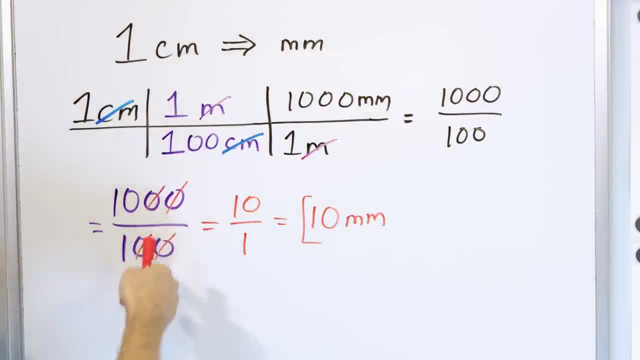 divide with trailing zeros like this. we can cancel the trailing zeros and then it makes everything simple. I don't have to do any like super hard division, because dividing by 100 is really, really easy, right? Last thing I want to talk about is the division. So I'm going to talk about 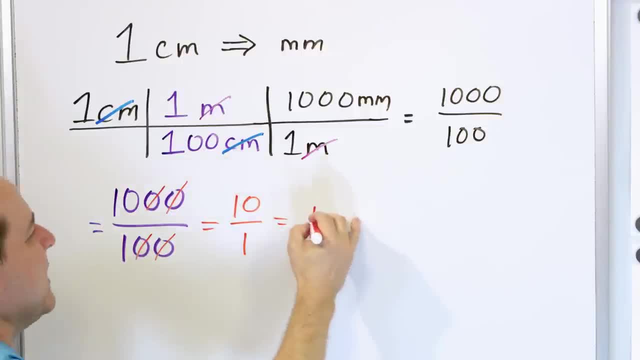 top is a 10. And on the bottom is a 1. And 10 divided by 1 is 10. And the unit is millimeters, And what we're saying is that 1 centimeter is 10 millimeters. 1 centimeter is 10 millimeters. 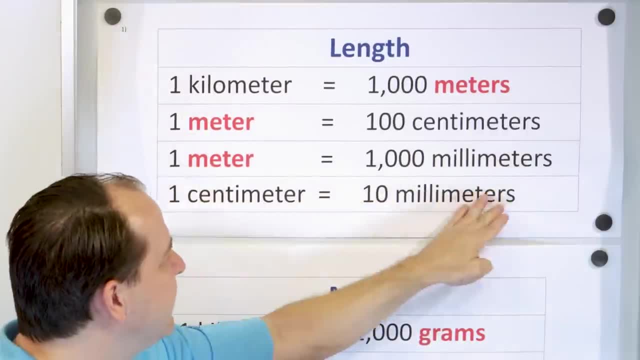 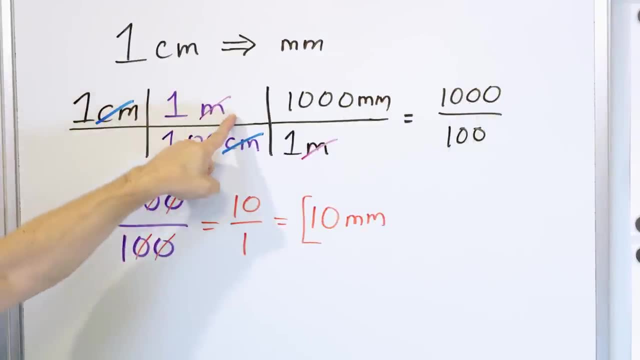 So we've proven that what is in this chart is correct, but not by using this line, By using everything else. And so what we did is we said: well, one, we go from centimeters to meters, and then we go from meters to millimeters, and then we multiply everything on the top, multiply. 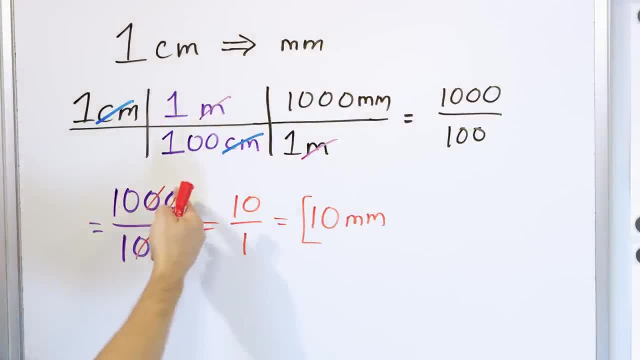 everything on the bottom and then we do this division. but when we divide with trailing zeros like this, we can cancel the trailing zeros and then it makes everything simple. I don't have to do any like super hard division, because dividing by a hundred is really really easy, right? last thing I'll say is you: 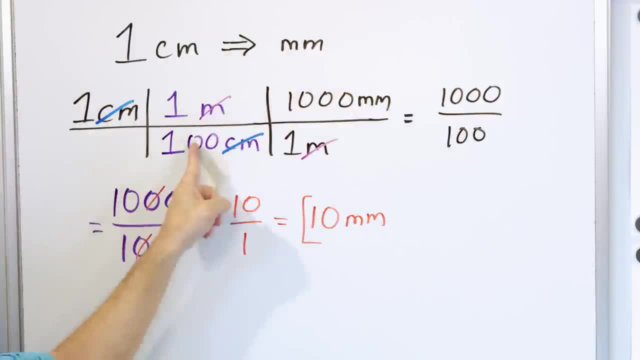 can think of this two ways. you can think of it as multiplying the tops, multiplying the bottoms and then dividing. or you can think of it as one times one is one, then divide by a hundred, then multiply by a thousand, then divide by one, so it's, it's. 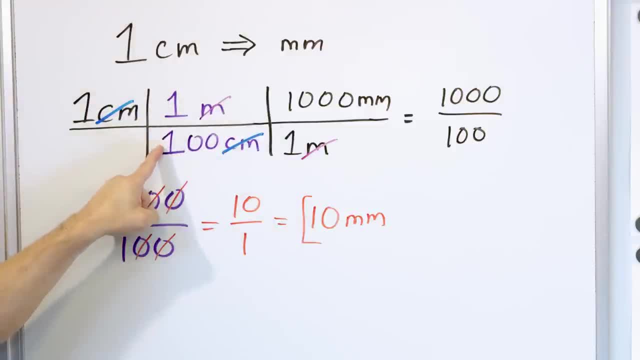 the same thing, it's just in a different order. so one times one is one. if you divide by a thousand, by hundred, one divided by a hundred, if you do the long division, you'll get a decimal. if you take that and then multiply by a thousand, then you'll get the answer. but it's doing it this way. it's easier if 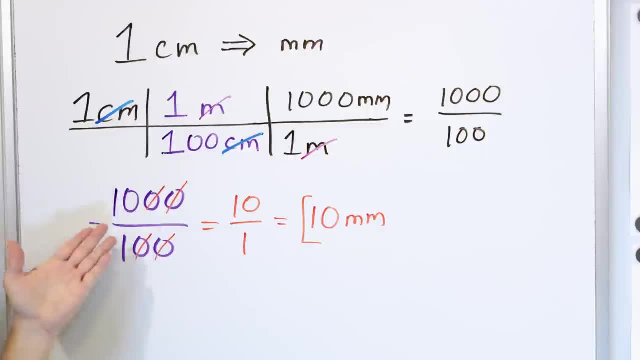 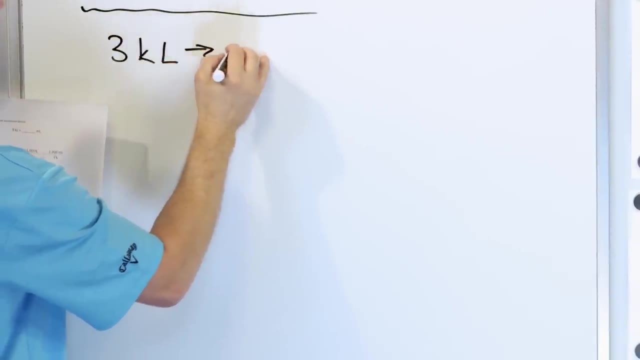 you multiply the tops and multiply the bottoms, then you'll get to the answer, because you can cancel these things much, much faster and much, much easier. all right, with more practice comes you know many more skills, so let's continue along. what about three kiloliters? let's go to milliliters. so what we want to do is write down what we. 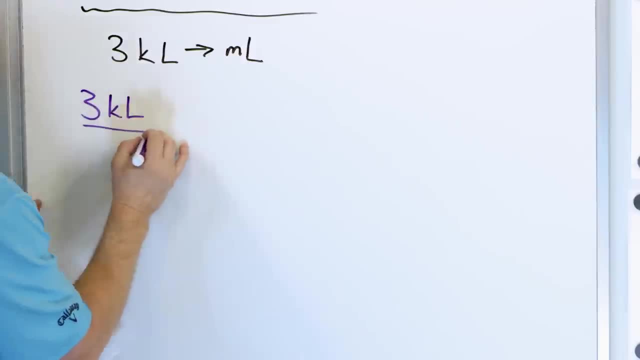 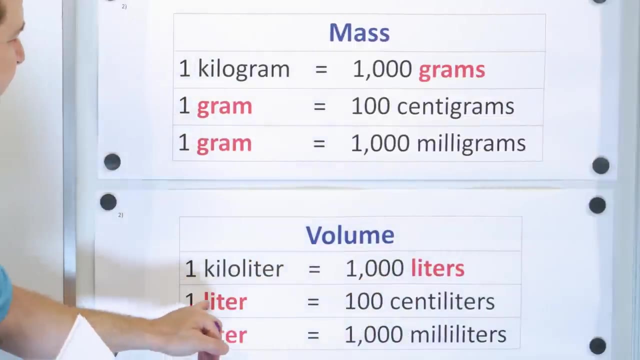 have been given three kilo liters. now we want to try to find a conversion that goes from kilo liters to milliliters, that's kilo liters- liters. there is no conversion that goes from kilo liters directly to milliliters to milliliters. 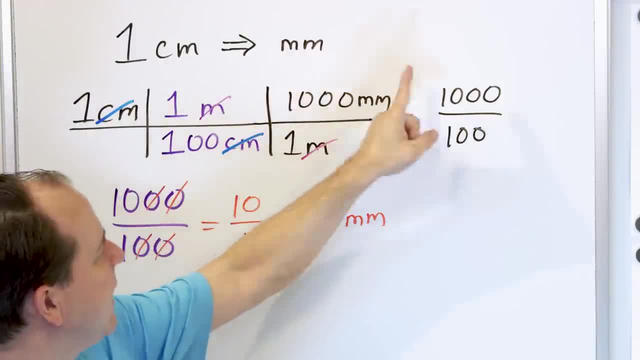 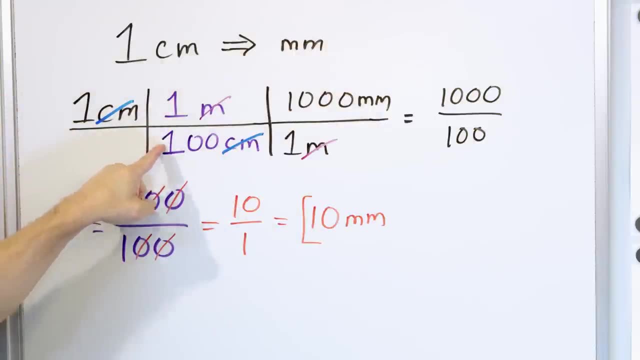 division. So the first thing I'll say is: you can think of this two ways. You can think of it as multiplying the tops, multiplying the bottoms and then dividing, Or you can think of it as: 1 times 1 is 1, then divide by 100, then 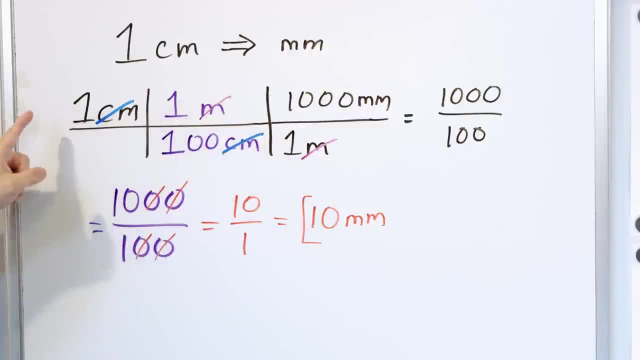 multiply by 1,000, then divide by 1.. So it's the same thing, It's just in a different order. So 1 times 1 is 1.. If you divide by 100,, 1 divided by 100, if 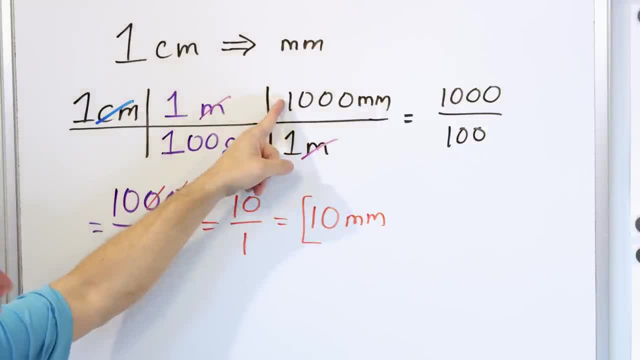 you do the long division, you'll get a decimal. If you take that and then multiply by 1,000, then you'll get the answer. But doing it this way is easier. If you multiply the tops and multiply the bottoms, then you'll get to. 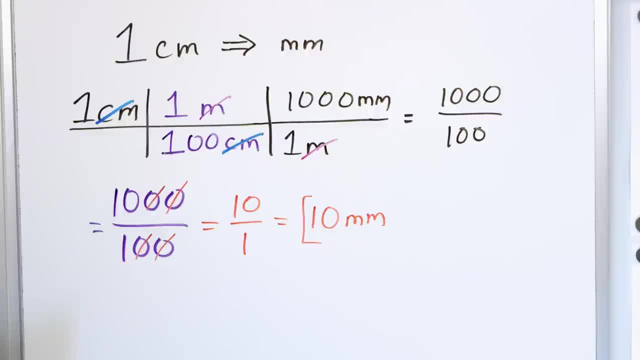 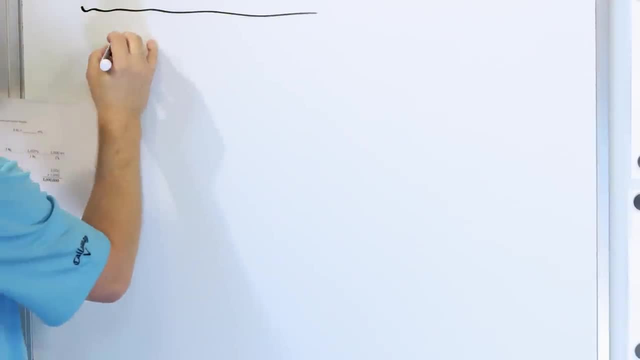 the answer because you can cancel these things much, much faster and much, much easier. All right, with more practice comes many more skills, So let's continue along. What about 3 kiloliters? Let's go to milliliters. So what we want to do is: 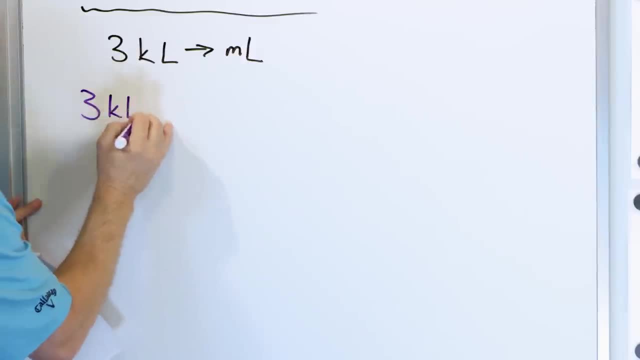 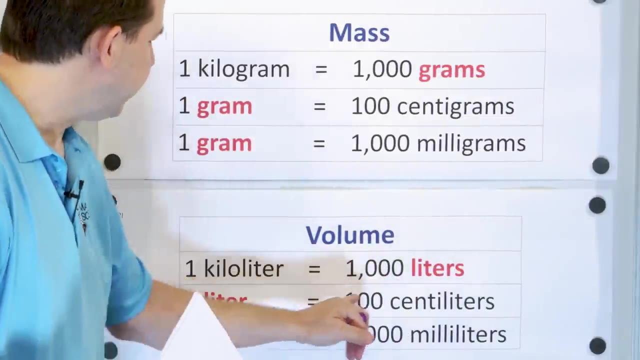 write down what we have been given: 3 kiloliters. Now we want to try to find a conversion that goes from kiloliters to milliliters, That's, kiloliters to milliliters, Kiloliters, liters. There is no conversion that goes from kiloliters directly to. 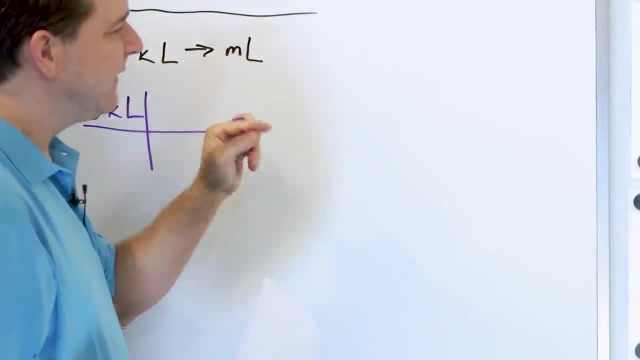 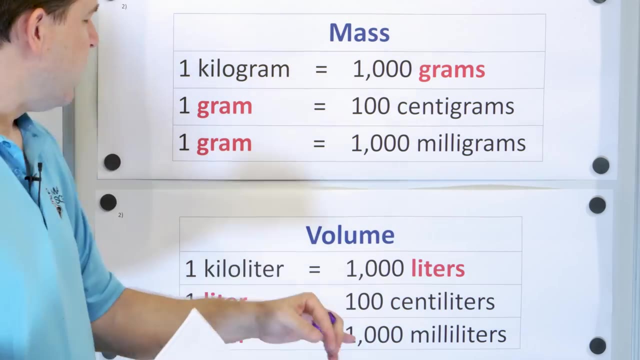 milliliters. So we can't do that. Is there another path to the answer? We can go from kiloliters to liters and then from liters to milliliters. So we do it in two steps. So we know that 1 kiloliter is 1,000 liters, because kilo means 1,000.. So 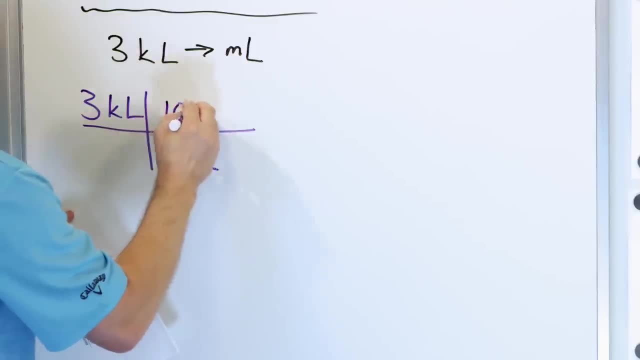 1 kiloliter- we write it down on the bottom- is 1,000 liters. We write it down this way because this is the only way kiloliters cancels. If we stop the calculation here, we'll just get liters. But we don't want liters. 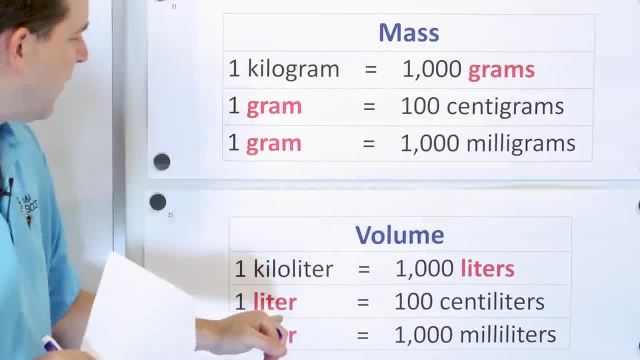 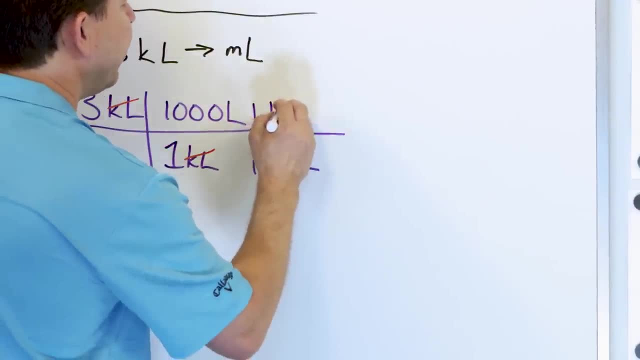 so we continue. We go from liters to milliliters, Liters to milliliters. 1 liter is 1,000 milliliters. We write 1 liter on the bottom, 1,000 milliliters on the top. Now liters cancels. 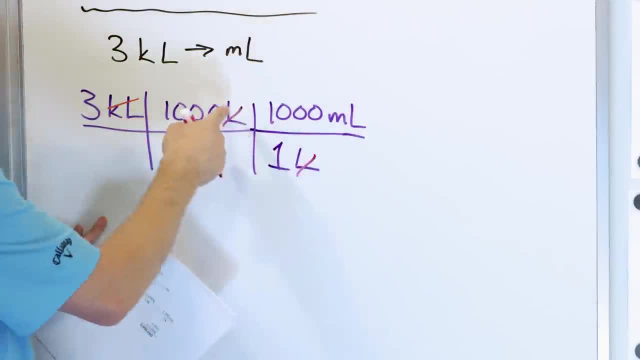 with liters. We wrote it this way: If we flipped it over, nothing would cancel. We have to write it this way to make it cancel, And so everything is canceled, except now we have the unit at the end that we want. The reason we're doing all this, by the way, is because it's hard to know. do I multiply? 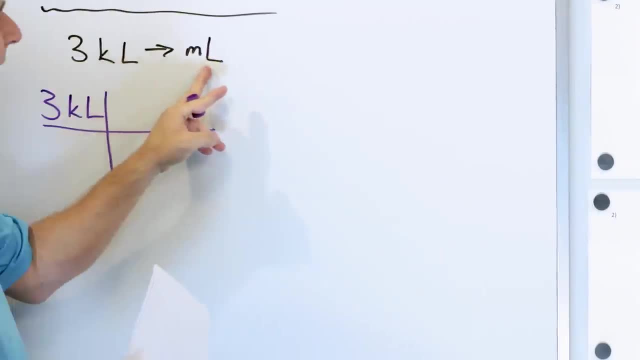 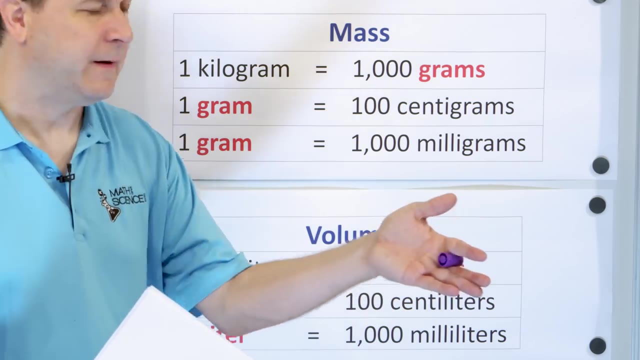 so we can't do that. is there another path to the answer? we can go from kiloliters to liters and then from liters to milliliters, so we do it in two steps. so we know that one kilo liter is 1,000 liters, because kilo means a. 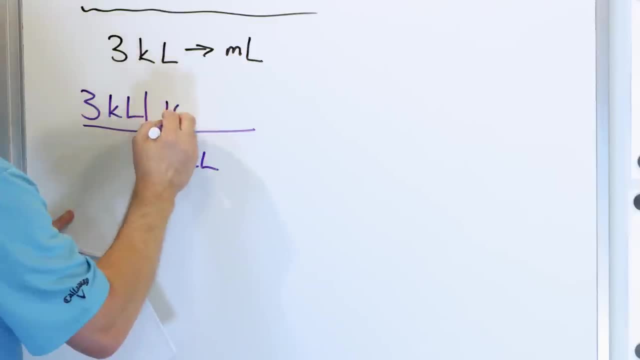 thousand. so one kilo liter- we write it down on the bottom- is 1,000 liters. we write it down this way because this is the only way kilo liters cancels. if we stop the calculation here, we'll just get liters. but we don't want leaders, so we 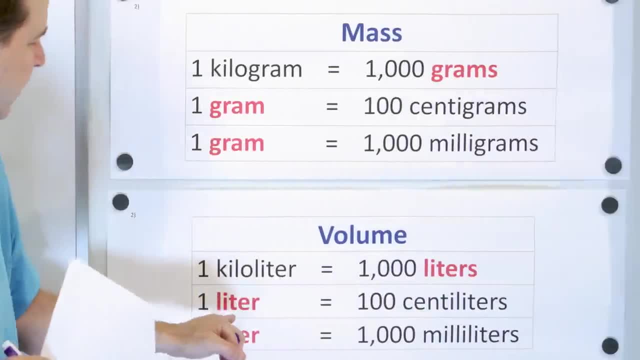 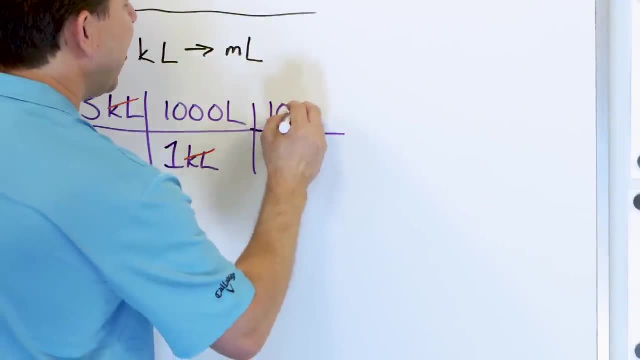 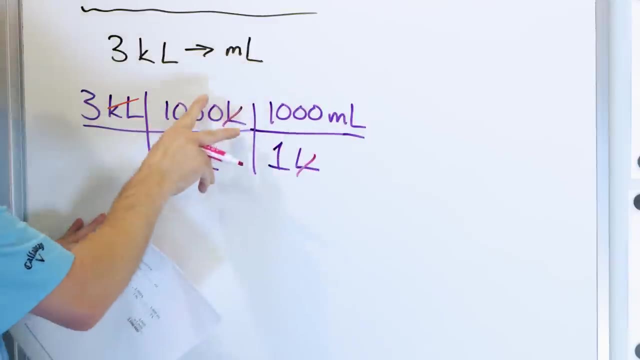 continue. we go from liters to milliliters, liters to milliliters. one liter is a thousand milliliters. okay, right, one liter on the bottom, 1,000 milliliters on the top. now leaders cancels with leaders. we wrote it this way. if we flipped it over, nothing. 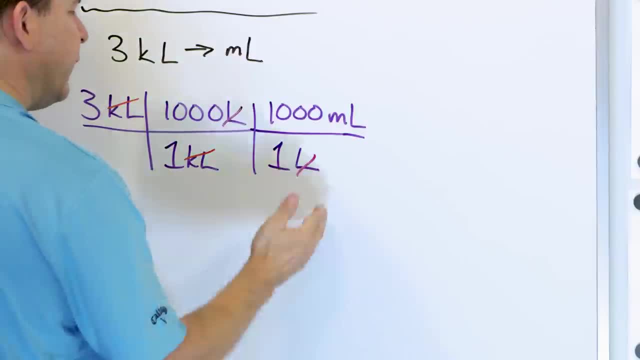 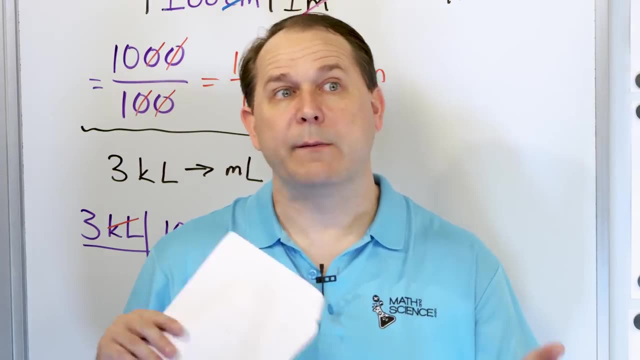 would cancel. we have to write it this way to make it cancel, and so everything is canceled, except now we have the unit at the end that we want. the reason we're doing all this, by the way, is because it's hard to know: do I multiply or do I? 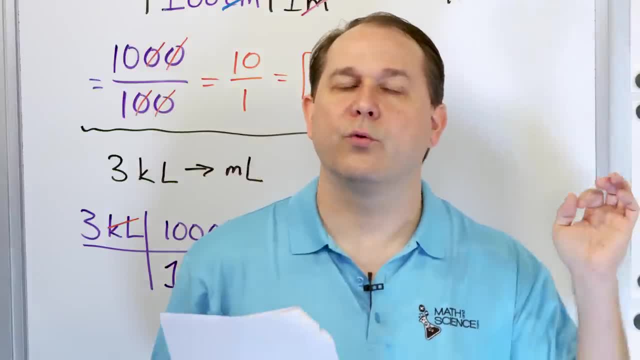 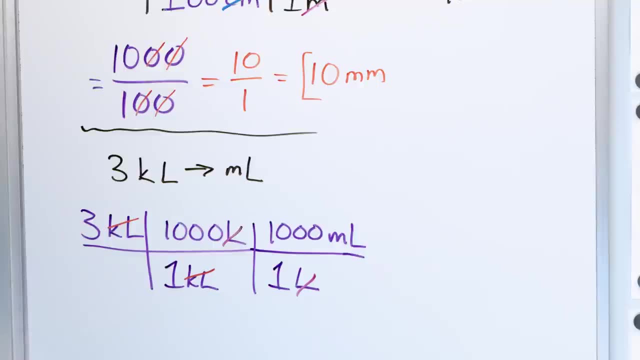 divide by these conversion factors. and this way of doing it makes it very easy. you don't have to guess, you always know what to do, because this is the only way that it can be written down to get the right answer. how do I finish it? well, I. 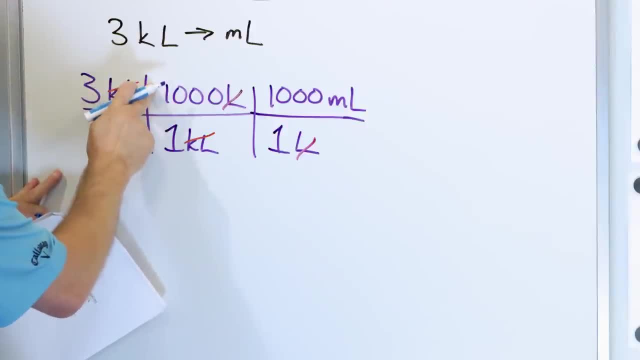 say I have on the top 3 times a thousand and then I have to divide by one- that's not going to change anything- and then multiply by another thousand and then divide by one- that's not going to change anything. so the dividing by the ones isn't really going to do anything. so three times a thousand is three thousand. 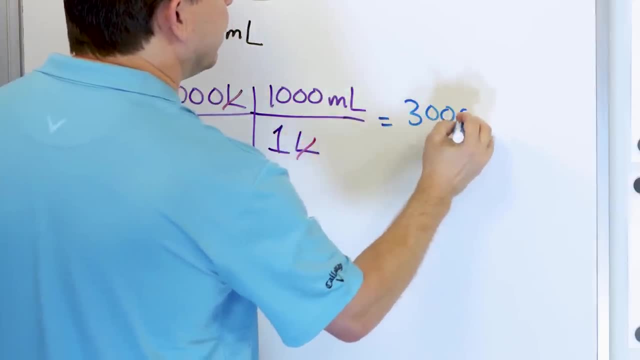 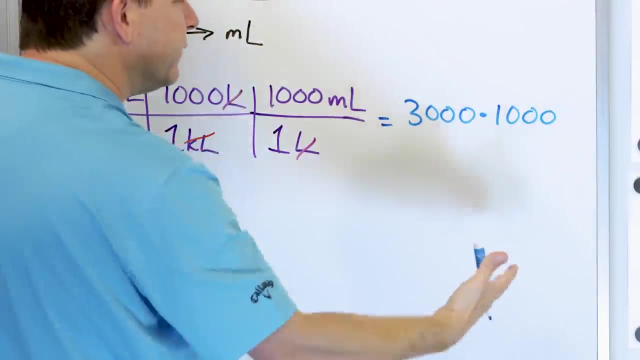 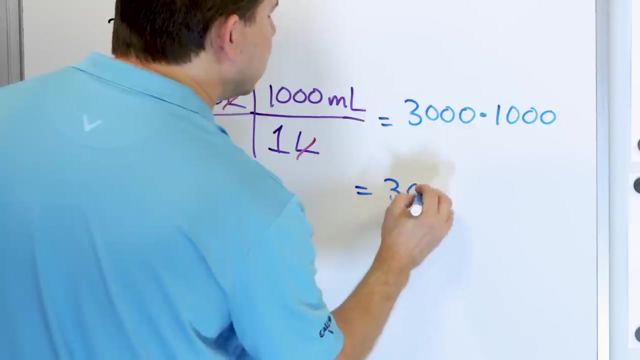 right. so what I have here is three thousand, but I still have to multiply by another thousand. now, how do I do this? of course, I can write it all down and do all the long, the long multiplication. but I know that when I multiply by a power of ten, all I have to do is write down its cover up, essentially cover up the. 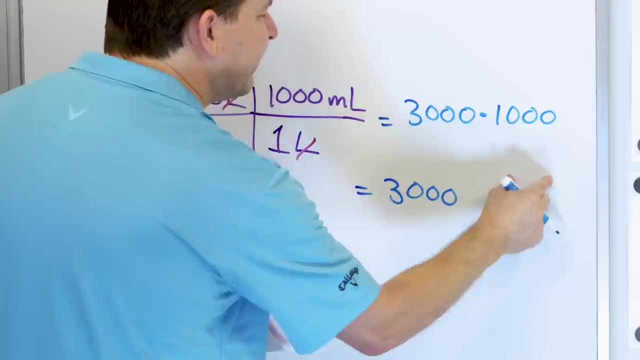 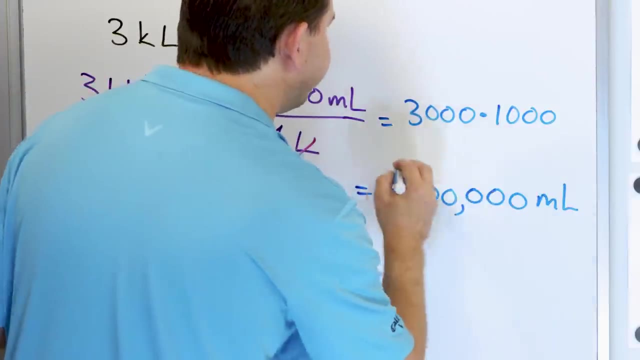 zeros here I'm multiplying by one, so I'm gonna get three thousand, and then I'll just add these zeros back in three more of them, and so it's going to be three million, and the unit here is milliliters, so the unit is three million milliliters. another way to look at it is: 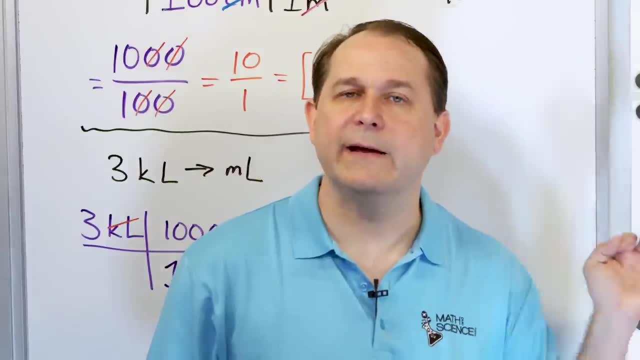 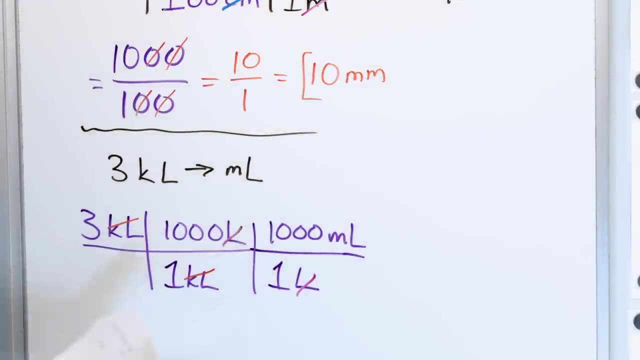 or do I divide by these conversion factors? And this way of doing it makes it very easy. You don't have to guess, You always know what to do, because this is the only way that it can be written down to get the right answer. Now, how do I finish it? Well, I say I have. 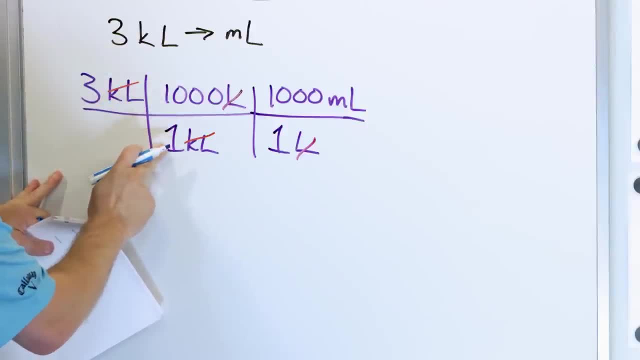 on the top 3 times 1,000, and then I have to divide by 1.. That's not going to change anything. And then multiply by another 1,000 and then divide by 1. That's not going to change anything. 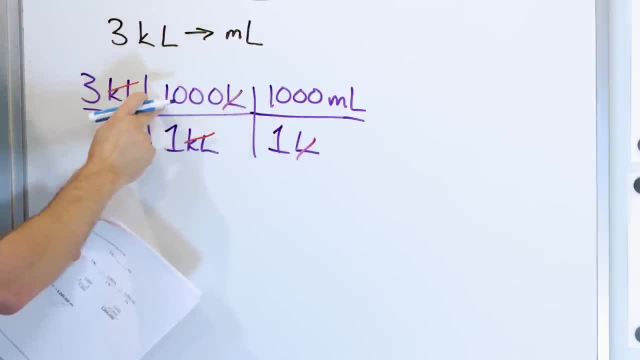 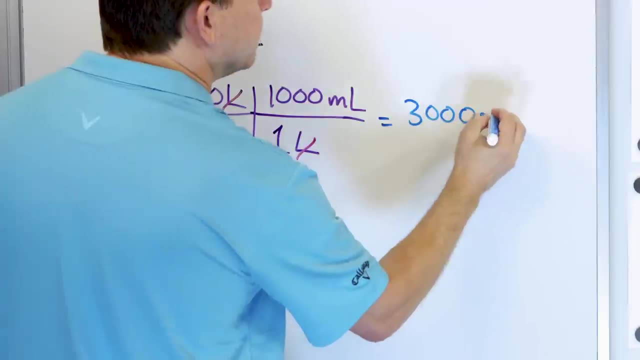 That's not really going to do anything. So 3 times 1,000 is 3,000, right, So what I have here is 3,000.. But I still have to multiply by another 1,000.. Now how do I do this Of? 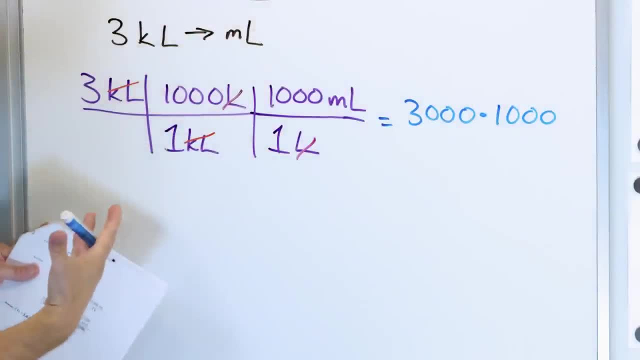 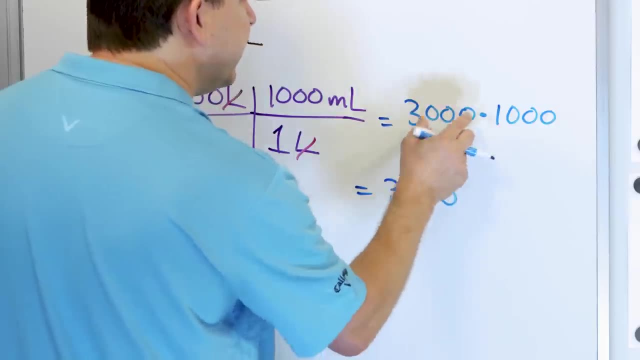 course I can write it all down and do all the long multiplication, But I know that when I multiply by a power of 10, all I have to do is write down, essentially cover up the zeros. here I'm multiplying by 1. So I'm going to get 3,000, and then I'll just add these. 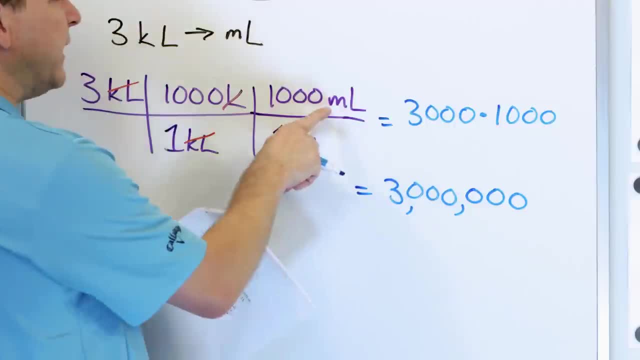 zeros back in Three more of them, And so it's going to be 3,000,000, and the unit here is milliliters, So the unit is 3,000,000 milliliters. Another way to look at it is: I can multiply this and: 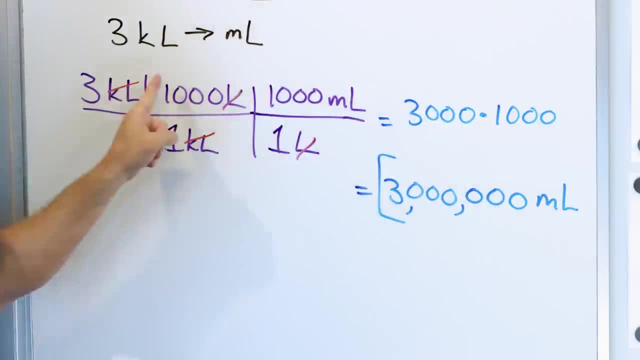 3 times 1 is 3, and I add three zeros to the end And then I take that and multiply by 1,000, again multiplying by 1, so that makes it 3,000, and then I add the zeros in again. 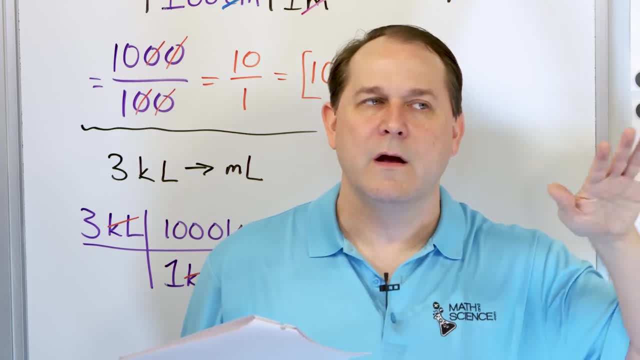 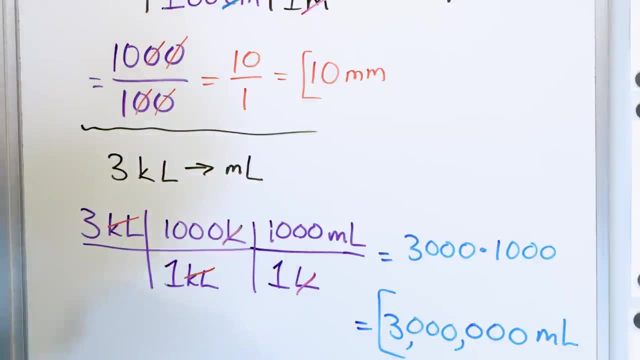 So, basically, when you multiply by 1,000, you just kind of cover up the zeros, multiply by 1. And then add the zeros back in at the end. That's all you're doing. So that's why there's six zeros here, because there's six zeros throughout here. 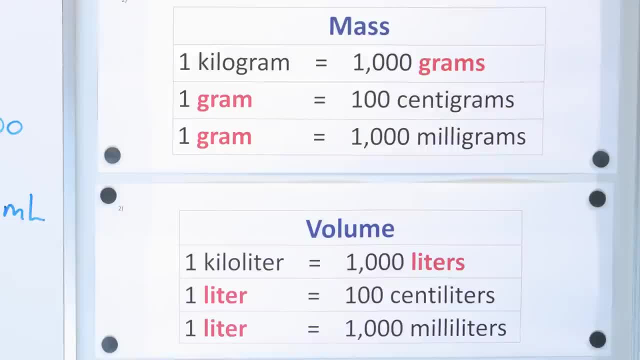 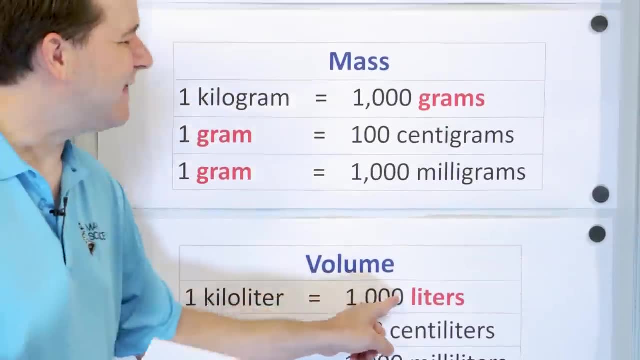 Now does this make sense? Let's see if this actually makes sense. We're saying: three kiloliters is 3,000,000 milliliters. Okay, Three kiloliters is 3,000 of these liters And every one of. 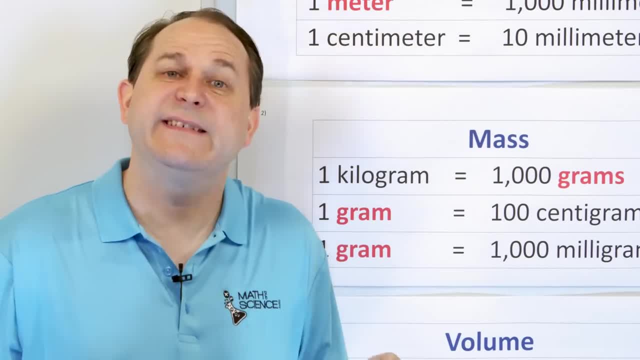 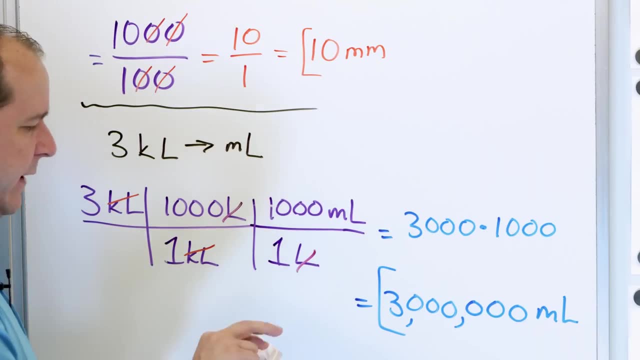 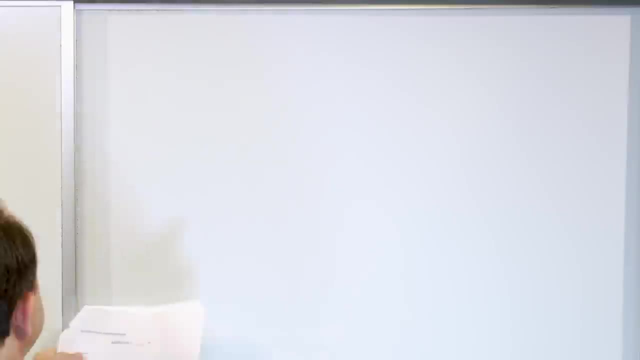 these liters has a thousand of these milliliters. So it makes sense that 3,000 of these of these liters would yield a huge number of milliliters, And that is exactly what we found. All right, let's move right along to problem number five. What about 42,000 millimeters? 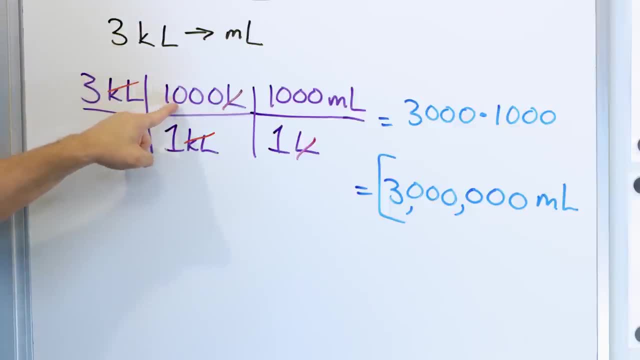 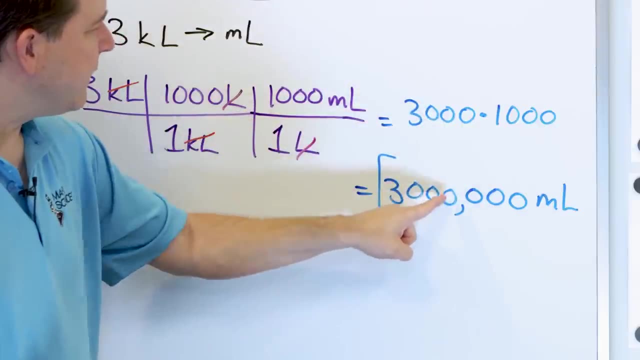 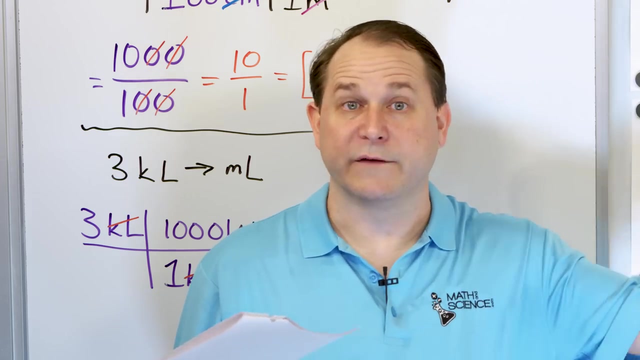 I can multiply this and three times one is three, and I add three zeros to the end, and then I take that and multiply by a thousand. again I'm multiplying by one, so that makes it three thousand, and then I add the zeros in again. so basically, when you multiply by a thousand you just kind of cover up the zeros, multiply by. 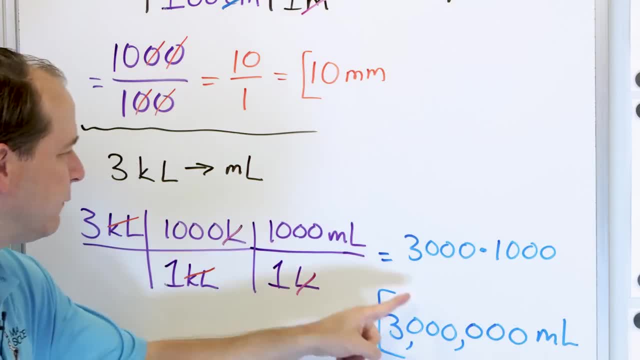 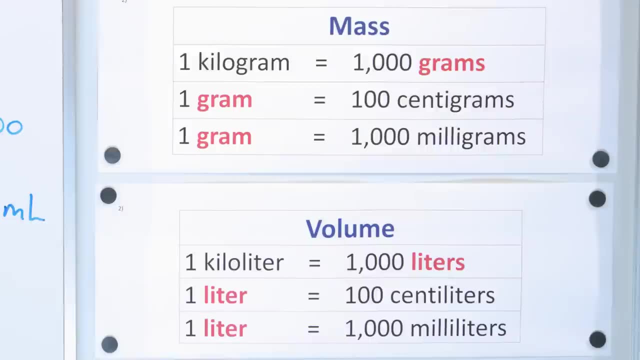 one and then add the zeros back in at the end. that's all you're doing. so that's why there's six zeros here, because there's six zeros throughout here. now, does this make sense? let's see if this actually makes sense. we're saying: three kiloliters is three million milliliters, okay, three. 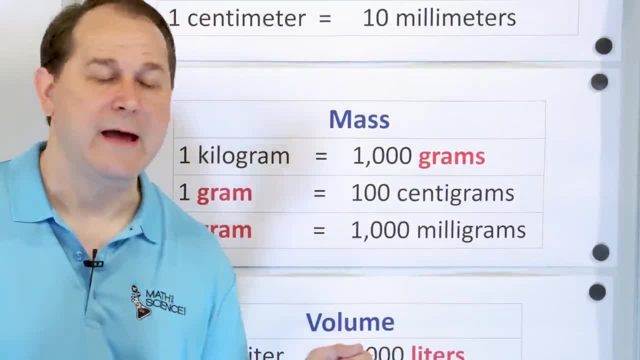 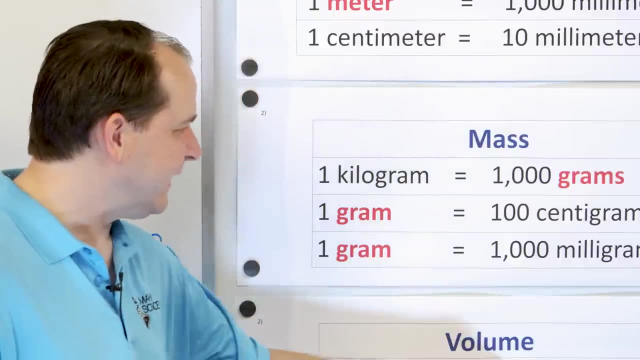 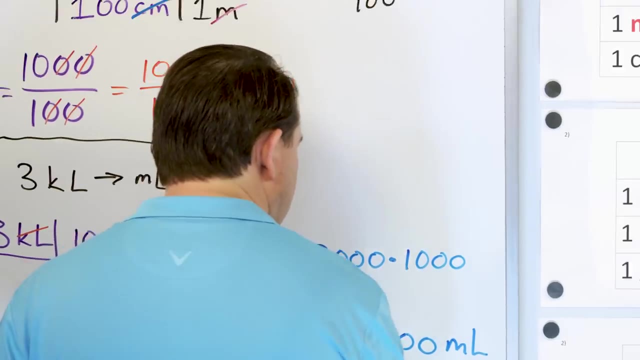 kiloliters is three thousand of these liters, and every one of these liters has a thousand of these milliliters. so it makes sense that three thousand of these of these liters would yield a huge number of milliliters, and that is exactly what we found. all right, let's move right along. 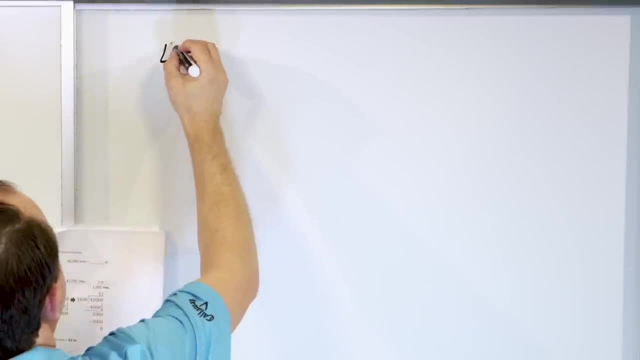 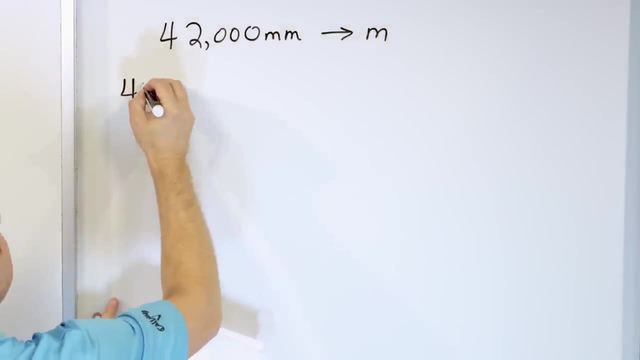 to problem number five. what about forty two thousand millimeters, and let's convert that to meters? so first we write down forty two thousand millimeters and we want to convert that to meters. now let's think about it. can we figure it out without looking at the chart? well, millimeter, milli means one thousand. 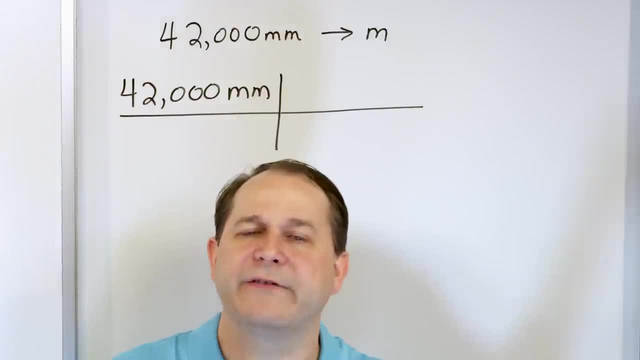 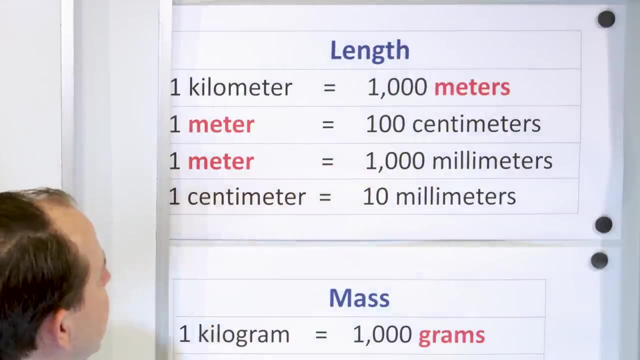 times smaller. so if I'm going from millimeters to meters, I think there's a thousand of those little bitty millimeters in a meter. let's see if we're right. a thousand millimeters is equal to one meter. that's the conversion factor we want to use and the only way we can. 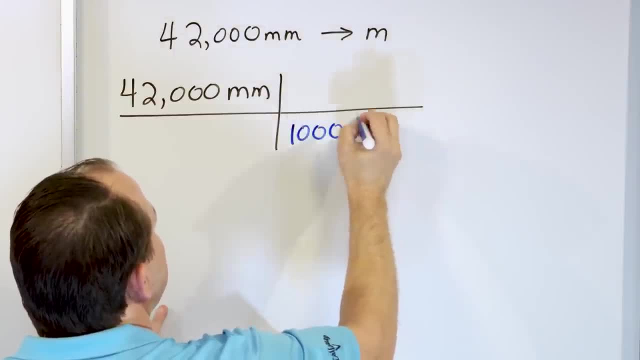 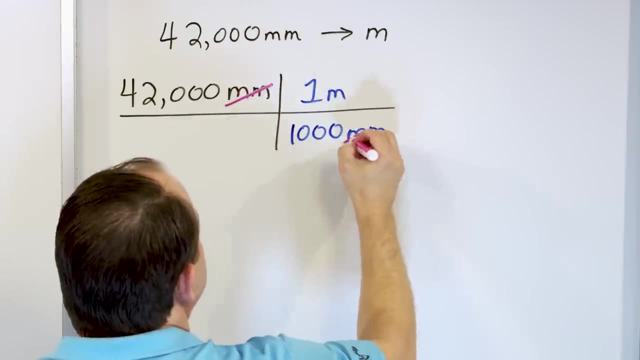 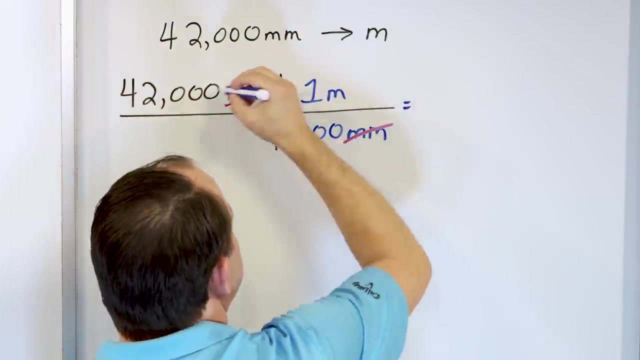 write: it is a thousand on the bottom, millimeters is one meter. that's the only way it works, because if we write it upside down, we won't cancel anything here. we cancel millimeters, and so we have forty two thousand times one and we have to divide by this. so let's write it. we multiply the top, we're still gonna. 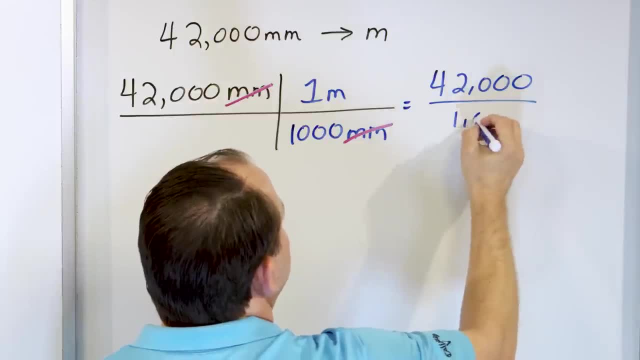 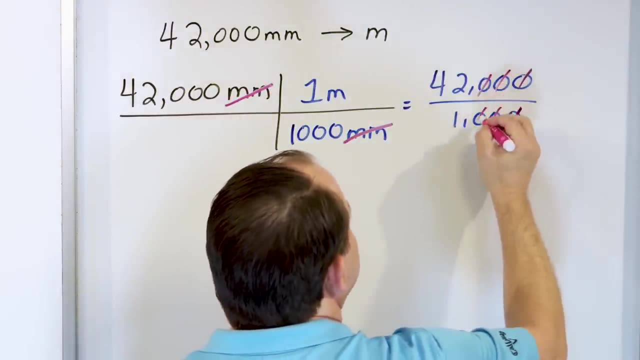 have forty two thousand, and on the bottom we have one thousand. all right, and so what do we get? we can cancel this zero with this one, this cancels with this one, this cancels with this one. what do I get? 42 on the top divided by one on the bottom, and so the 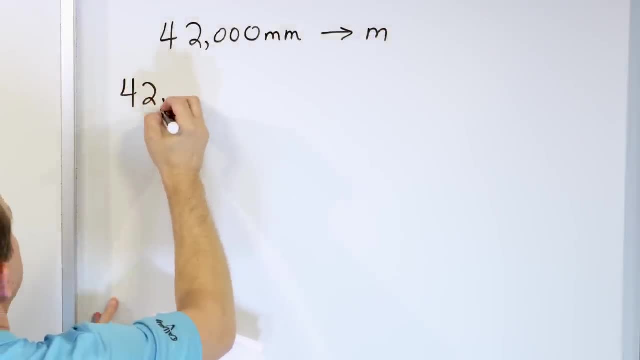 And let's convert that to meters. So first we write down 42,000 millimeters and we want to convert that to meters. Now let's think about it. Can we figure it out without looking at the chart? Well, millimeter, milli means 1,000 times smaller. 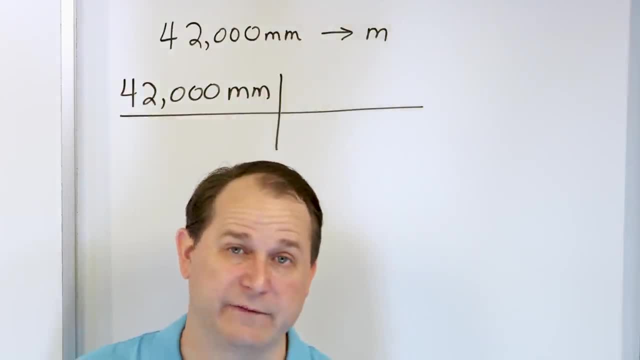 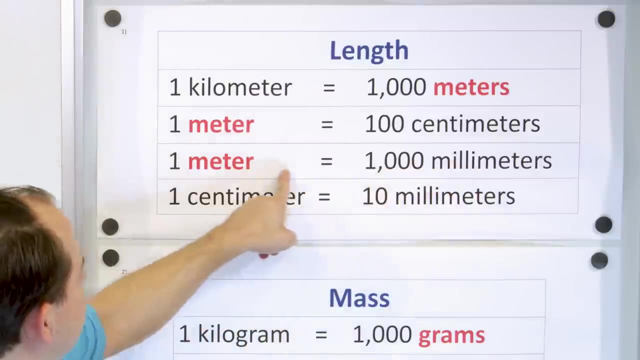 So if I'm going from millimeters to meters, I think there's a thousand of those little bitty millimeters in a meter. Let's see if we're right. A thousand millimeters is equal to one meter. That's the conversion factor we want to use And the only way we can write. 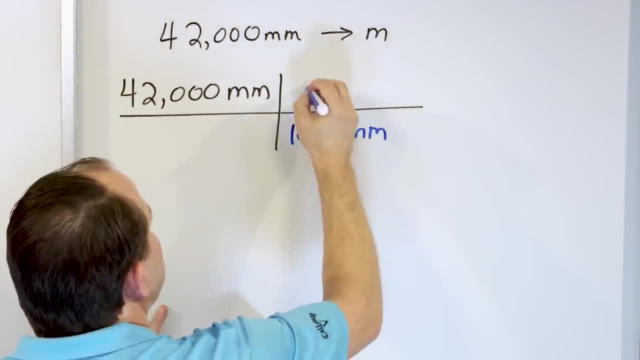 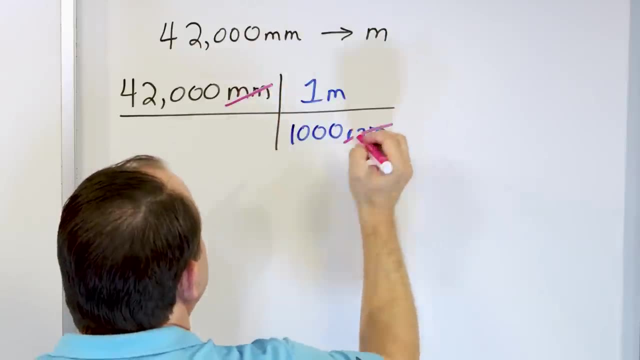 it is a thousand on the bottom. Millimeters is one meter. That's the only way it works, because if we write it upside down we won't cancel anything. Here we cancel millimeters, And so we have 42,000 times one. 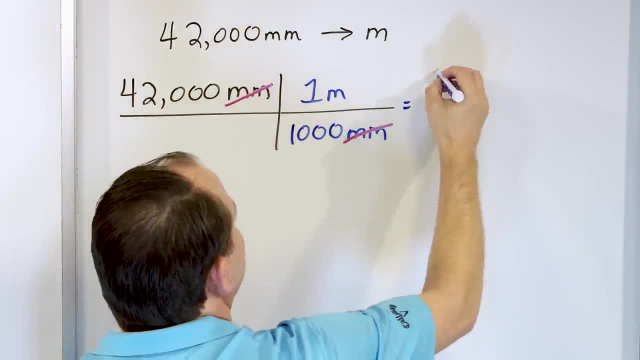 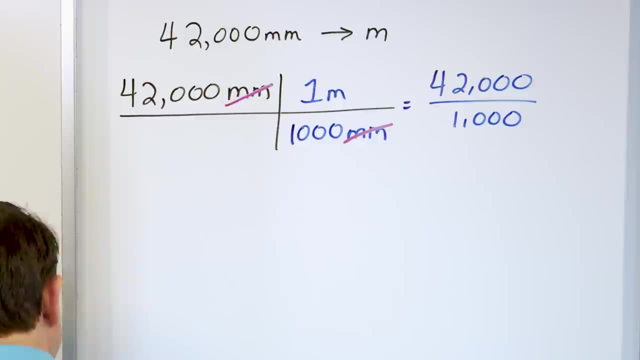 And we have to divide by this. So let's write it: We multiply the top, We're still going to have 42,000. And on the bottom, we have 1,000.. All right, And so what do we get We? 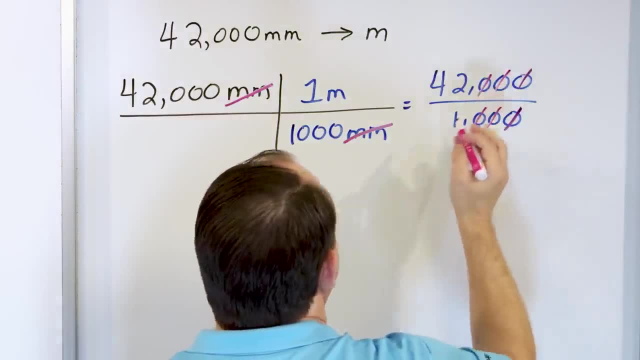 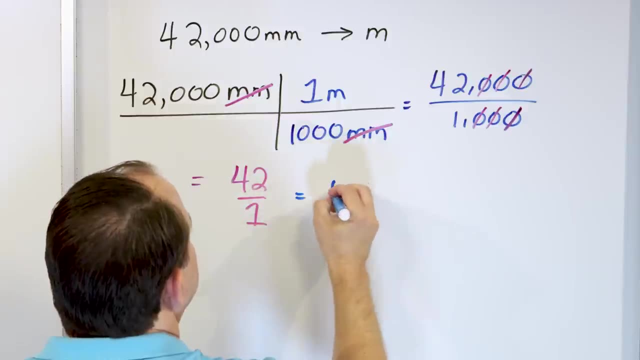 can cancel this zero with this one. This cancels with this one. This cancels with this one. What do I get? 42 on the top divided by one on the bottom, And so the answer I actually get is 42. And the unit left over is meters, So the answer is 42 meters. 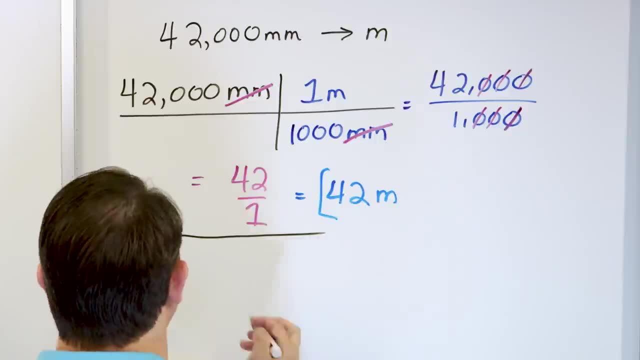 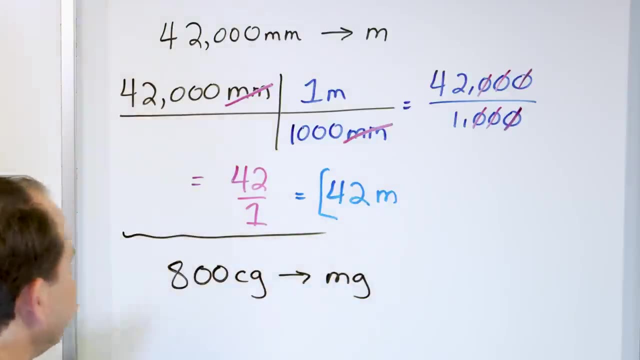 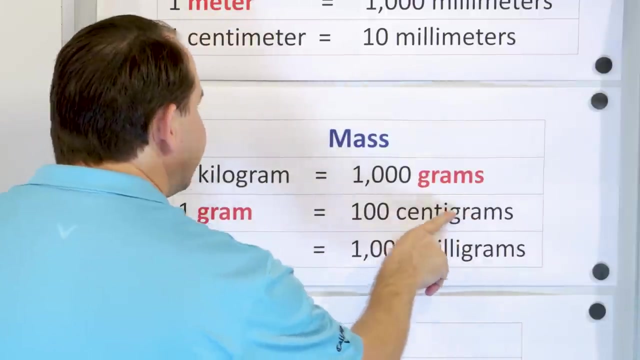 All right Crews run along making a little more progress. now that we know what we're doing- 800 centigrams- Let's convert that to milligrams. Now, I don't have a conversion that goes straight from centigrams to milligrams, But I do have something that goes from centigrams. 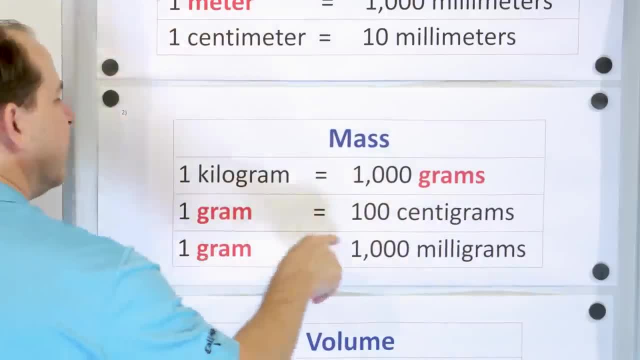 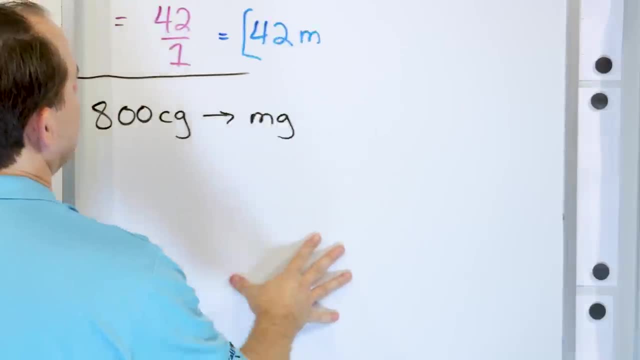 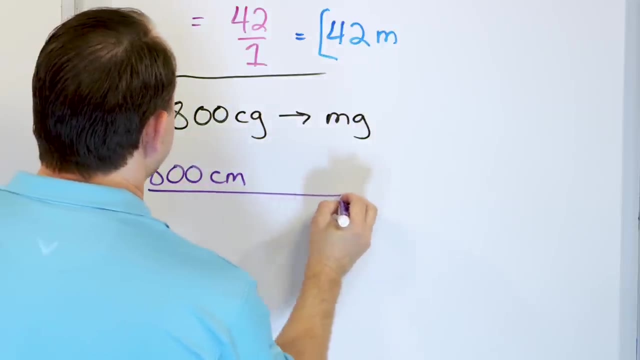 to grams, And then, once I'm in grams, I can go from grams to milligrams. So that's what we want to do. We want to do it in two steps. 100 centigrams is one gram, So let's first count what we know: 800 centigrams- Oops, not centimeters, Centigrams, Centigrams, And. 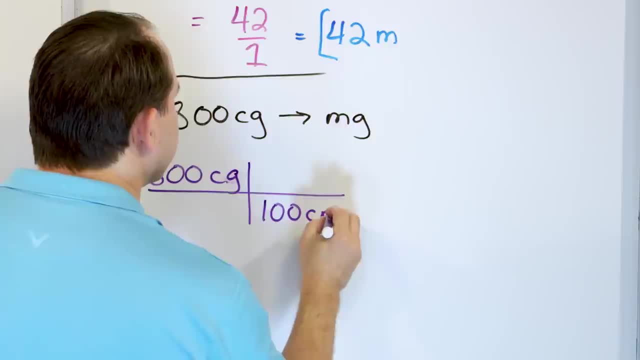 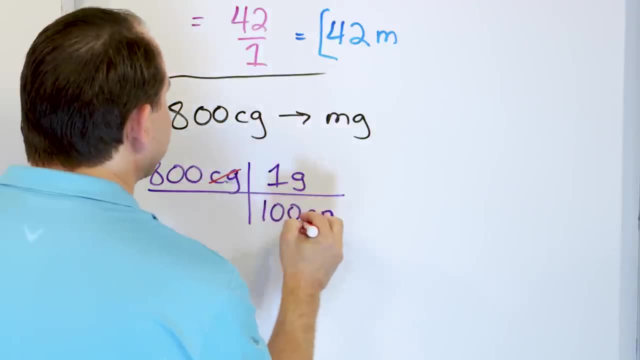 we just said that 100 of these little centigrams is one gram. Right, And we have to write it like that because that's the only way that centigrams will cancel. If we stop the calculation, we'll be left with grams. But we don't want to stop there. We want to go from grams to 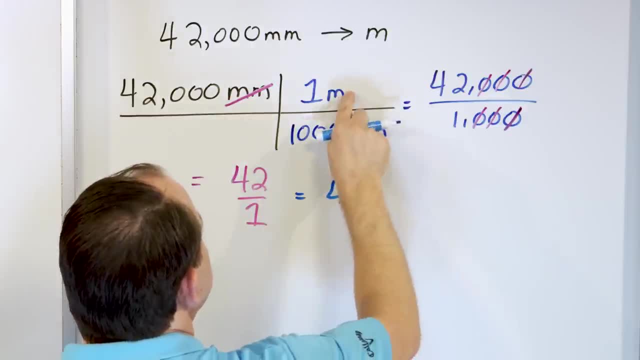 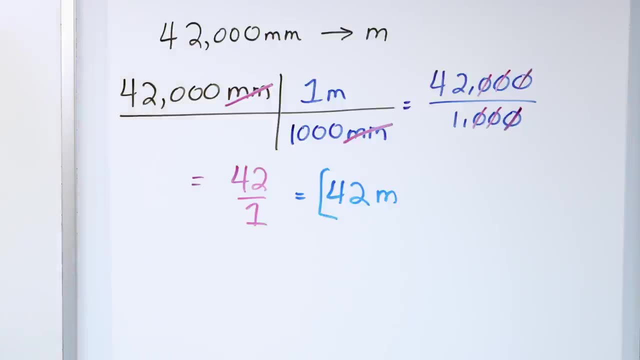 answer I actually get is 42, and the unit left over is meters, so the answer is 42 meters. all right, cruising right along, making a little more progress. now that we know what we're doing- centigrams- let's convert that to milligrams. now I don't have a conversion. 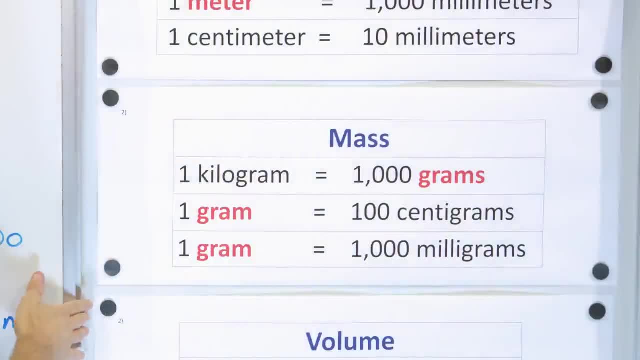 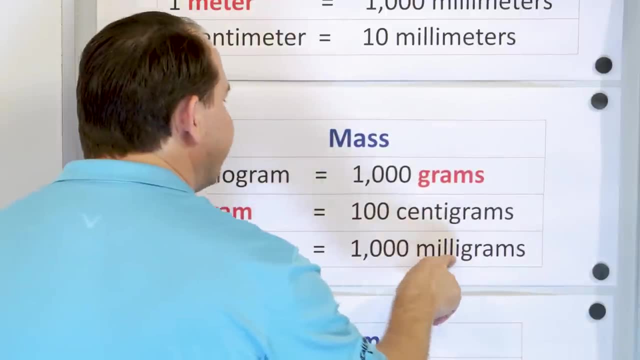 that goes straight from centigrams to milligrams, right, but I do have something that goes from centigrams to grams and then, once I'm in grams, I can go from grams to milligrams. so that's what we want to do. we want to do it in two steps. 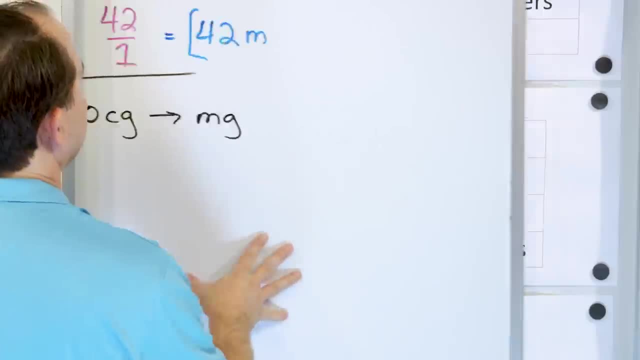 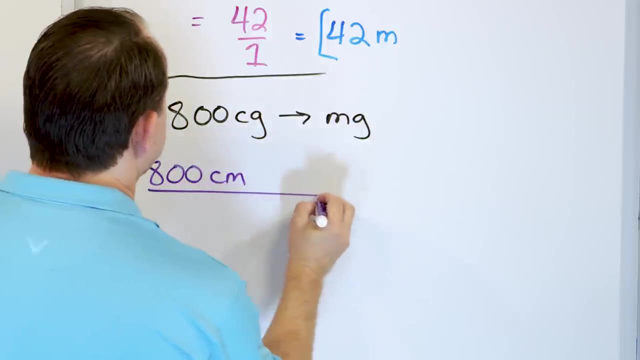 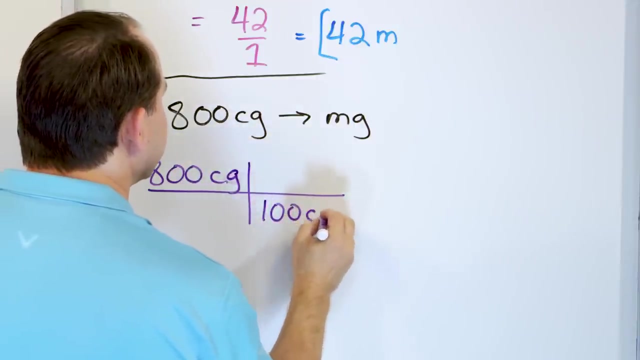 one hundred centigrams is one gram, so let's first write down what we know: 800 centigrams, oops, not even a centigrams, Oops, not centimeters. centigrams, Centigrams. And we just said that 100 of these little centigrams. 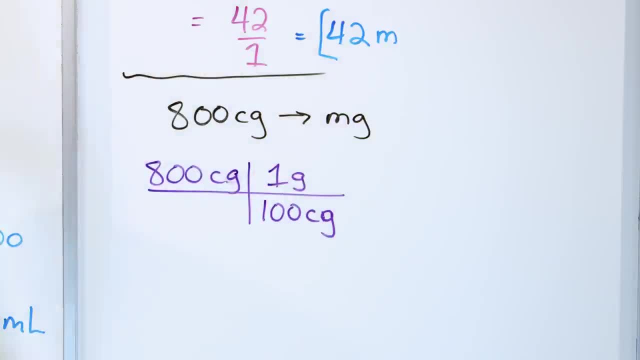 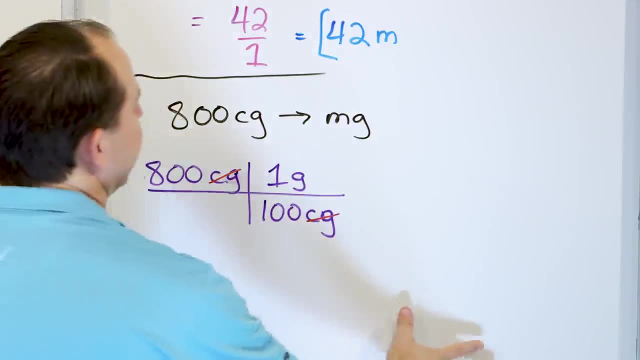 is one gram right, And we have to write it like that because that's the only way that centigrams will cancel. If we stop the calculation, we'll be left with grams. but we don't want to stop there. We wanna go from grams to milligrams. 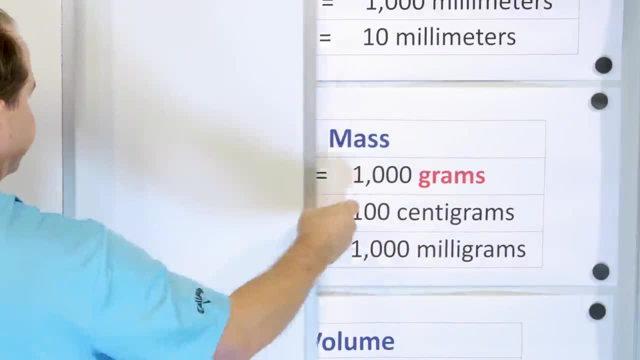 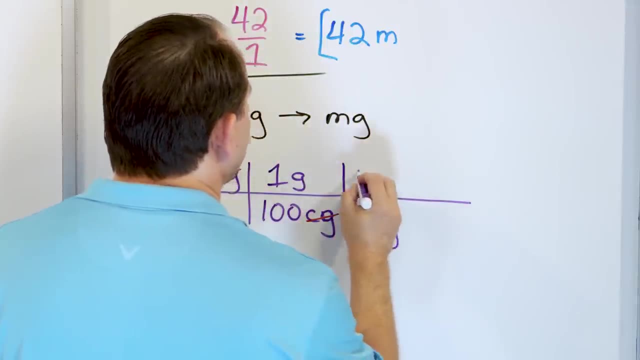 One gram is 1,000 milligrams. So we continue our table, We can string them along and we say that one gram is 1,000 milligrams And then, by arranging it like this, if we flip it over, nothing will cancel. 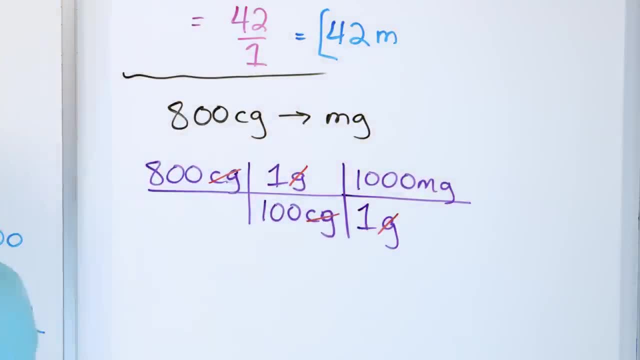 Arranging it like this means grams cancels with grams. Now how do we complete the calculation? Well, first we multiply the tops right, And by multiplying the tops we have 800 times 1, but that doesn't do anything- times 1,000. 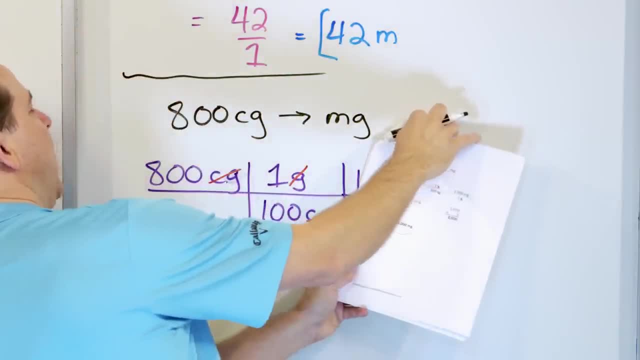 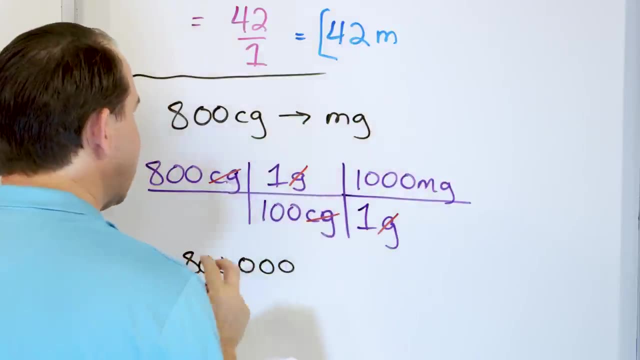 But it's easy to multiply that. We just cover up the zeros, multiply by one, we get 800, and then we have to add these zeros back in three more of them. So this is what happens when we multiply the top. 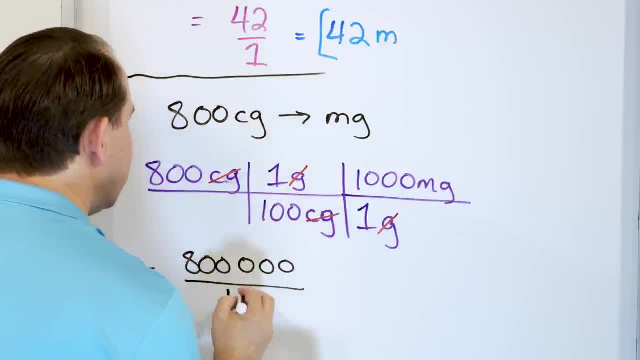 We have to divide by this, but this times one is still 100, so it's just gonna be 100 on the bottom. Now we have a lot of trailing zeros. This can cancel with this, and this can cancel with this. 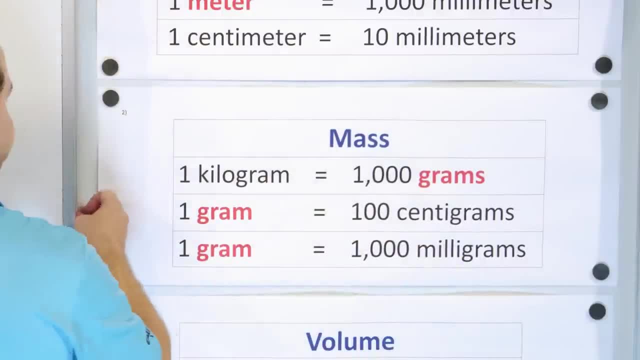 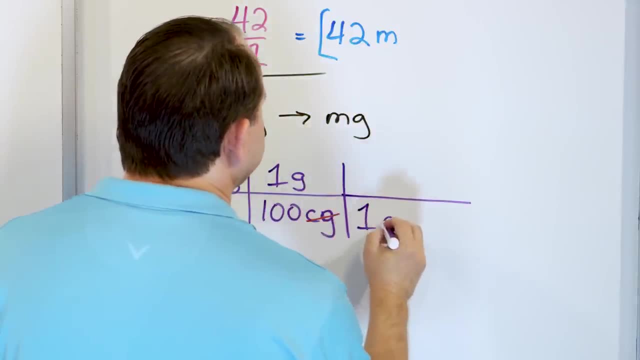 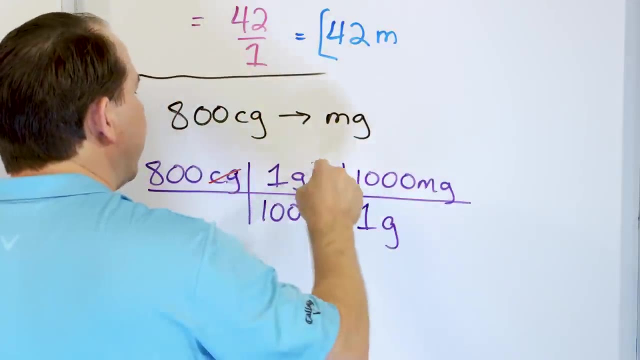 milligrams. One gram is 1,000 milligrams. So we continue our table, We can string them along And we say that one gram is 1,000 milligrams And then, by arranging it like this, if we flip it over, nothing will cancel Arranging. 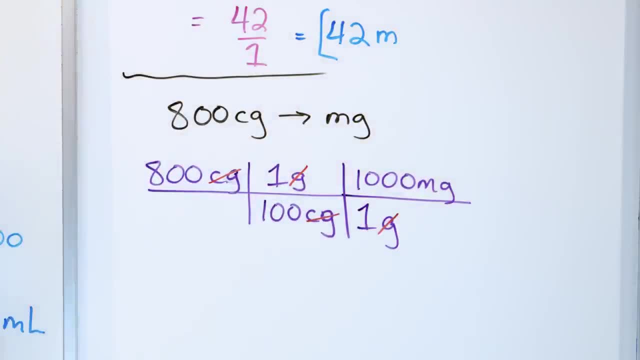 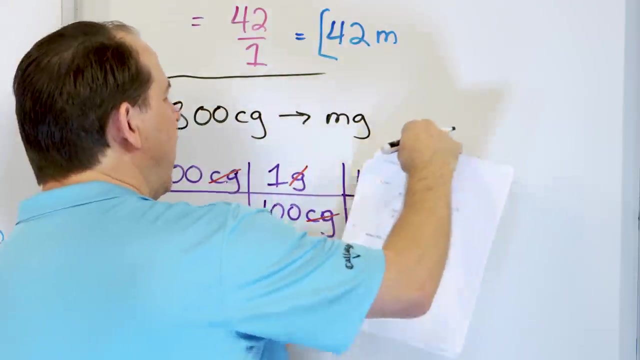 it like. this means grams cancels with grams. Now how do we complete the calculation? Well, first we multiply the tops Right, And by multiplying the tops we have 800 times 1., But that doesn't do anything. 1,000. But it's easy to multiply that. We just cover up the zeros and multiply by 1.. 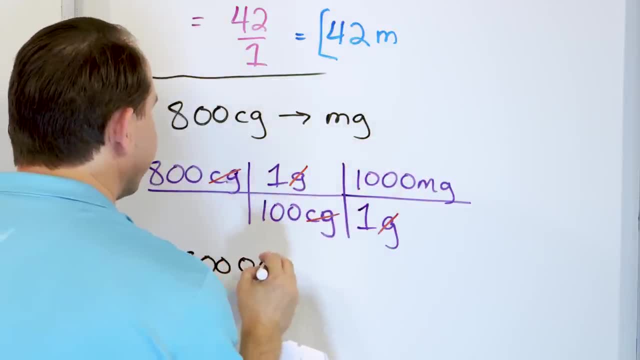 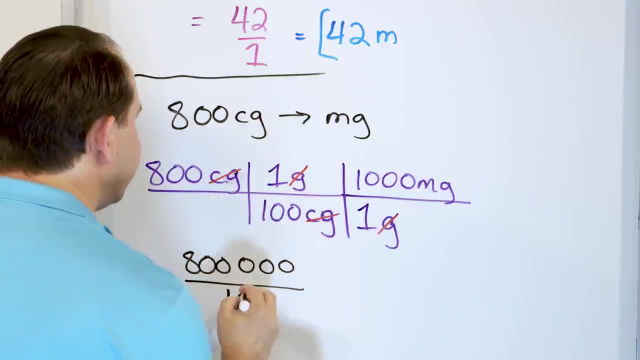 We get 800. And then we have to add these zeros back in three more of them. So this is what happens when we multiply the top. We have to divide by this, But this times 1 is still 100. So it's just going to be 100 on the bottom. 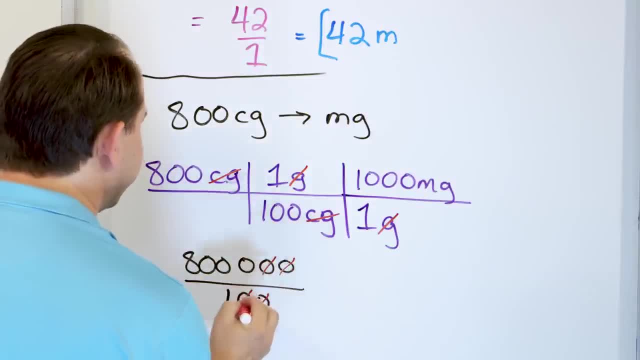 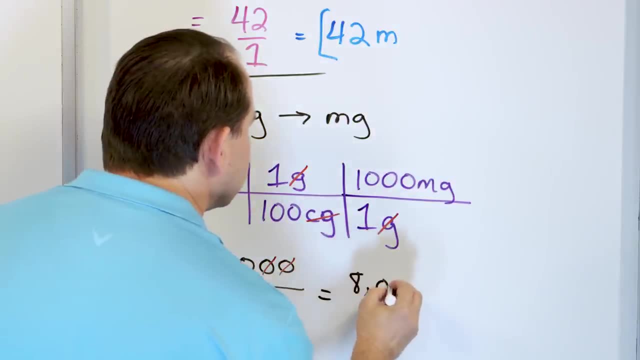 Now we have a lot of trailing zeros. This can cancel with this, And this can cancel with this, And so what's going to happen? On the top, I still have three zeros, So that's 8,000.. And then we divide it by the one that's on the bottom, And so what you have is 8,000.. 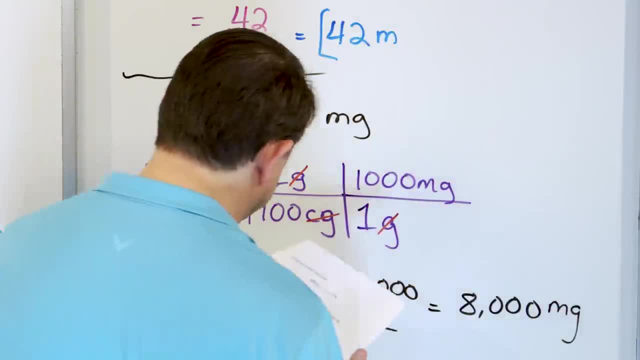 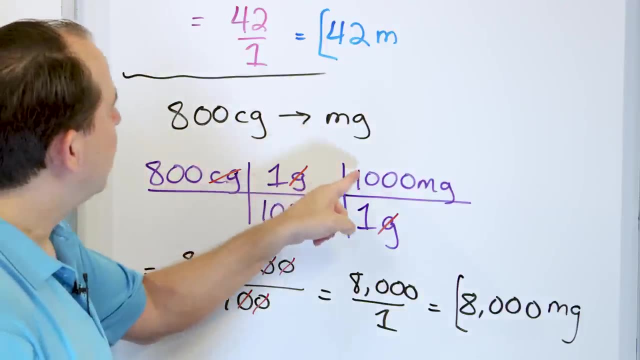 What are we talking about? Milligrams? That's the only unit left. Let me check and make sure that's right: 8,000 milligrams. So you see why it's so nice to work with the metric system, Because multiplying when you 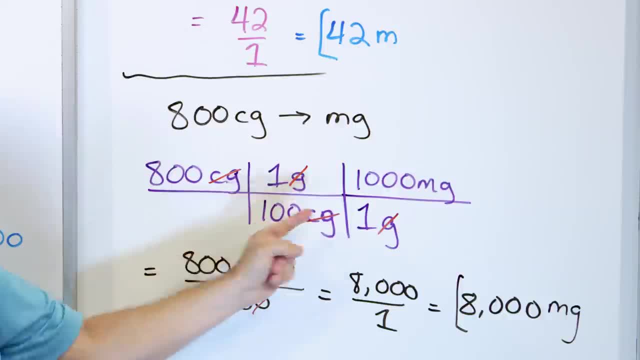 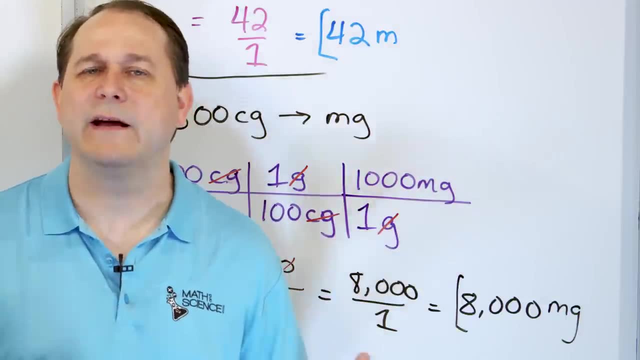 have a bunch of zeros makes it easy to multiply And then dividing. when you have a bunch of zeros makes it easy to divide, And since everything is a power of 10, it just makes it very simple. We have a couple more problems. I want to erase this and continue our lesson, All right. 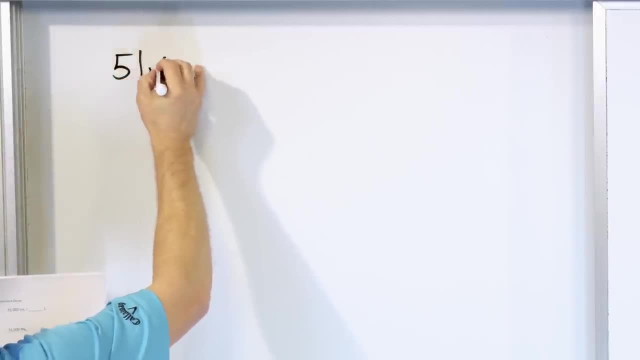 Only two more, Two more problems. Let's take a look at 51,000 milliliters. Let's convert that into the unit of liters. Well, the first thing is we write down what we are given. We're given 51,000 milliliters. 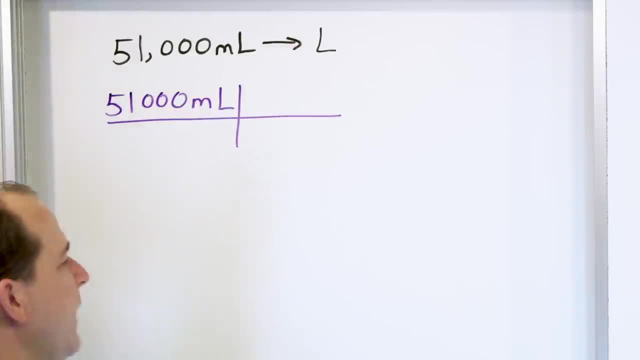 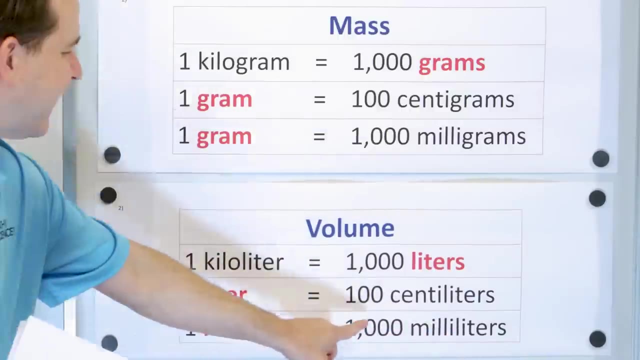 And we want to find a conversion factor that goes to liters. All right, We think there is one. So we go back and check our table And we see that we have milliliters and liters here. One liter is 1,000 of these little bitty milliliters. So we know that one liter is. 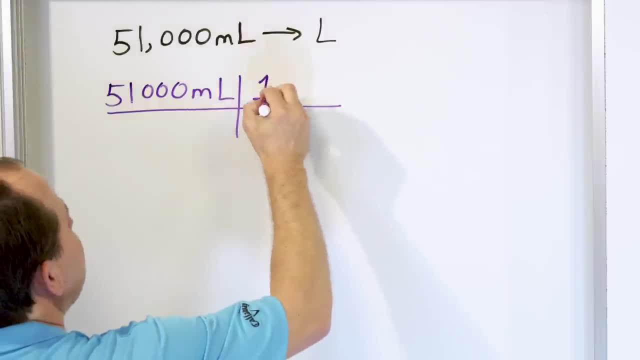 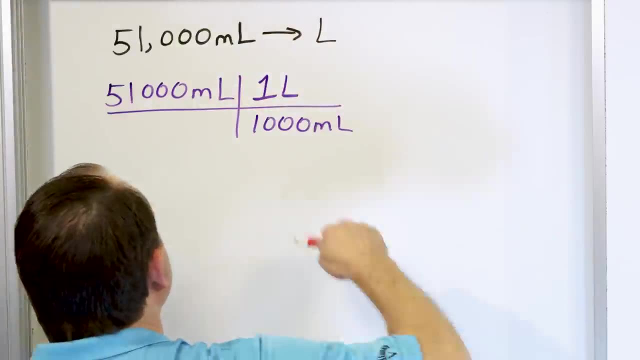 1,000. Milliliters. The only way we can write it is with one liter on the top and one thousand milliliters on the bottom, because if we flip it over, nothing will cancel. This is the only way the milliliters cancel, leaving us with liters. 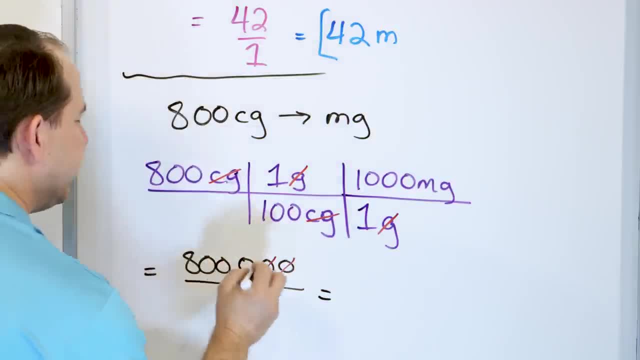 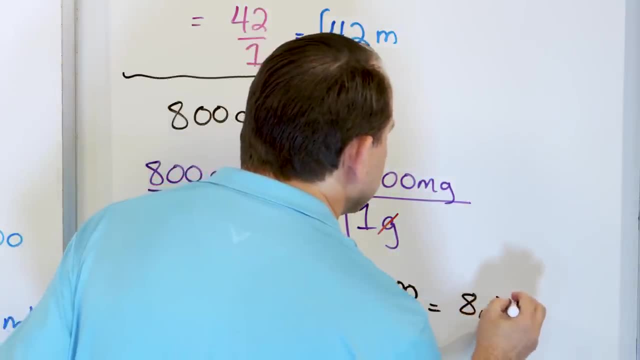 And so what's going to happen? on the top, I still have three zeros, so that's 8,000, divided by the one that's on the bottom, And so what you have is 8,000,. what are we talking about? 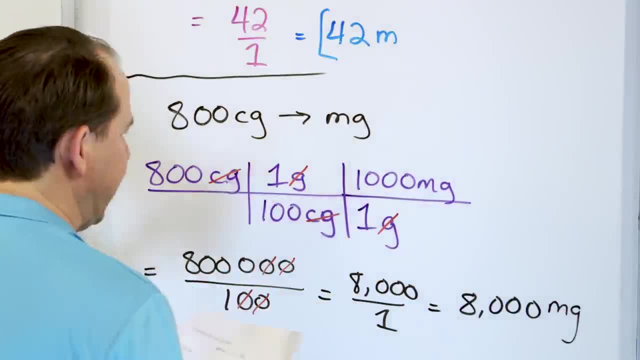 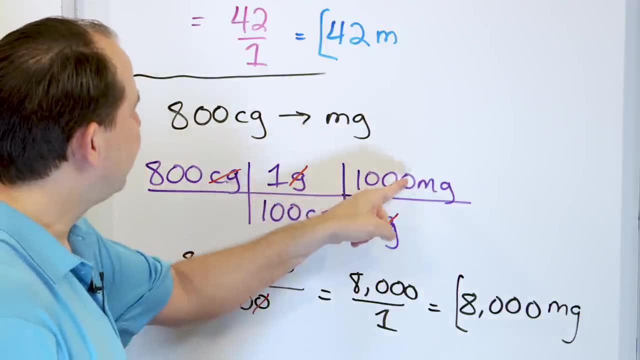 Milligrams. that's the only unit left. Let me check and make sure that's right: 8,000 milligrams. So you see why it's so nice to work with the metric system. Because multiplying when you have a bunch of zeros- 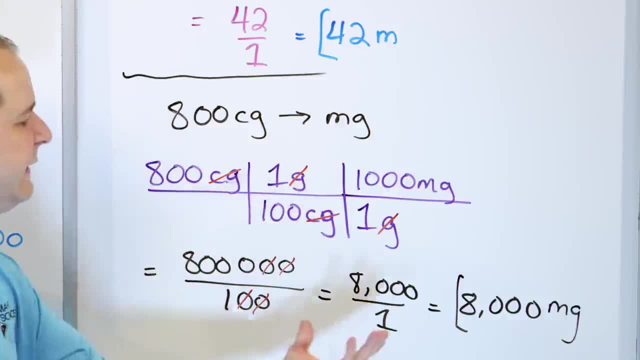 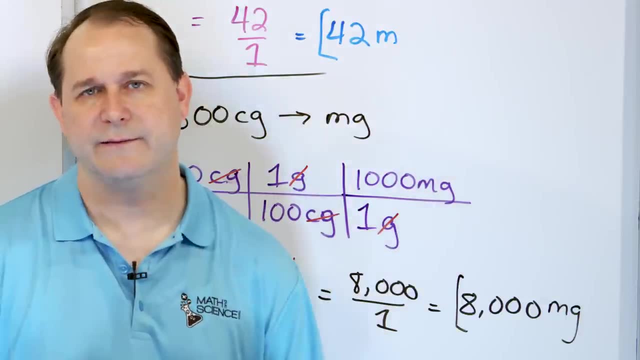 makes it easy to multiply and then dividing when you have a bunch of zeros makes it easy to divide And since everything is a power of 10, it just makes it very simple. We have a couple more problems. I wanna erase this and continue our lesson. 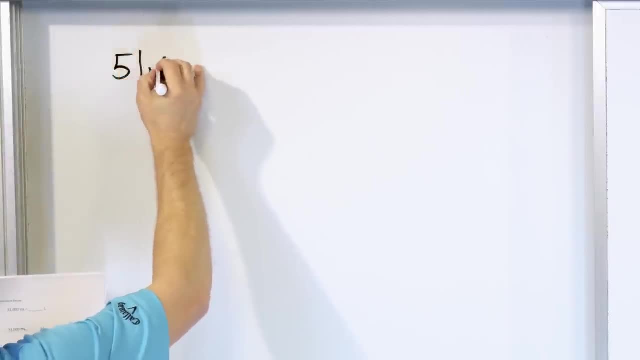 All right, only two more problems. Let's take a look at 51,000 milliliters. Let's convert that into the unit of liters. Well, the first thing is we write down what we are given. We're given 51,000 milliliters. 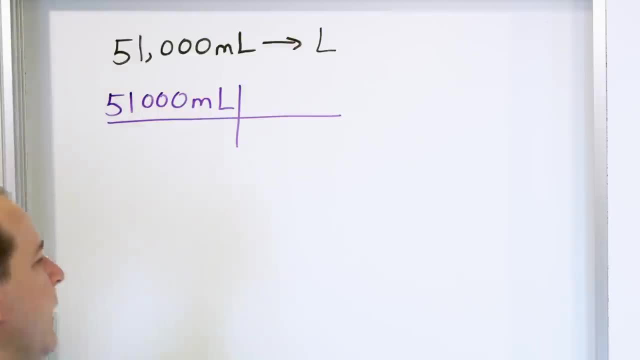 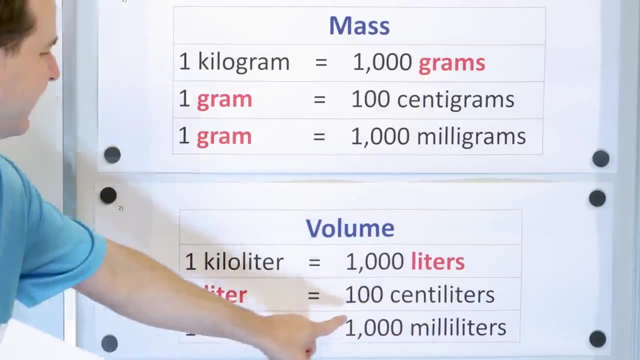 and we wanna find a conversion factor that goes to liters. All right, we think there is one. so we go back and check our table and we see that we have milliliters and liters here. One liter is 1,000 of these little bitty milliliters. 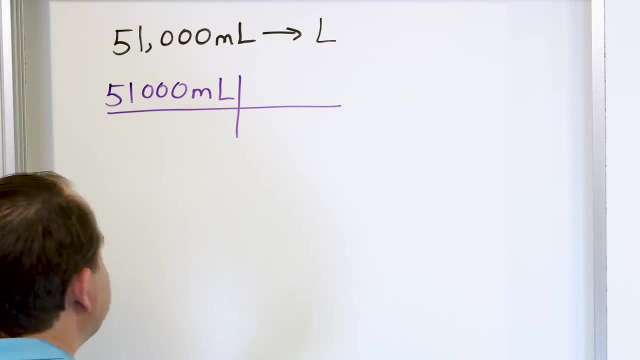 So we know that one liter is 1,000 milliliters. The only way we can write it is with one liter. one liter on the top and 1,000 milliliters on the bottom, because if we flip it over, nothing will cancel. 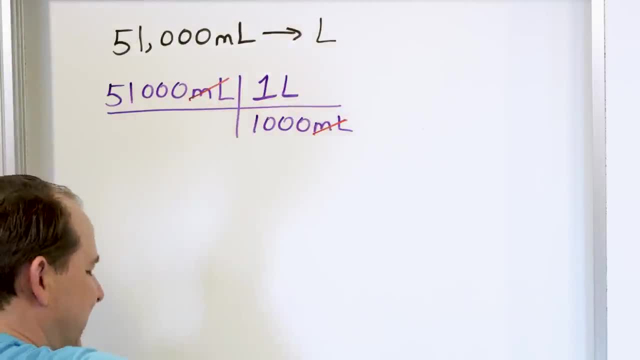 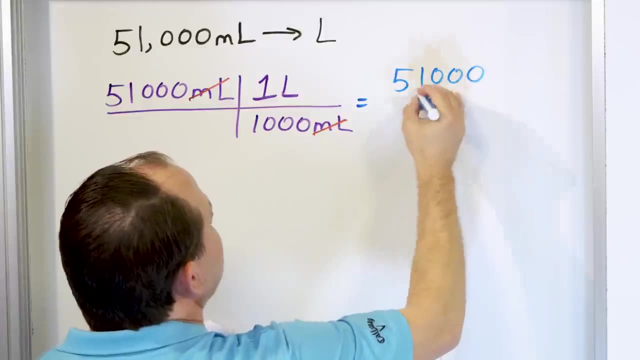 This is the only way the milliliters cancel, leaving us with liters. So all I really have to do is take the 51,000 times the one, which is just gonna be 51,000, and on the bottom I just have 1,000. 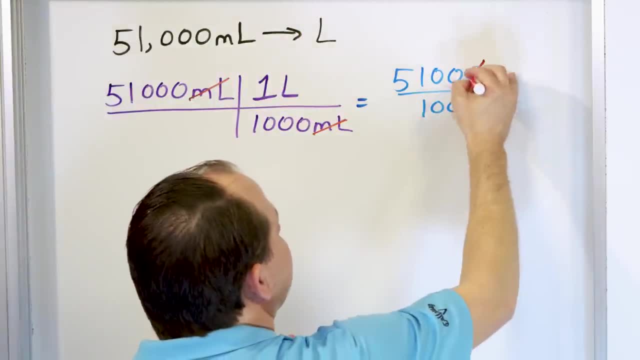 And now I have to do this division. But I have a lot of trailing zeros. This cancels, and this cancels, and this cancels, and all I really have on the top is 51, and on the bottom I just have a one, and then I have one. 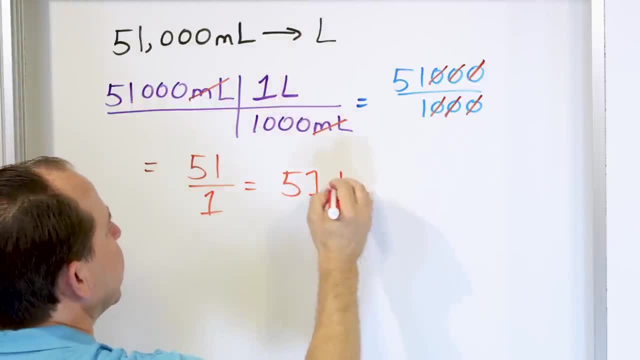 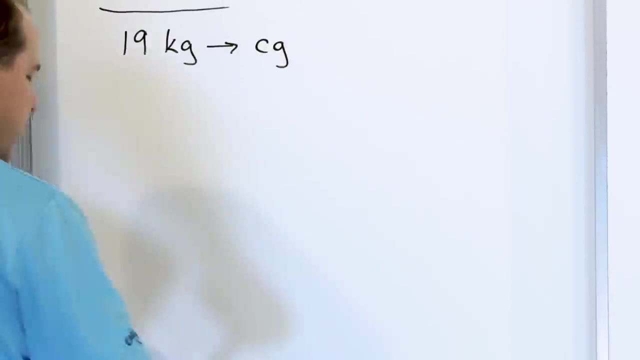 and so that's divided by one, so it's 51, what liters? and the answer is 51 liters, and that's the final answer. here's our last problem for this lesson. we have 19 kilograms. let's convert it to centigrams. kilograms to centigrams: we do not have a. 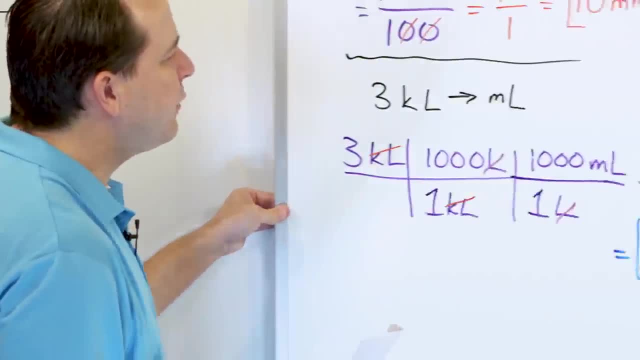 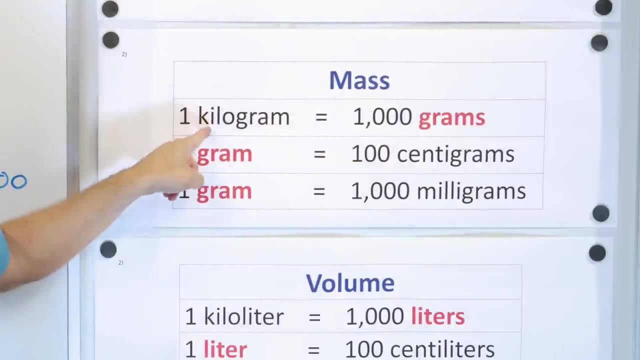 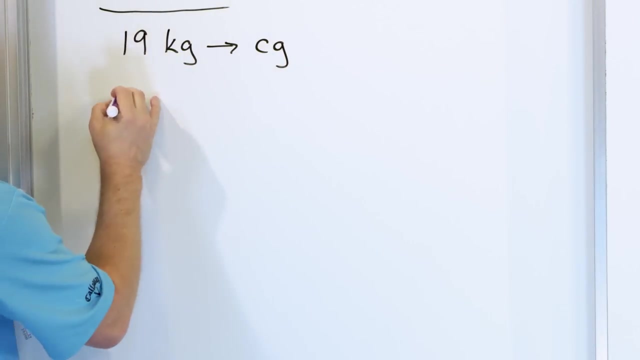 direct path from kilograms to centigrams, but we do have a path from kilograms to grams and then, once we get to grams, we go from grams to centigrams. so let's start by saying one kilogram is a thousand of these little bitty grams. let's write down what we are given. 19 kilograms extend our table and we want to write down now. 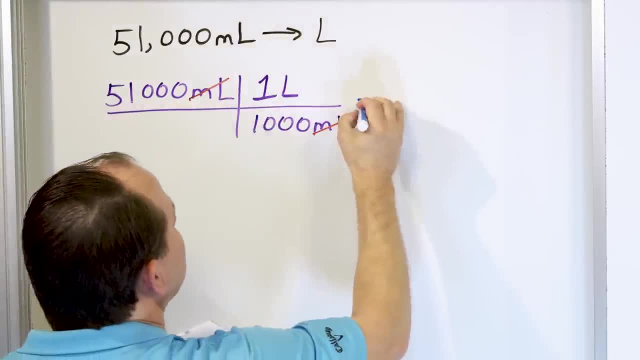 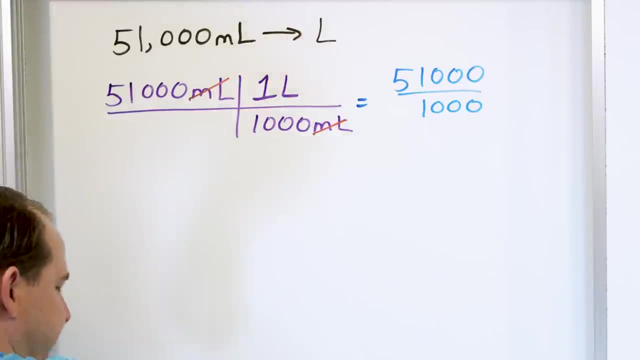 So all I really have to do is take the 51,000 times the one, which is just going to be 51,000, and on the bottom I just have 1,000. And now I have to do this division, But I have a lot of trailing zeros. This cancels, and this cancels, and this cancels, and all I really 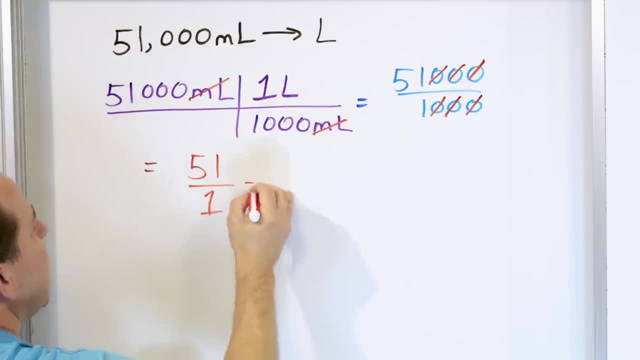 have on the top is 51. And on the bottom I just have a 1., And so that's divided by 1. So it's 51, what Liters? And the answer is 51 liters. And that's the final answer. 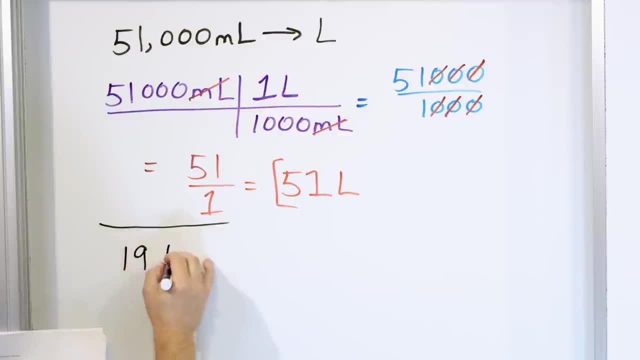 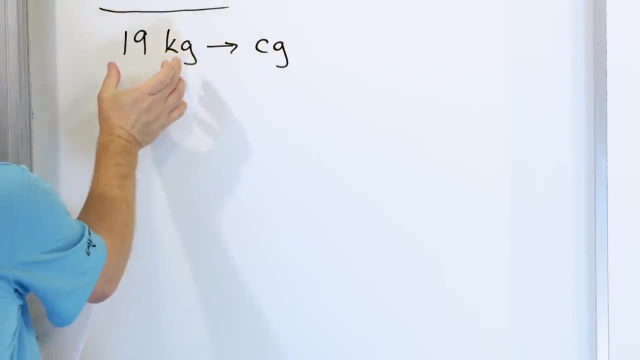 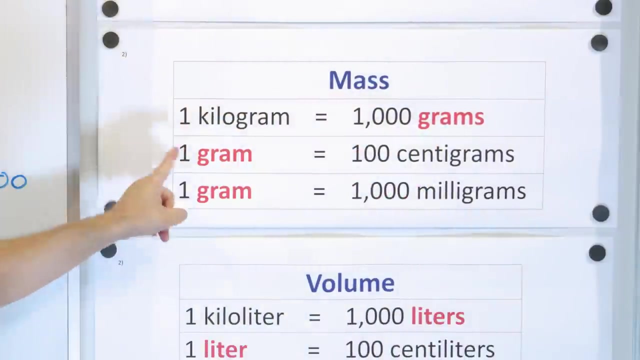 Here's our last problem for this lesson. We have 19 kilograms. Let's convert it to centigrams: Kilograms to centigrams. We do not have a direct path from kilograms to centigrams, But we do have a path from kilograms to grams And then, once we get to grams, 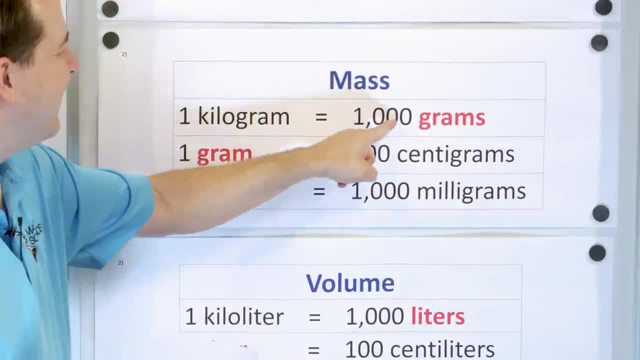 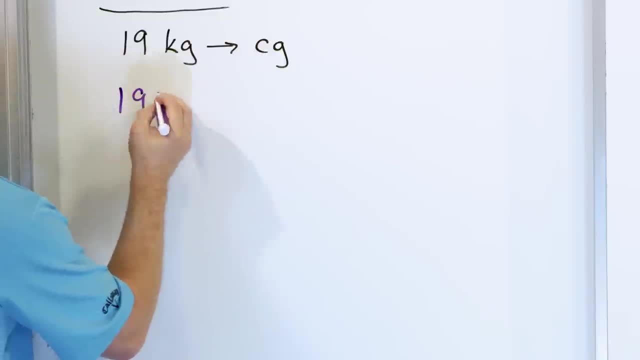 we go from grams to centigrams. So let's start by saying 1 kilogram is 1,000 of these little bitty grams. Let's write down what we are given: 19 kilograms Extend our table And we want to. 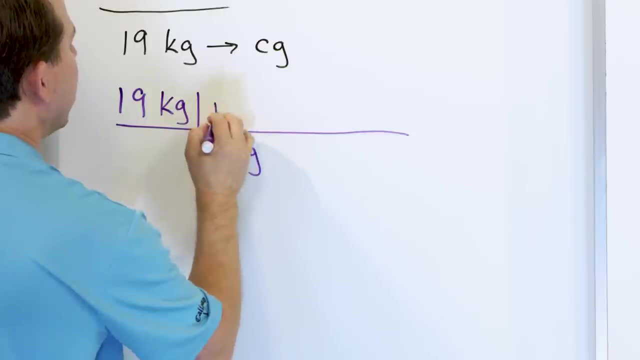 write down now that 1 kilogram is 1,000 of these little bitty grams. We have to write it that way because it's the only way the kilograms cancel. Now, going from grams to centigrams, Let's remind us what that is. 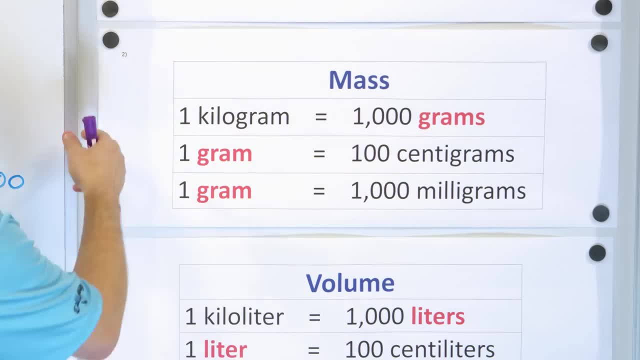 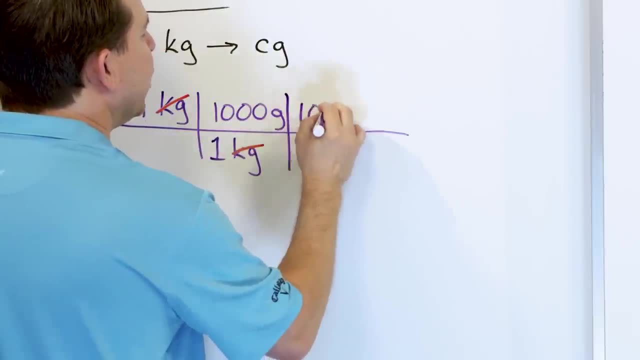 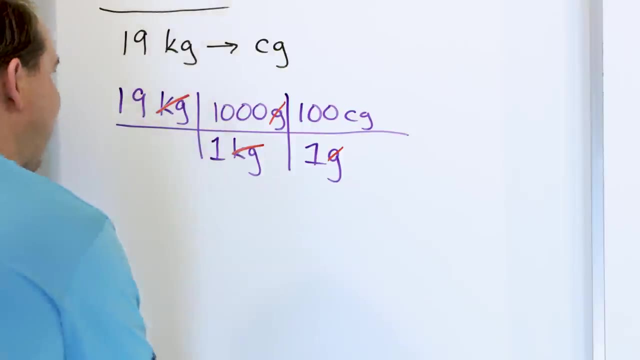 1 gram is 100 of these little bitty centigrams, Right? So we go and say: well, 1 gram is 100 centigrams. This is the only way I can write it, because I have to have a gram on the top and a gram on the bottom. to cancel. Now I am left with. 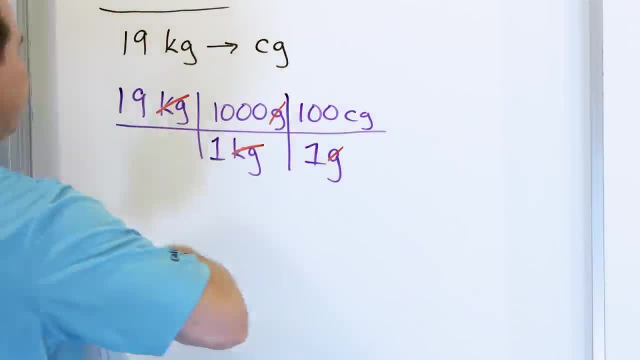 the unit I want to calculate. So how do I finish the calculation? I have to multiply the top and then I divide by the top, And then I have to multiply the top and then I divide by the top, And then I have to multiply the top and then I divide by the bottom. But 1 times 1 is 1.. So 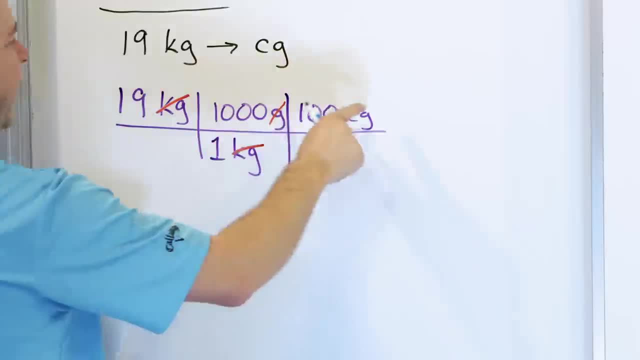 dividing by 1 is going to do nothing, So really I just have to multiply the top. So here I have 19 times 1,000.. What is that? Well, you just cover up the zeros. 19 times 1 is 19.. And then I just 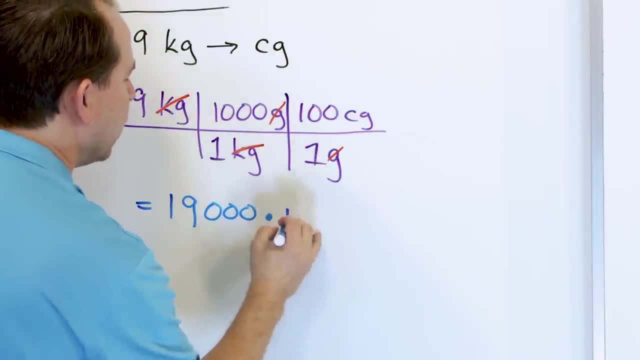 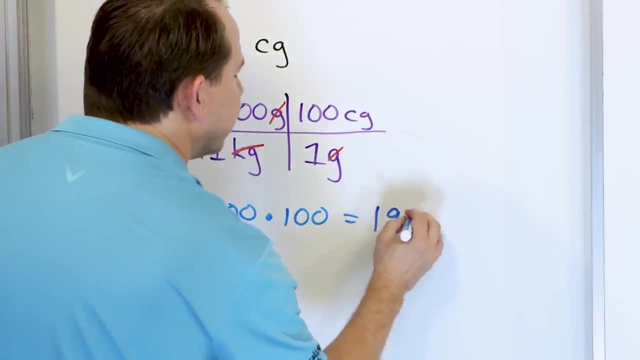 add the three zeros And then I still have to multiply by this 100.. What is this times 100?? I just cover up the zeros, multiply by 1. It's going to be 19,000.. And I covered it up here and 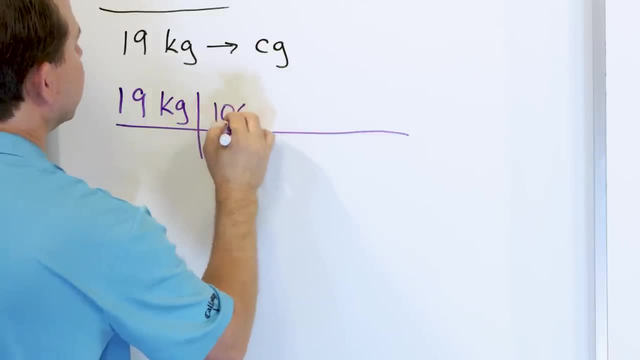 that one kilogram is 1 000 of these little bitty grams. we have to write it that way because it's the only way the kilograms cancel. now, going from grams to centigrams, let's remind us what that is: one gram is 100 kilograms. 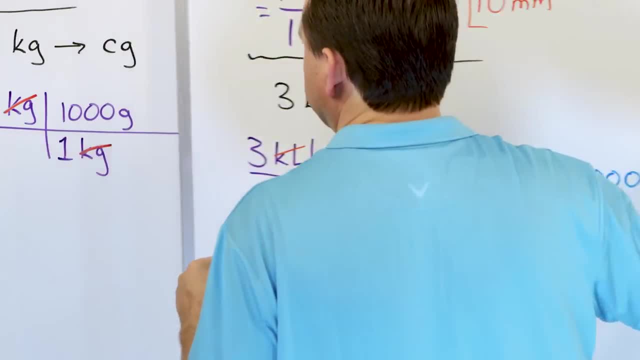 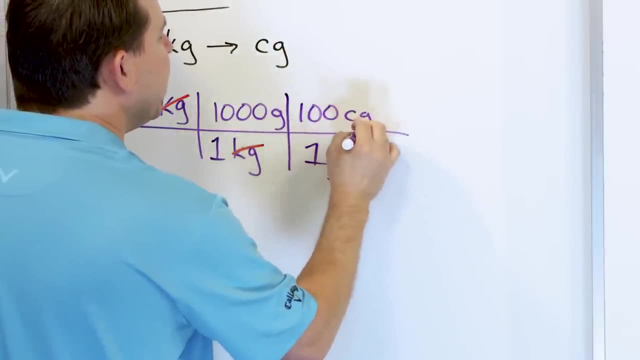 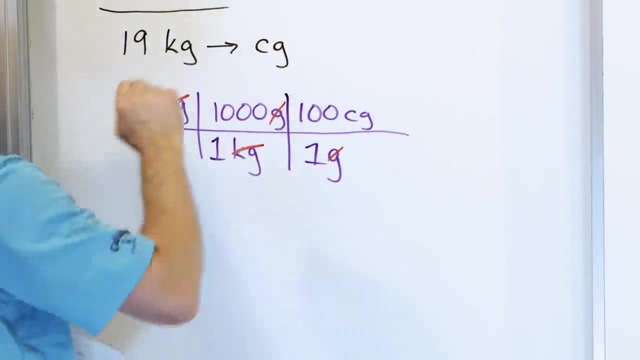 of these little bitty centigrams, right? So we go and say, well, one gram is 100 centigrams. This is the only way I can write it, because I have to have a gram on the top and a gram on the bottom to cancel. Now I am left with the unit I want to calculate. So how do I finish the 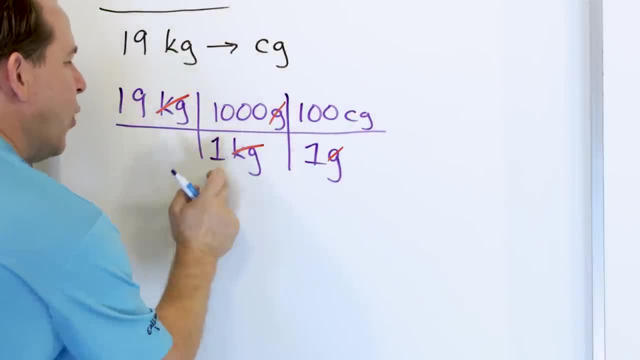 calculation. I have to multiply the top and then I divide by the bottom. but one times one is one, So dividing by one is going to do nothing. So really I just have to multiply the top. So here I have 19 times a thousand. What is that? Well, you just cover up the zeros 19 times one. 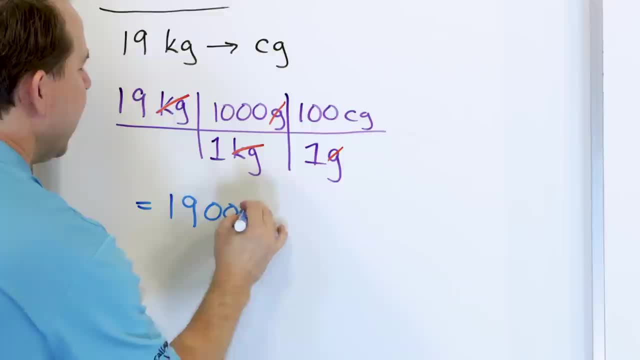 is 19.. And then I just add the three zeros And then I still have to multiply by this 100.. What is this times a hundred? I just cover up the zeros, multiply by one, It's going to be 19,000. 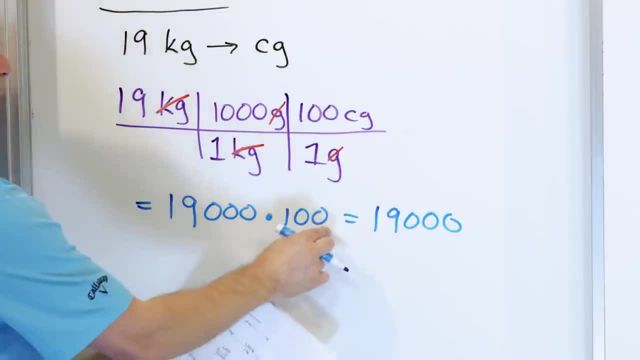 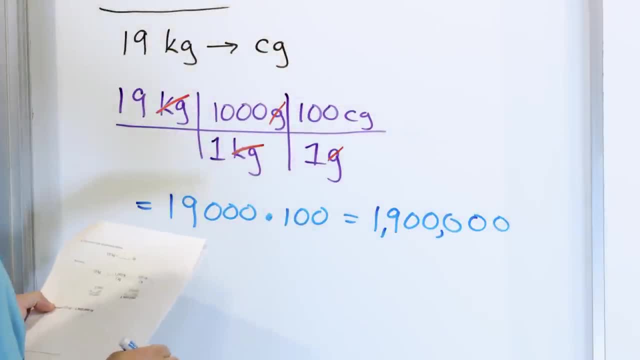 here's a comma, and then here's a comma: 1,900,000.. And the unit I'm talking about is Sinta Rams. So you see, multiplying by powers of 10, I just multiply by one, add the three zeros And then 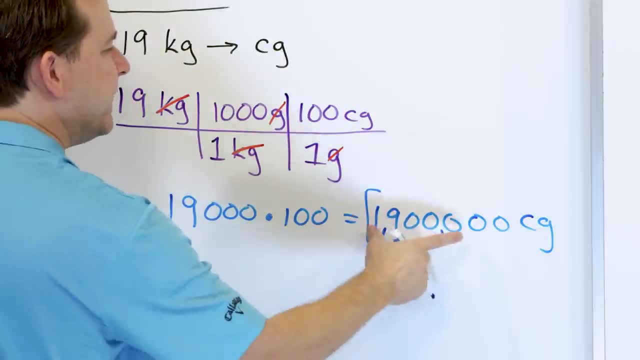 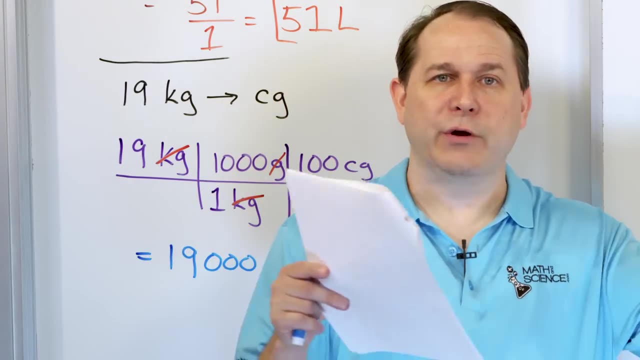 I multiply by this one, I multiply by one and then add the two zeros at the end. So basically, when you multiply by 10 or 100 or 1,000, you just essentially write down what you start with and you add zeros at the end. It's very simple And that's why unit conversions in the metric system. 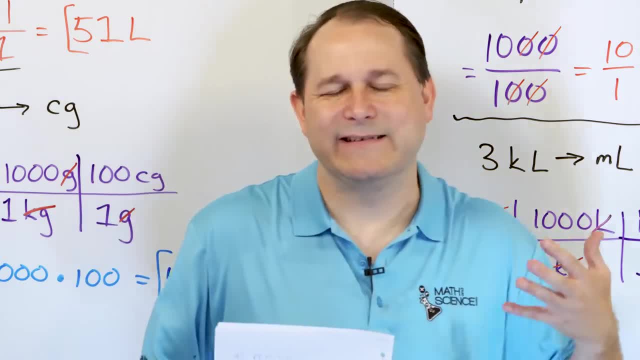 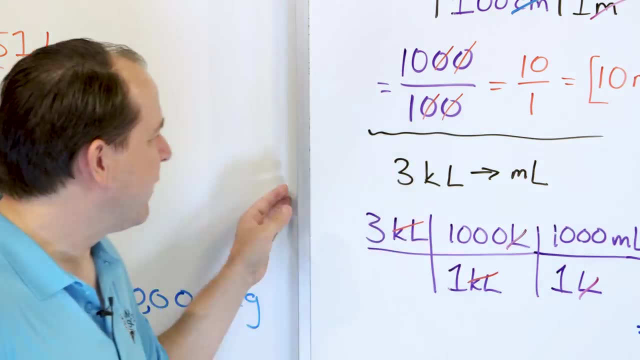 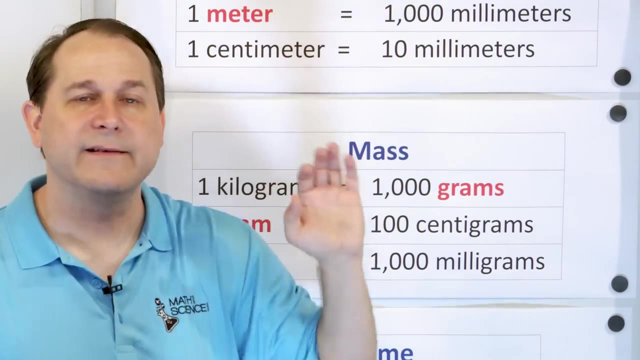 is so, so convenient. When we get into science and engineering and astronomy and things like that, we only use the metric system. because this table- remember in the beginning I told you this entire table- all it has is tens and hundreds and thousands and things like this, And it makes it.